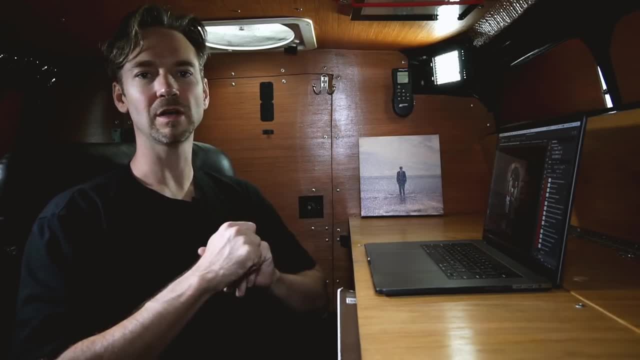 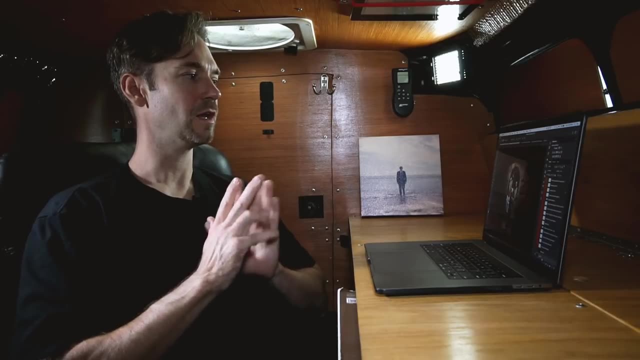 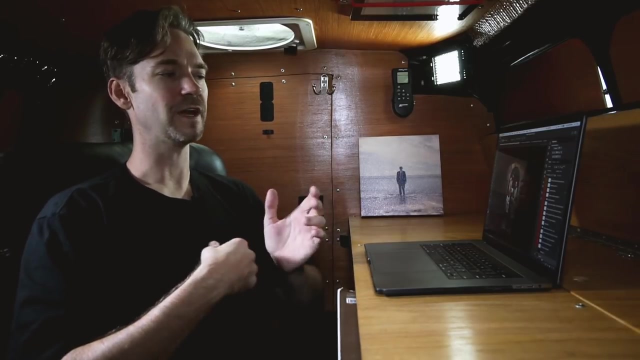 or all those things are going to be covered today. Let's go into the computer and we've got a couple submissions, but I'm going to be focusing on two photos from Tomer Jacobson and Maxim Golovanov. They submitted first and I wanted to do a very detailed critique for their work because they're fine art photographers and 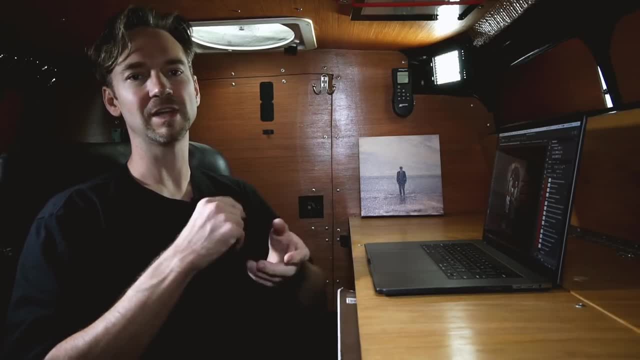 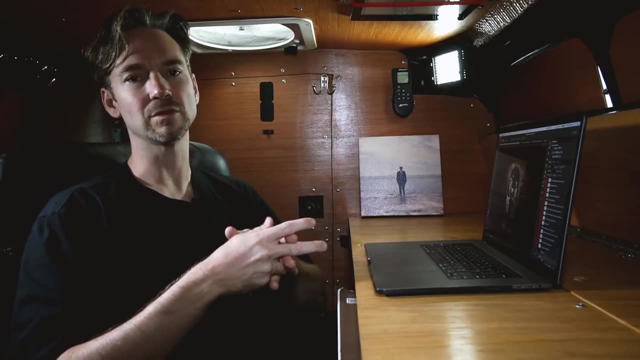 since they're fine art photographers, they have a little bit more time to plan things out, set things up, work with the grids, different grid systems a little more, as opposed to street photography, Which have minimal time to capture what they want. 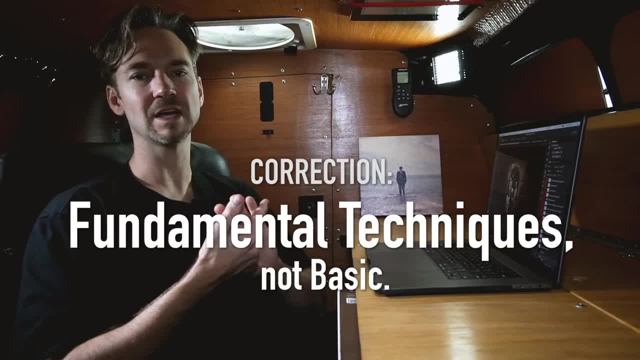 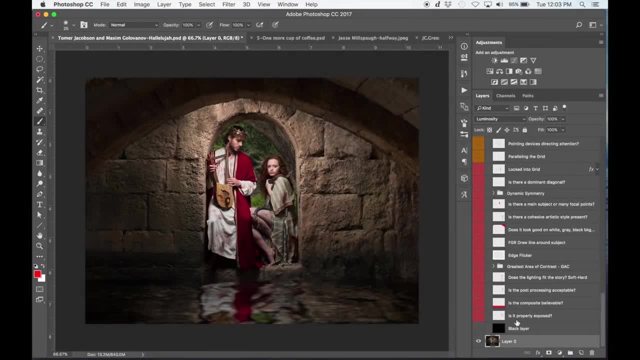 And they have to focus on some very basic design techniques instead of some more complex ones. So let's get into it. Let's go into the screen here. So this first one. they submitted quite a few photos, but since these take so long to do and to look at all the details and to present it in an unbiased way, 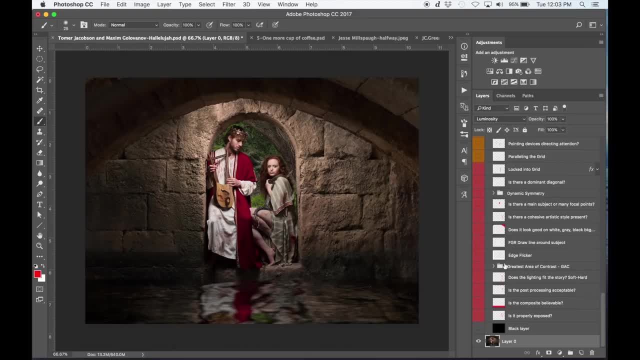 I was only able to do two of these, but they did have quite a few more good photos and I'll put their link to them in the description And a link to their website up so you guys can check it out. First off, we're just gonna check the. 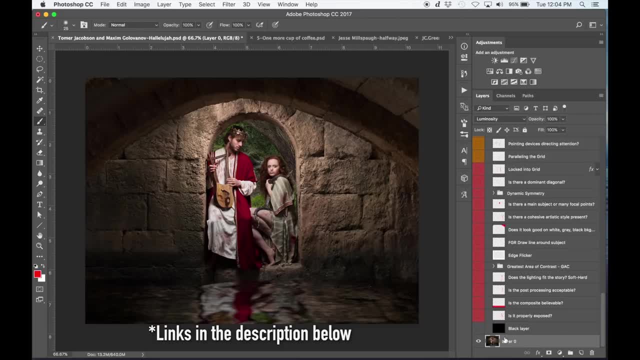 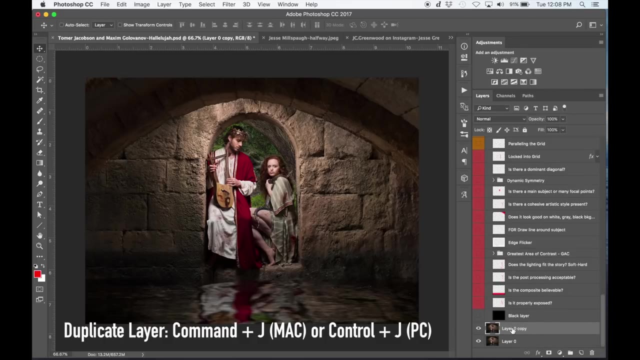 exposure and see if the exposure is good for the photo. And I noticed, at least on my computer, it's a little bit darker than normal, which is easy to fix. Usually a good way to test this is to push Command J. That's going to duplicate the layer. You can push Ctrl J if you like on a PC. 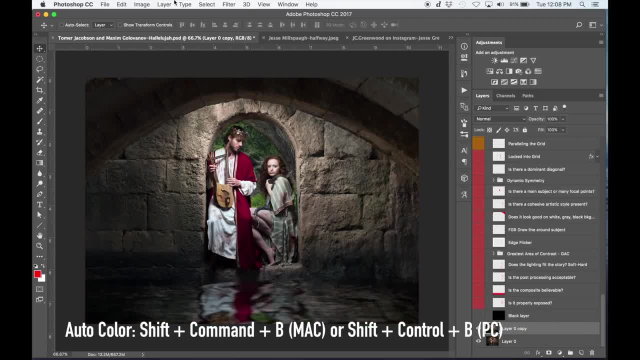 Then Shift Command B, do Auto Color- and that's up here also- And image auto color and that adjusts the color as well as the exposure. but my friend Joseph gave me a tip that if you put it to luminosity it's just gonna show the exposure correction and not the color correction, which is kind of cool. 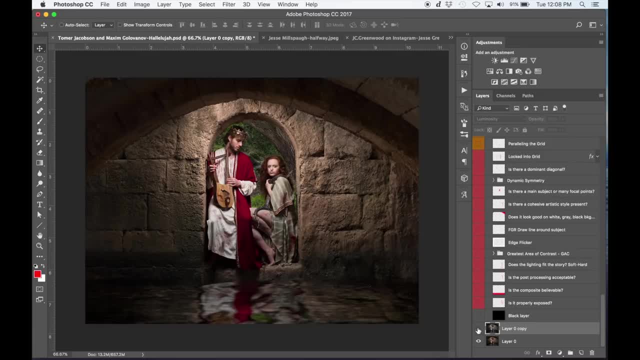 so do that and now we can compare the before and after. that was before. so now, after we have a little bit bump in the exposure and it's a little bit brighter and things are properly exposed there. so that's our starting point and I'm gonna put a black layer on here so we can see the correction or the adjustment layers. 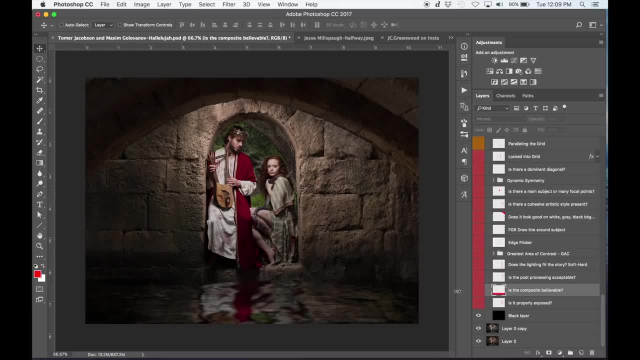 pretty easy. now we'll ask the question: is the composite believable? so a lot of things that can maybe discount a great photo is unbelievable composites. so right here, this water reflection isn't very realistic. it's a good job, but I can still tell it's a composite like nothing else up here. I mean, even if this, this 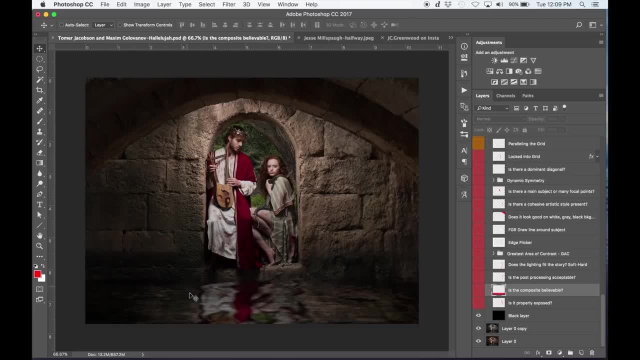 little instrument is a composite, I can still tell it's a composite, like nothing else up here. I mean, even if this, this little instrument, is a composite, I can't tell, but this I can definitely tell is a composite. so I would either look up some tutorials on how to create believable reflections or 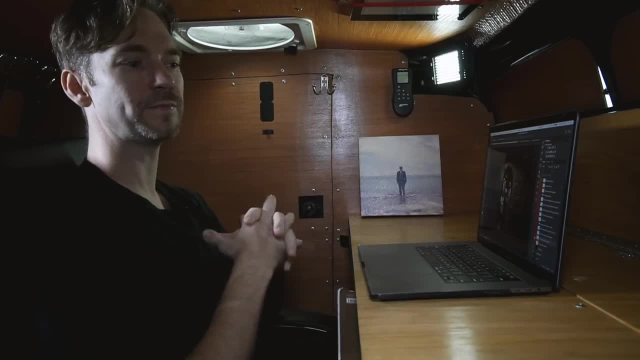 I would just take that out completely. and I know on his website he's got all of these images are inspired by certain songs. but to see it in an unbiased way, we have to look at our art as everyone else that doesn't have the same emotions, doesn't have the same emotions, the same experience that people have. that can't. 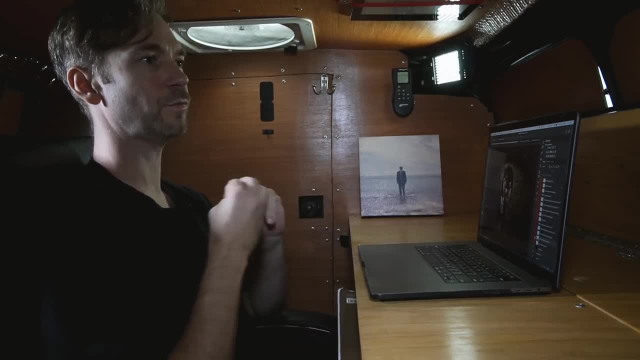 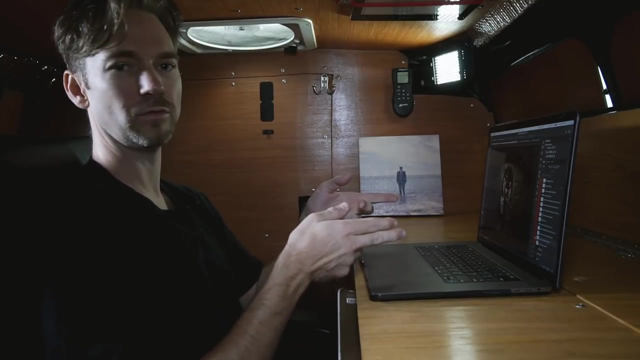 experiences isn't listening to the same song. We have to put our work out there in a way that's communicated clearly and let people create their own stories. So maybe if I was listening to the song while I was viewing this, then I would start to understand maybe why the water was there and 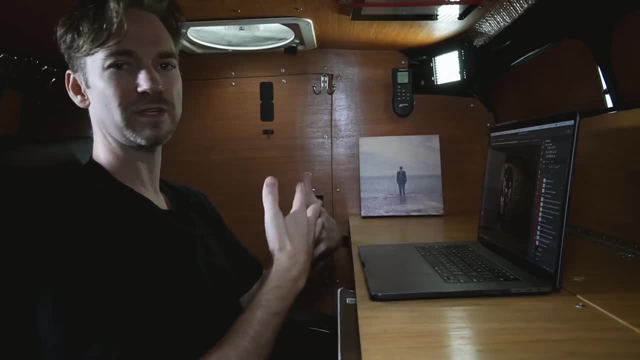 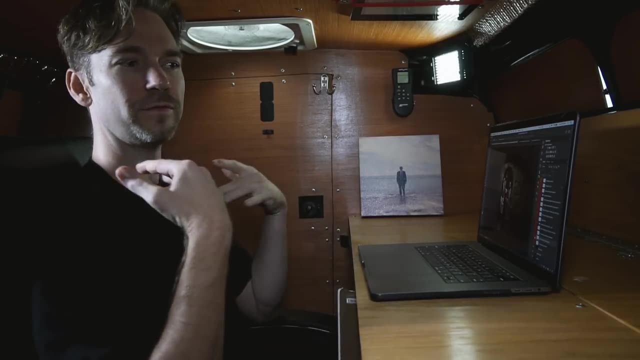 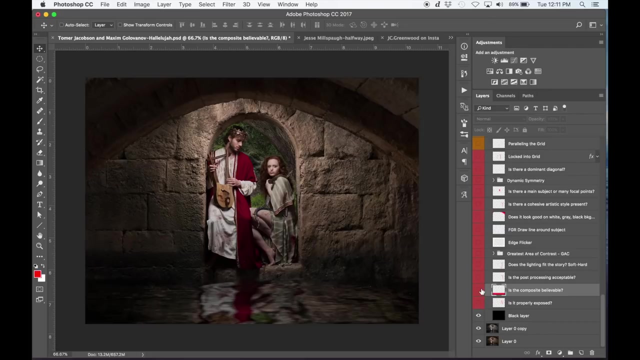 things like that, But I have to judge it on the way it's presented to people, without further explanations like captions or music or anything like that, And that's how photographers should present their work. It's cool to create a concept like this that goes with music, but if people 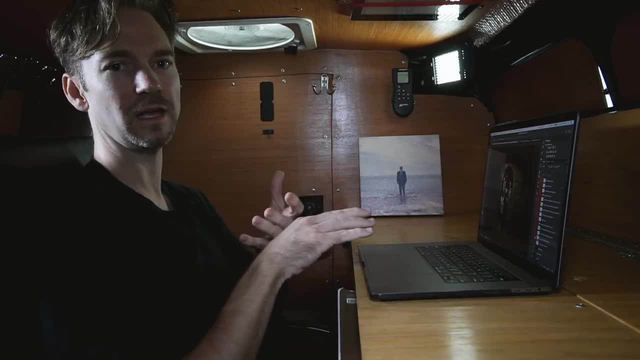 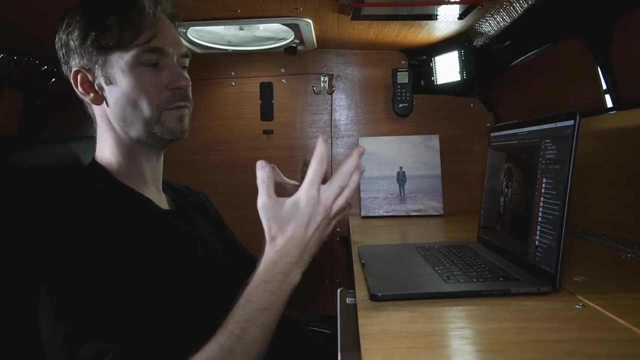 aren't viewing your photo with the music, which is probably, I would say, 50 to 90 percent of the time, because that image is floating around Facebook and things like that. you need to communicate it in a clear way. that can work very well without music or additional captions. 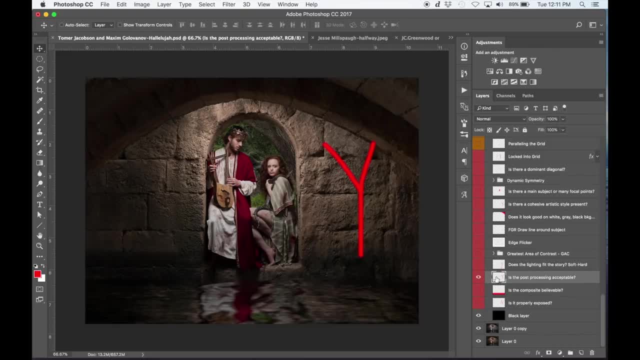 So I would check out the reflection. Is the post-processing acceptable? Yes, I think it's acceptable. Looks good to me. Does the lighting fit the story? So you've got soft lighting, which is good. You could probably manipulate the way you're telling your story by, since you've got blood and 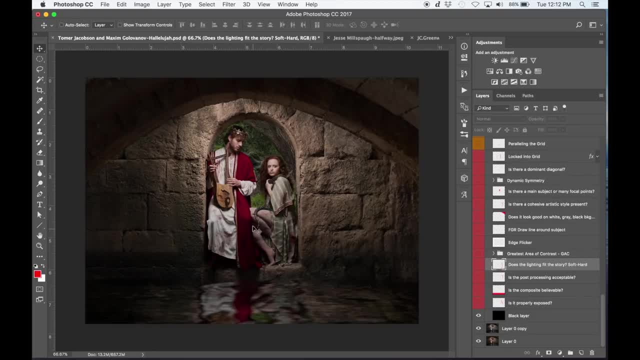 you've got kind of a dramatic story going with the snake and the blood and the dark, cavernous room. you might be able to manipulate it a little differently: the way it's communicated, by using harsher light. lighting that's not as soft as you have here. The soft light's quite flattering. 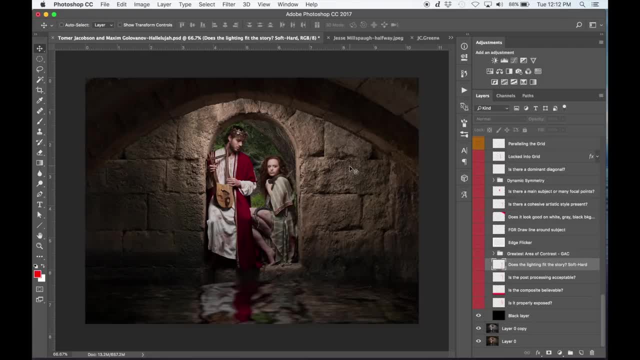 for the subjects, but if you're trying to communicate in a different way than what you're trying, you can make it even more harsh feeling and more dramatic. if you had more dramatic lighting, Imagine this scene with candles everywhere instead of the soft box above. That would create a 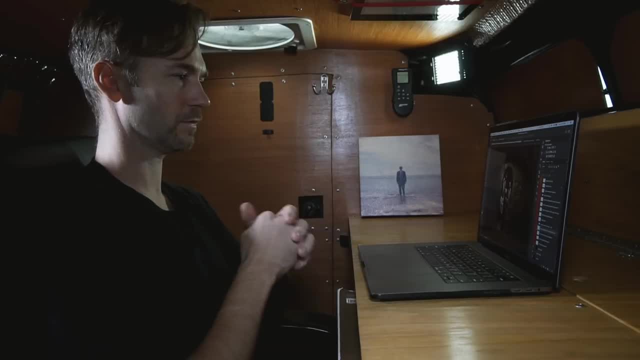 different scene, but that's only good if that's the story you're trying to tell. So we can't judge it on anything else except for the way it's presented And we can't be biased on the way we would do it. but I'm just throwing some ideas out there of how the story can change. 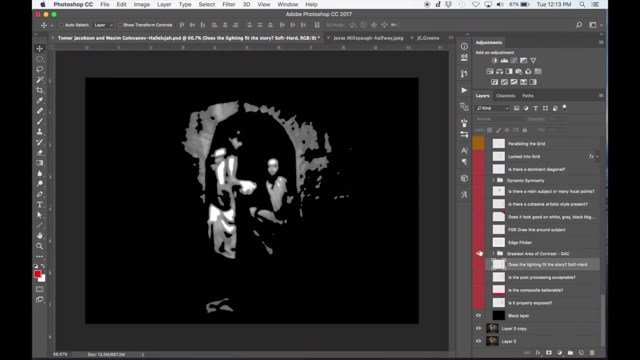 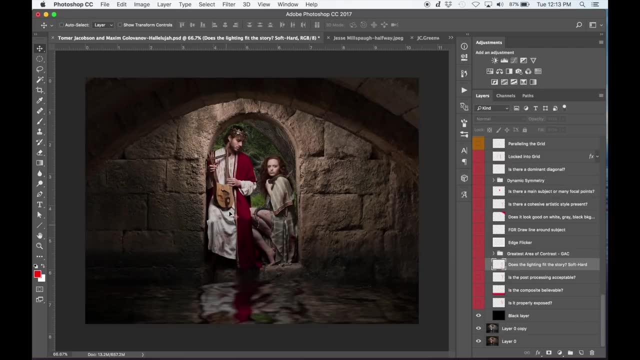 depending on the type of lighting you choose for your scene. So we've got the greatest area of contrast, which is good. It's in a good spot. The man has the most significant amount of contrast. He's got that big white robe with a dark. 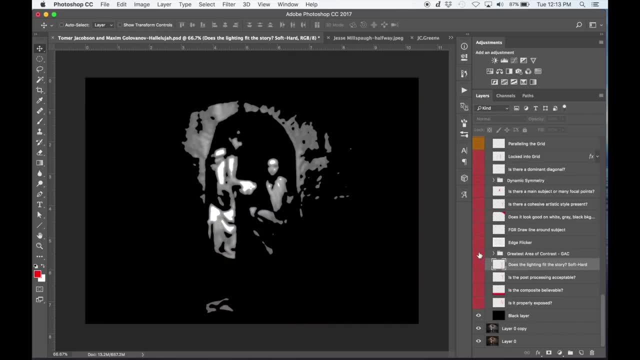 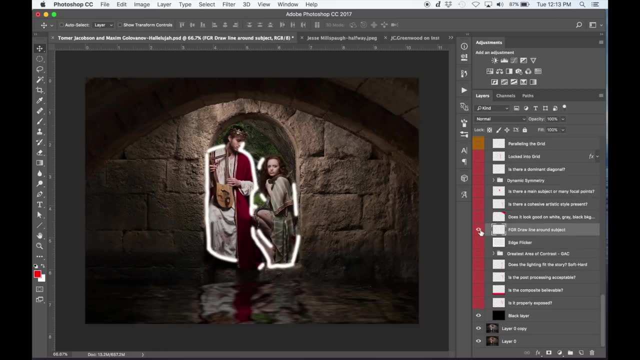 shawl on him So we can see. that's where the eyes go first, which is good. The edge flicker. we're looking for high contrast near the edge and that one looks good. There's no high contrast near the edge. Figure-ground relationship. we draw an. 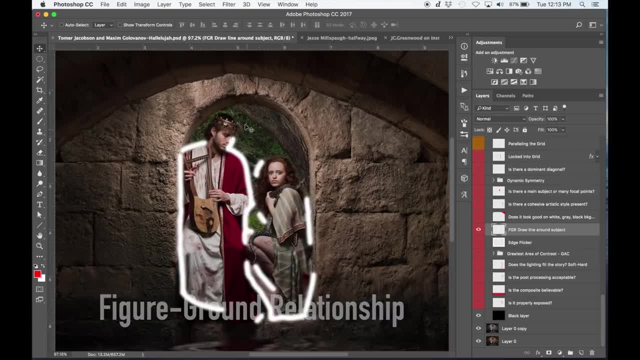 imaginary line around the subject and see where we lose contrast. So you've got pretty good contrast around them. The figure-ground relationship is a little bit weakened by his dark hair up against the dark background and it goes around and then around her hair in the dark background. okay, And then the 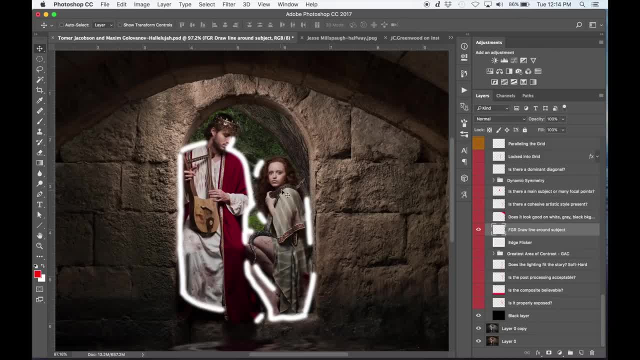 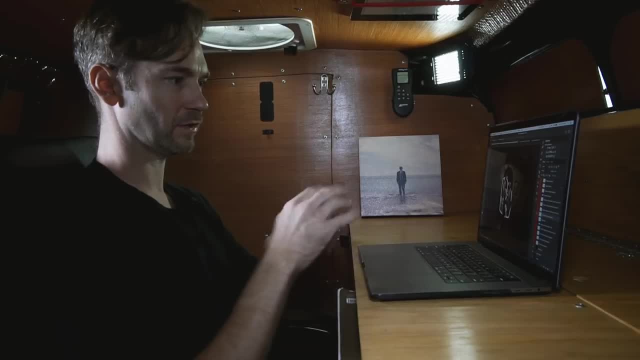 snake head is a little bit lower contrast, as well as his body near her shadow right here. So that could be adjusted as well. And to tell you the truth- I'm going to get into all this stuff- I actually didn't notice the snake at first, until I was analyzing it. 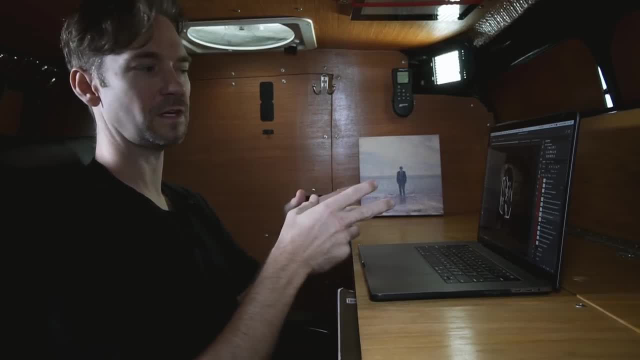 So we're going to take note of that. the way people perceive what they see, They're going to see the image as a whole instead of the individual parts. I'll explain that in the area where we cover negative space: Okay, so also I check for. 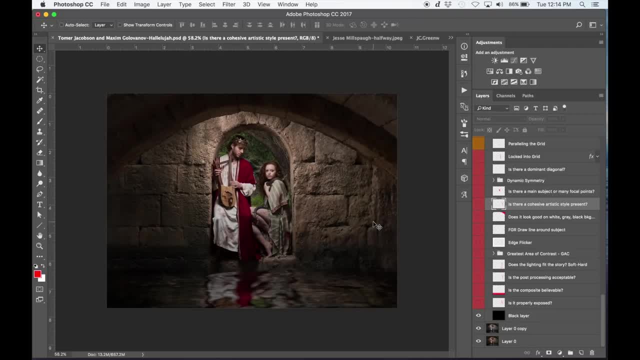 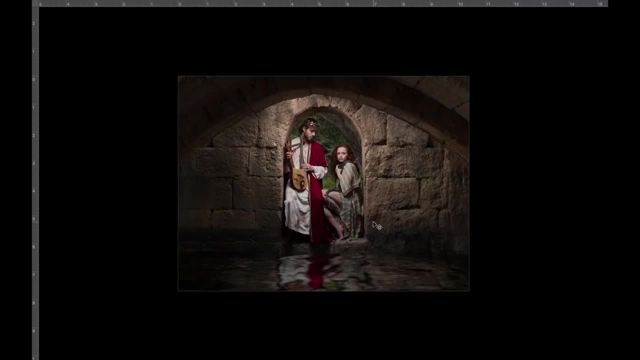 if it looks good on gray, black and white, And this is going to be showing you the areas that are high in contrast around the edges that perhaps you missed. So when we go straight black, we can see that the upper corner right here has quite a bit of contrast. 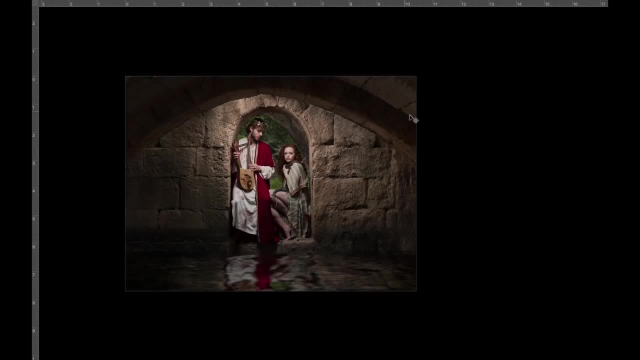 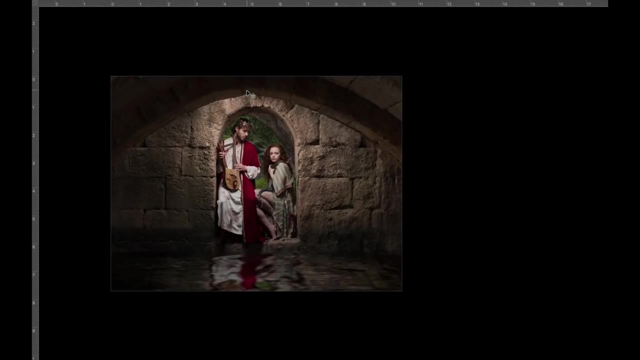 And then over here we see a little bit of contrast. It's still subdued enough to not draw too much attention, So we can leave that as is. Doing this with gray white and black gives you the chance to see it by using 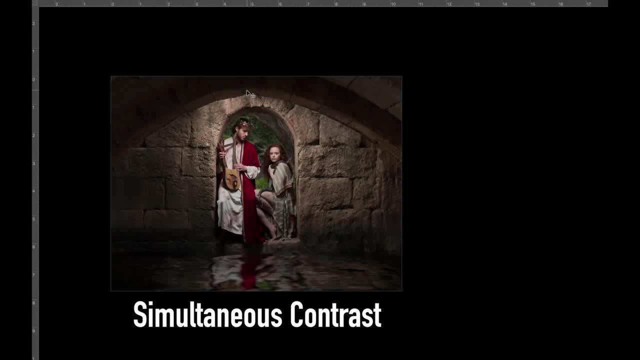 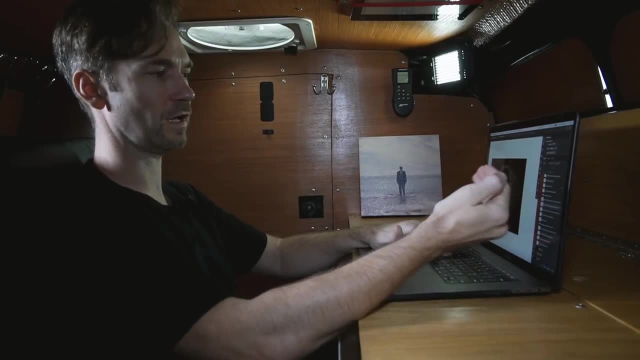 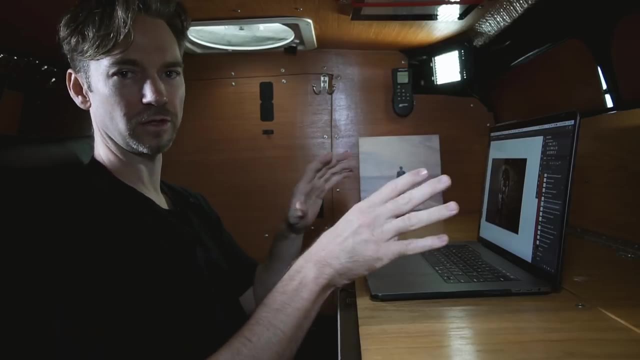 simultaneous contrast. So if the background is darker than your photo, then the photo is going to look lighter. But when you switch it to white, now your photo's darker and the background's lighter. So with simultaneous contrast you can start to see a little bit of different things, depending on the neighboring value. 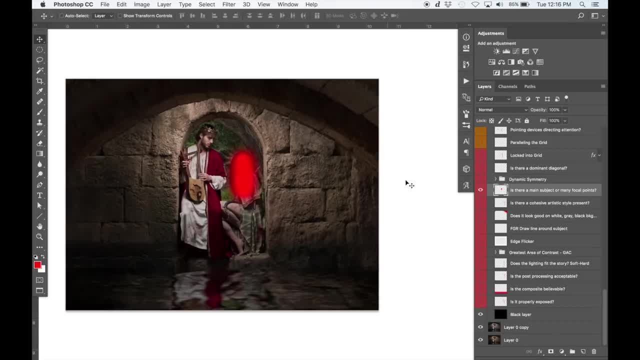 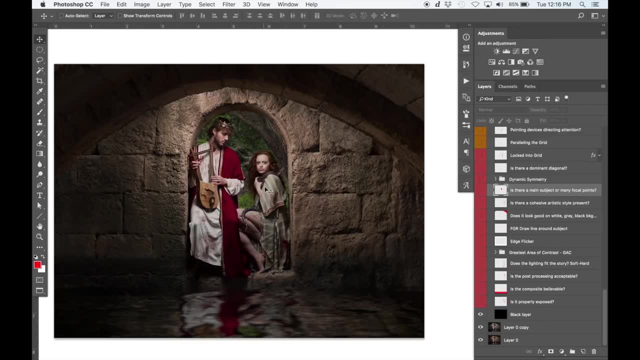 Is there a main focal point or subject, Or is there multiple ones drawing our attention? So I would say she's the main focal point because she's looking straight at us And her pose is very dynamic, And then he's looking at her, so that directs attention to her. 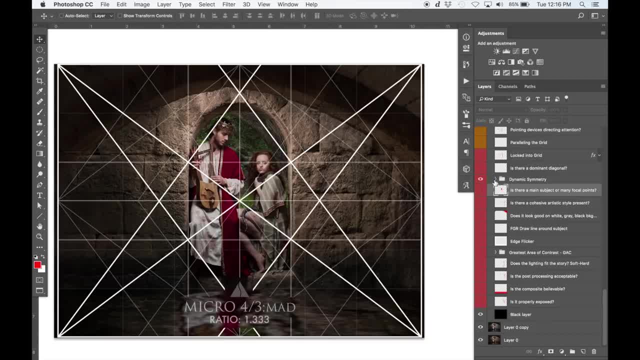 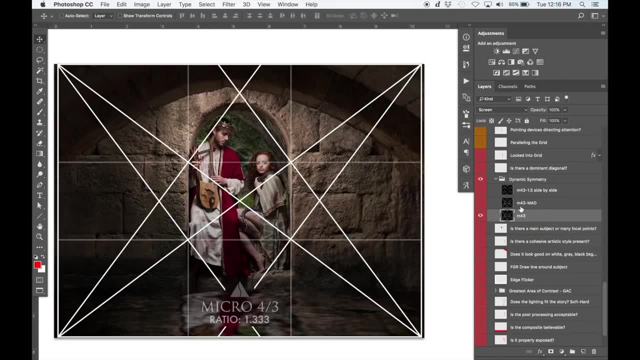 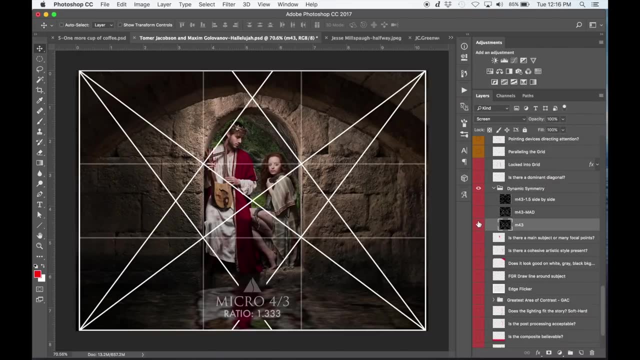 So that's what I'm seeing, is that she's the main focal point. Okay, dynamic symmetry: I don't believe that you use dynamic symmetry to compose these images, but we can still analyze it with the grid, And the grid that it's closest to is the micro four-thirds grid, which is just a four-thirds ratio of 1.333.. 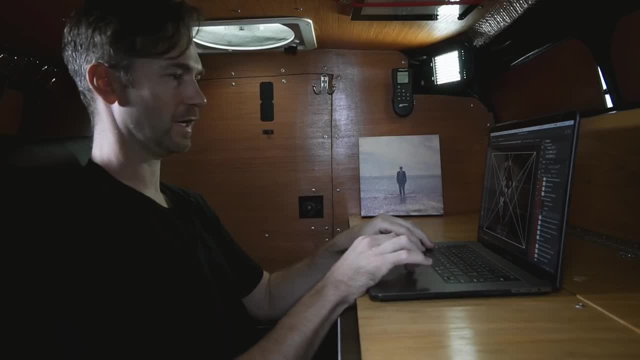 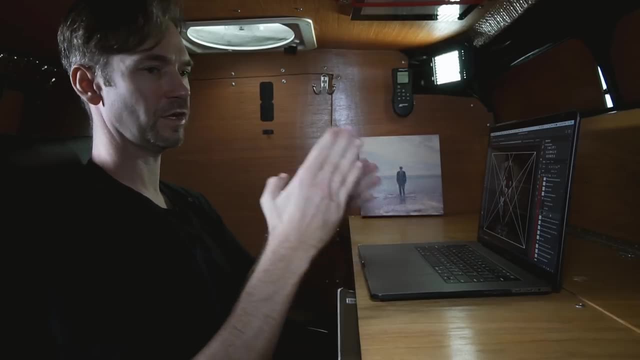 And if you wanted to get this exact, you could crop it down exact. But I don't recommend cropping huge chunks of your image off. I recommend composing in-camera with the grid and then you can snip the ends off or snip the top off. 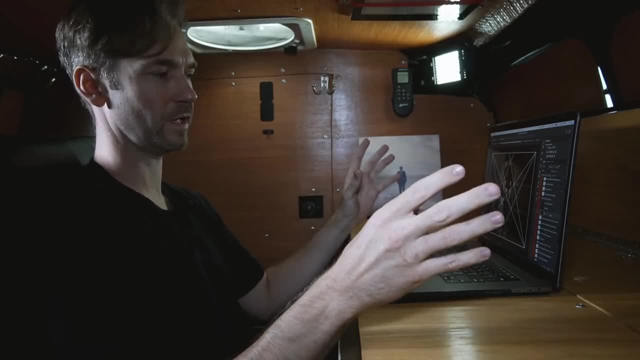 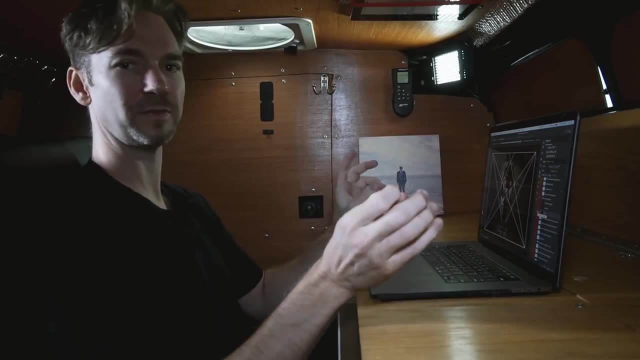 whatever you need, I recommend not just shooting what you want and then coming into Photoshop or Lightroom and just cropping the heck out of it. So do it on location and you'll save lots of pixels and you'll be in more control of your composition. 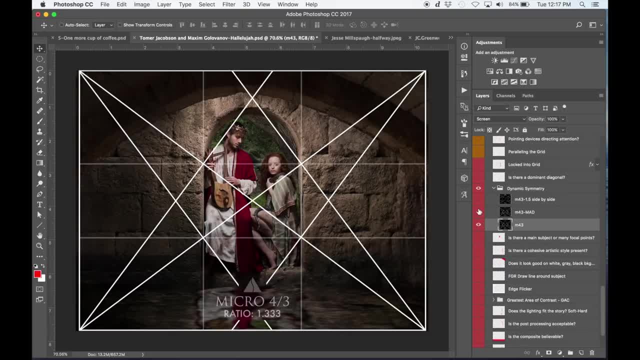 Interestingly enough, we've got some things lining up here. Let me see if there's a dominant diagonal, which there is, is her leg. It's not a huge diagonal, but it's still a diagonal. We see diagonals in his composition, which is good. 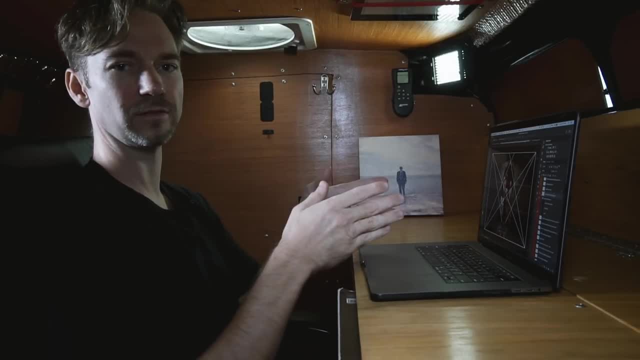 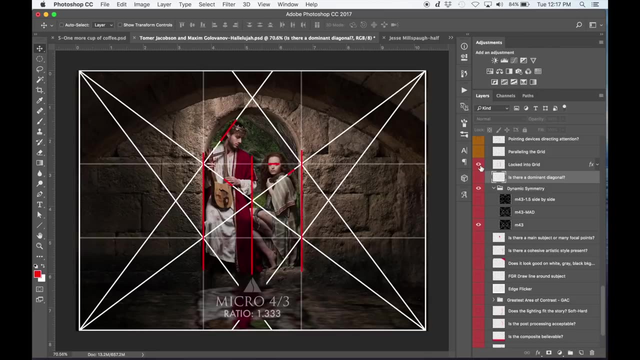 It makes it more dynamic. Instead of like a flat, everything's horizontal or everything's vertical, we have some dynamic movement in this which helps, and we'll see that. So let's see the things that are locked in. We've got quite a few things locking in. 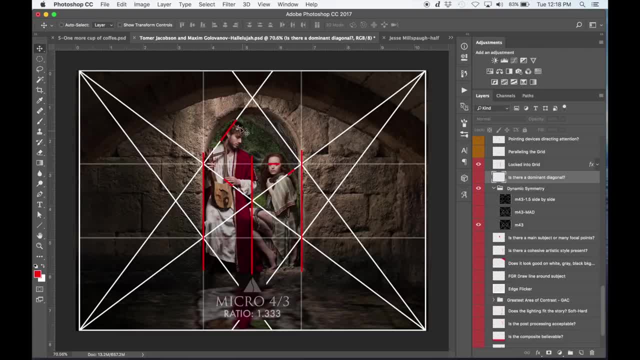 The doorway, her eyes, the snake head, the man's head, his hand, the center which is where his body is- Okay, but all of this negative space- we're going to talk about that soon. All of this grid is not filled up and the dominant diagonal is very small. 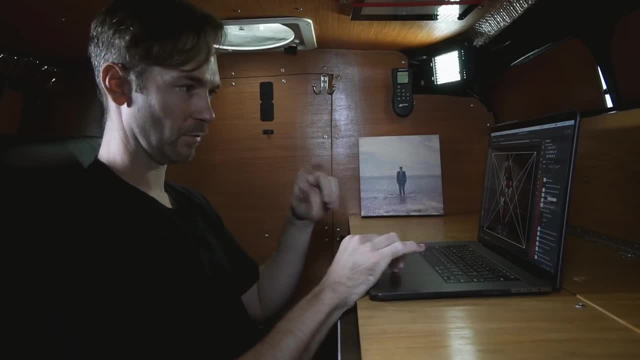 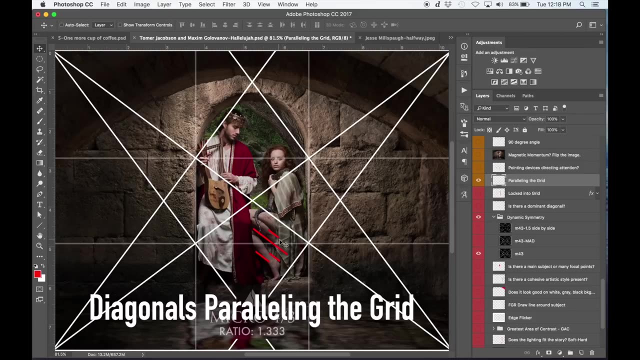 So we have less of an impact on our viewers And we're going to cover all that. Let's look at paralleling things that are paralleling to the grid And he did a nice job of just capturing diagonals And coincidentally, they parallel quite a bit with her legs here. 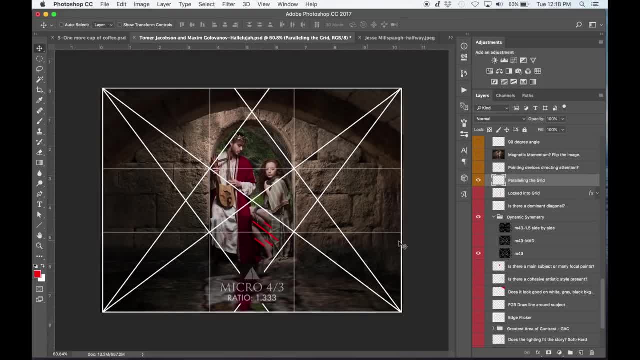 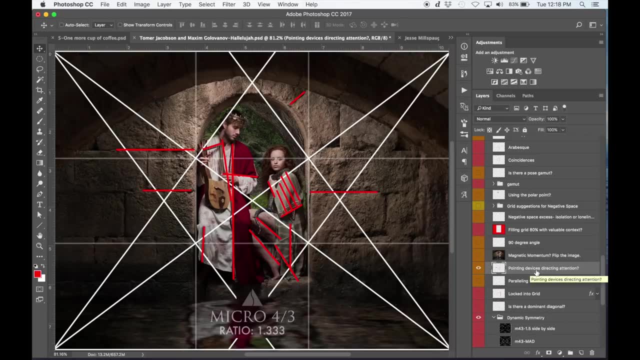 And they're paralleling the exact diagonal of the Micro Four Thirds grid. Do we have pointing devices? And pointing devices are like. I guess you consider them leading lines, but they're more advanced And they're not described. They're not describing generic roadways or pathways or bridges that lead to the subject. 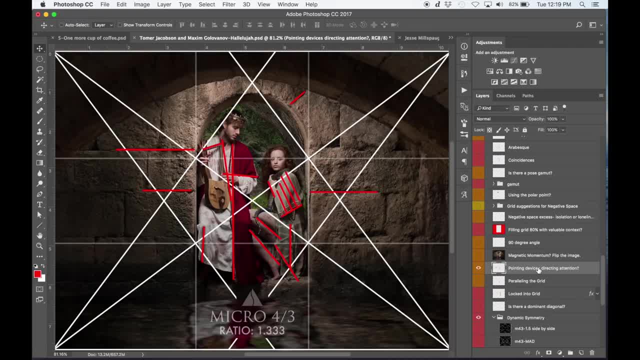 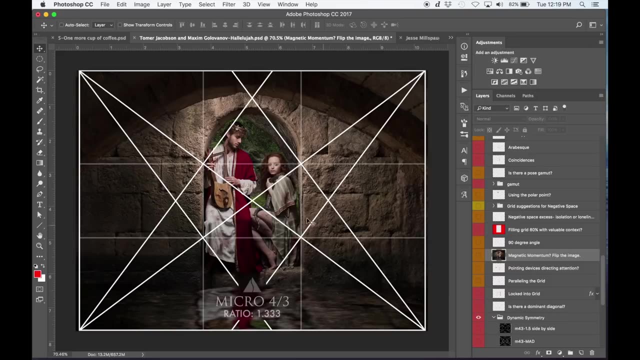 It's more advanced and it's hidden linear movements that direct attention towards the viewer. So right here we could see a lot of different linear movements that direct attention towards our subject here, which is good. Okay. so magnetic momentum is a thing that I've kind of put a term on, where your greatest area of contrast, 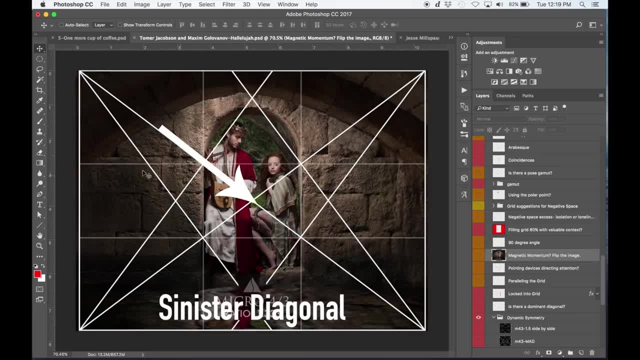 if it's in close proximity with the sinister diagonal, which is the diagonal that goes from top left to bottom right. That's the sinister diagonal. So if you have a high contrasting element in the upper left polar point or near the sinister diagonal, that's going to create more movement up and down because of the way we read. 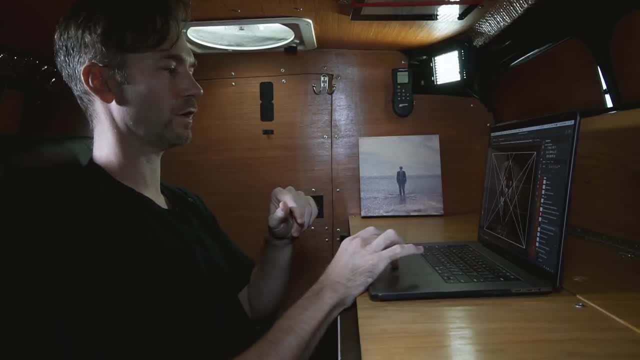 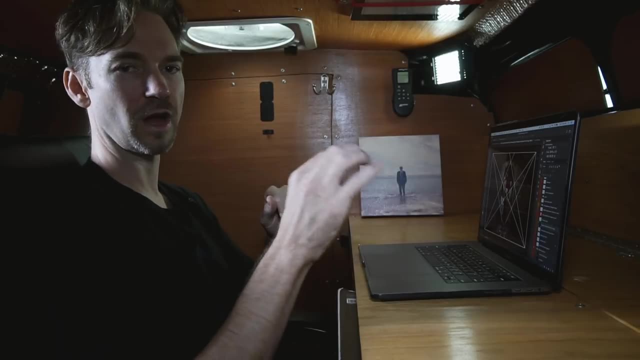 the way we read left to right and top to bottom. So each corner, each area of the grid kind of manipulates the way the viewer is going to read your work, depending on the area of contrast that's within it. So one way we can try this. 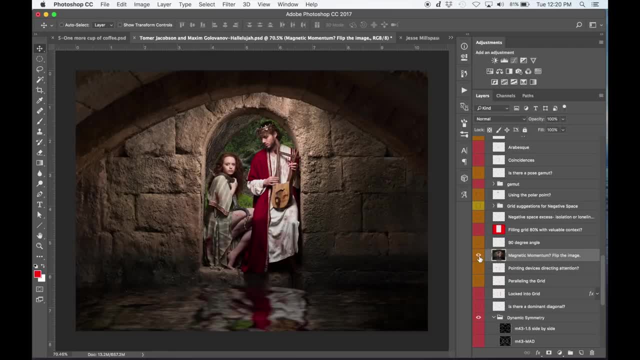 one way we can try that and test it is by flipping the image. So when we flip this image, we see it in a whole different way, the way the diagonals are creating different movement, And we can see that this- let me draw on this: 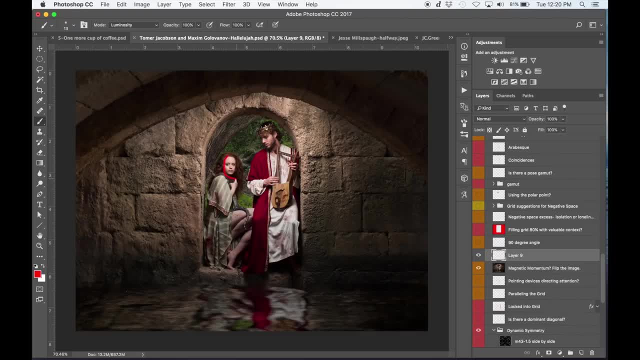 we actually see a movement. Okay, we're looking at her and we see her legs, but her legs are actually creating this movement up into the instrument, which hits the doorway and swings back around and loops. So that's a nice movement that we didn't see before. 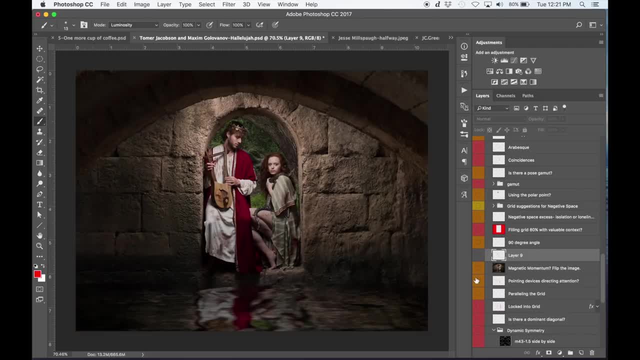 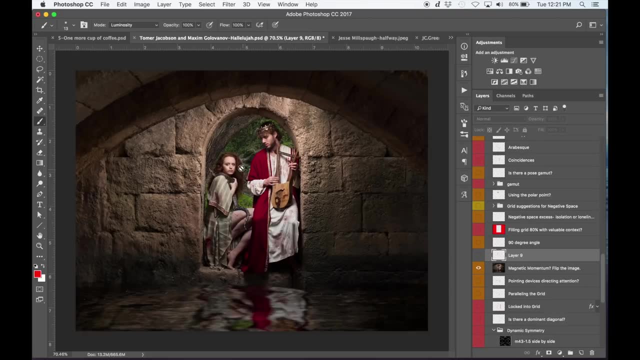 And with this one, in this one, we're reading backwards the movement. Okay, so it just depends on the story you're trying to tell. Both ways work in my opinion. I like the movement that's created with this, And she's on the left. 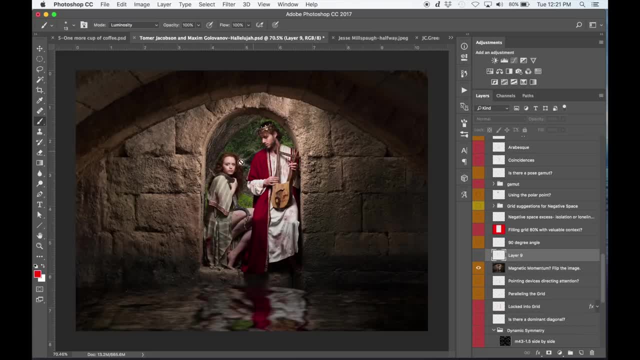 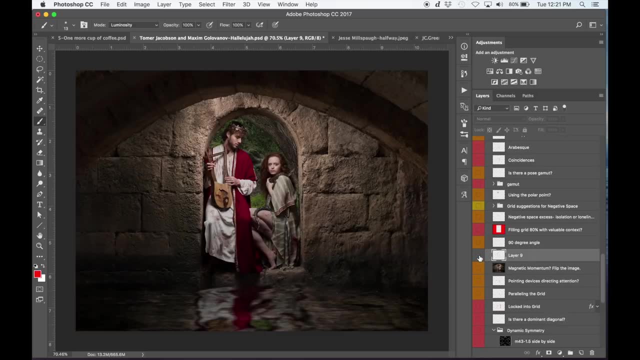 I think she's the main focal point, And then his gaze is reinforcing that. So we've got this movement with his gaze and it just keeps circling around like that. So I like that with the movement there We don't have any 90 degree angles. 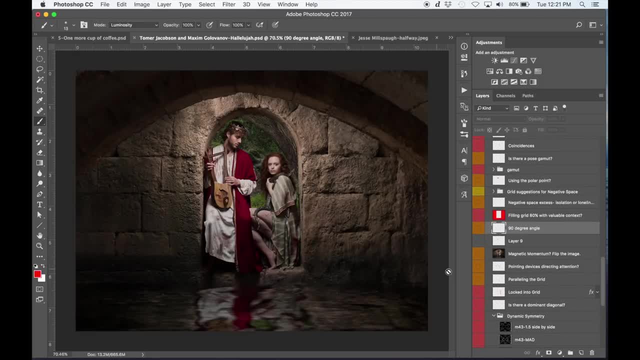 90 degree angles add strength to the image, but it's not necessary to have them. It's just something to be aware of. Like you could pose her. If you wanted to make her a little bit stronger in the composition, you could have had one of her legs, creating a 90 degree angle with her arm here. 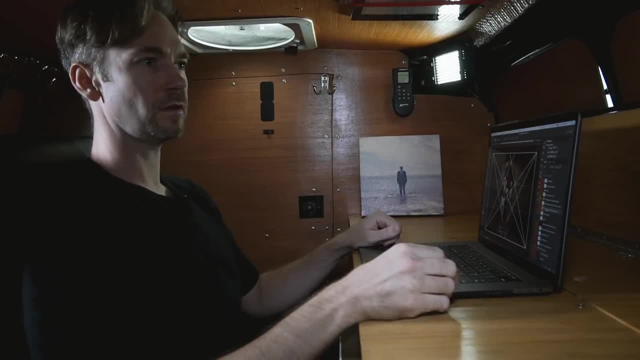 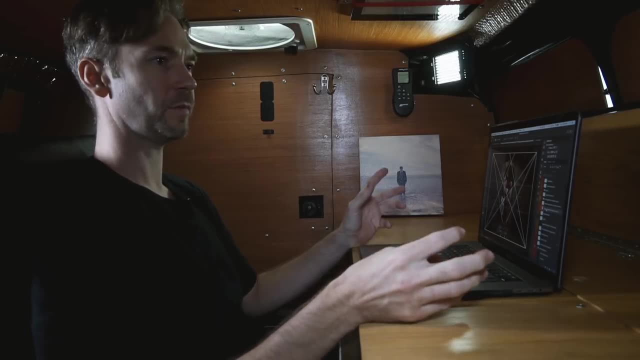 But I like the diagonals you created there. All right. so one thing I noticed when analyzing hundreds of master pieces, paintings and photos, things like that- is that they fill the grid up about 80% with context, important information, and the rest of it is negative space. 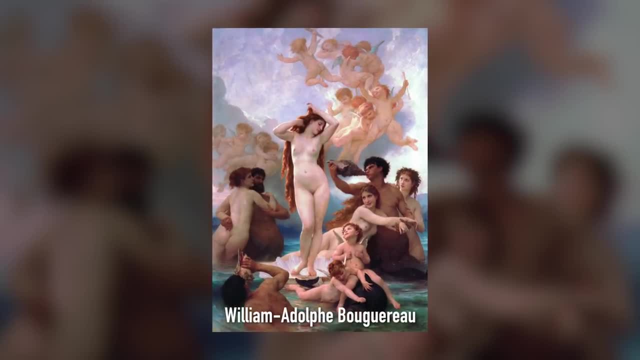 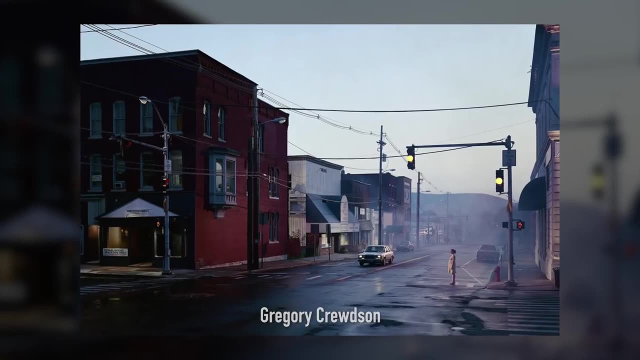 So 20% negative space, And that's not for everything. Gregory Crutzen uses tons of negative space because he's trying to portray isolation, loneliness or a scale of some kind where people are small and mountains are huge. You can show that scale like that. 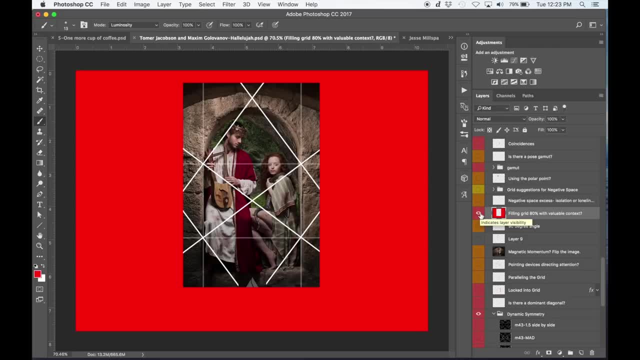 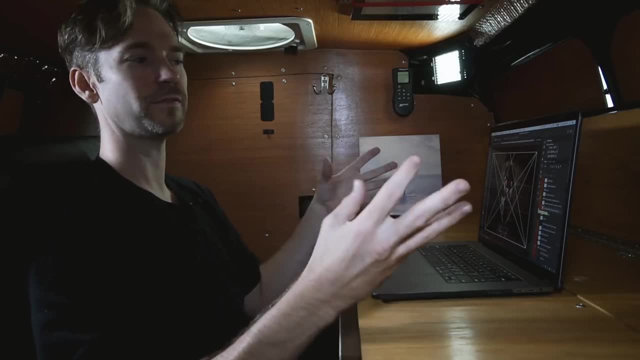 So in this case we can see that there's a lot of negative space- over 20%- And this is just a rough guesstimate. You don't have to get it precise or anything like that. It's just to give you an idea of how much to fill the grid. 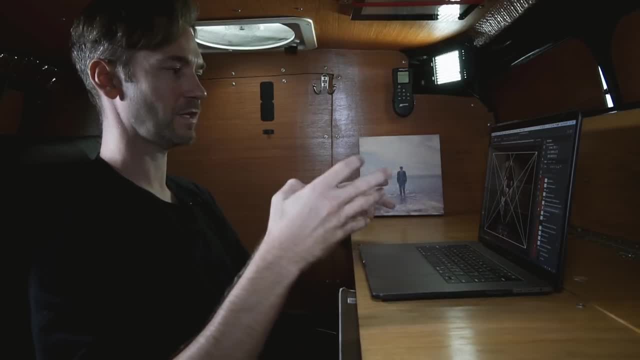 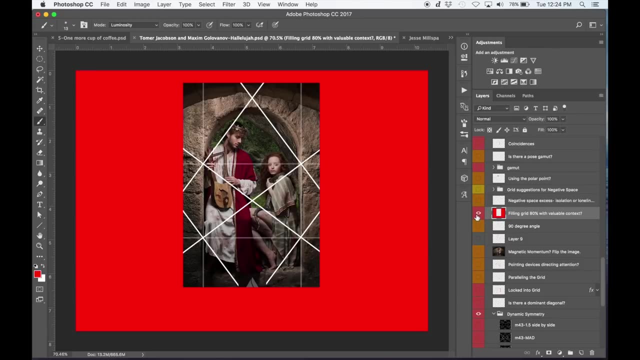 Fill it up with important stuff, Unless you're trying to portray isolation or loneliness. So in this case, with this story, you could be portraying isolation or loneliness, but this much negative space, And I love the cavernous area, but is there a chunk that can still tell the story? 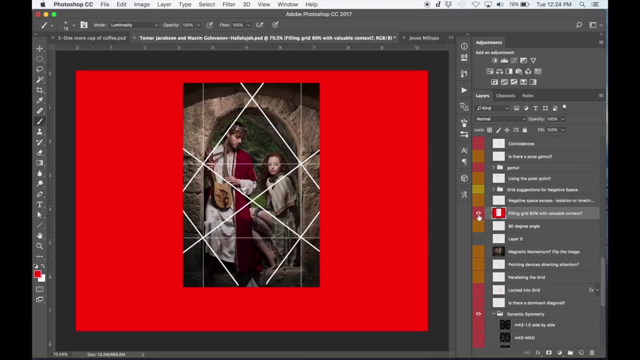 and still describe the location, but fill the grid more. That's what our question is. So I think if we shot it on location with this framework, that we'd have less negative space. We'd be focusing more on the subjects: the man and the woman and the snake. 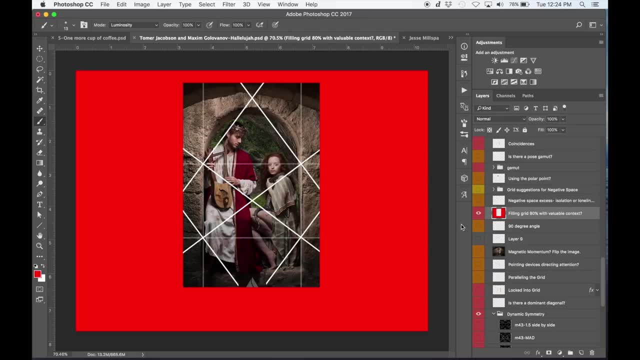 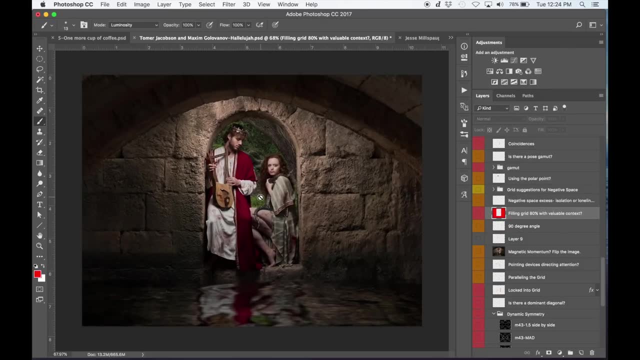 and then we could still describe a little bit of the cavern, Because once we take this framing off, we start to see that the cavern or the room has higher priority than the people within it, And that could be good or that could be bad. 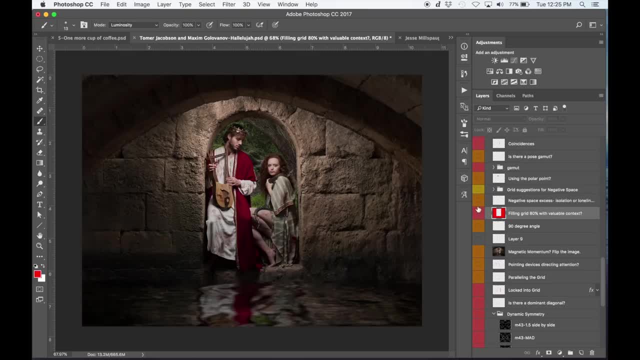 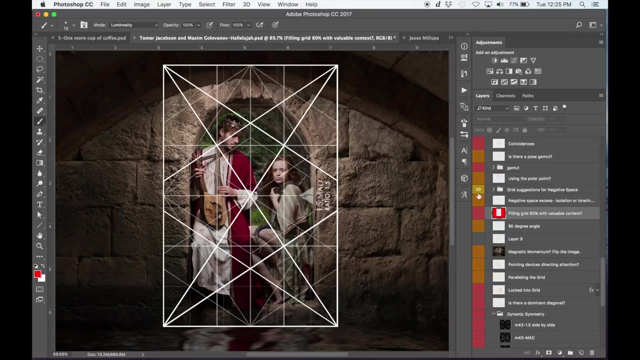 depending on the story you're trying to create. So that's just something to be aware of. So that's my grid suggestion. I would have maybe gotten a little closer to the subject and composed with a 1.5 grid, because when we look at it, 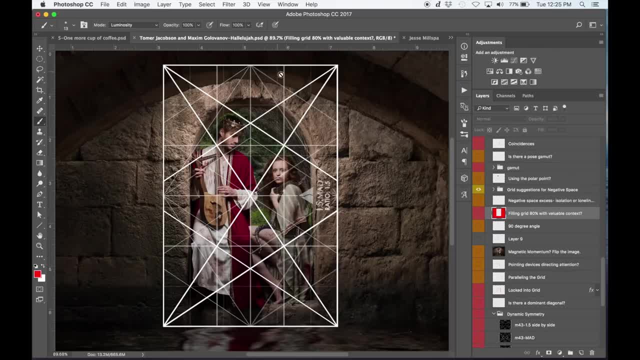 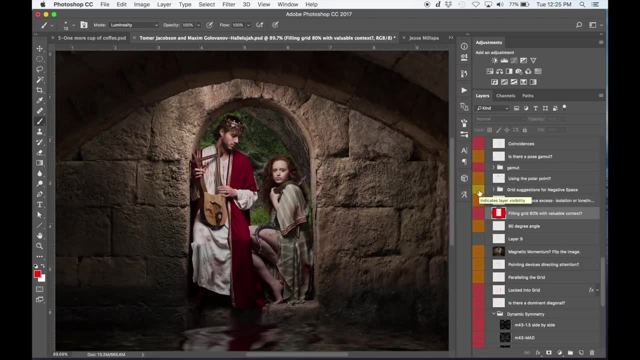 we see that it's pretty much 80% filled up with important context, and then this is the negative space around it That solidifies the story and what you're trying to tell the viewer, I think. But it depends on the story you want to create. 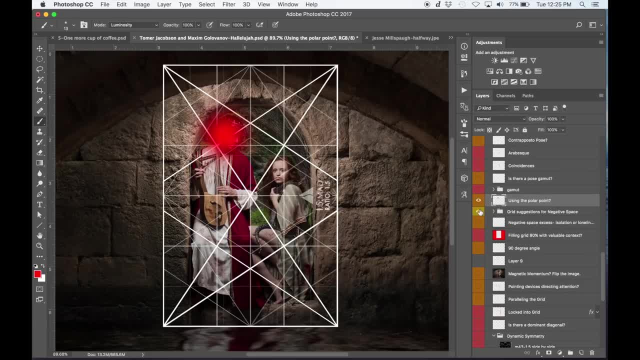 Okay, so are you using the polar point? And with this grid, the 1.5, there's a polar point. This is just something, another technique that you can look into with dynamic symmetry, If you're using this polar point. 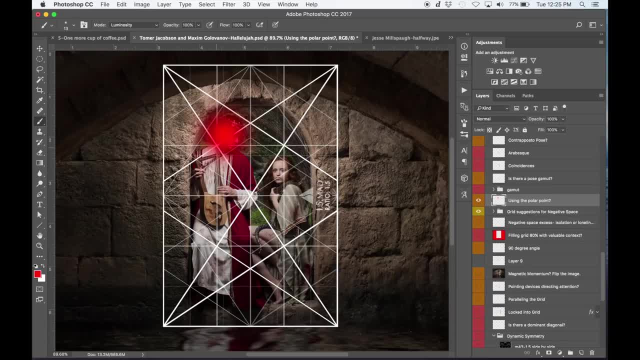 the polar point is not like a rule of thirds grid or anything like that, It's just. it can be the beginning of your composition, So it can start with the greatest area of contrast, a gaze down the sinister diagonal, a coincidence across. 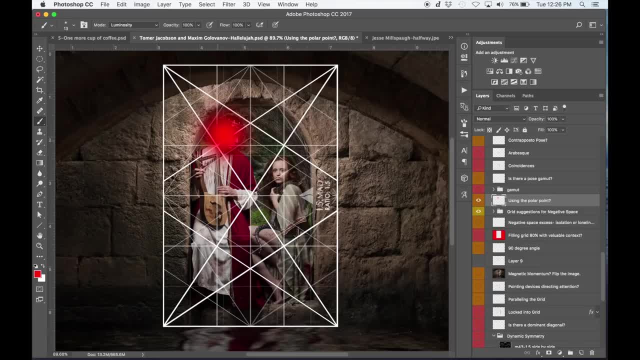 It could be a nice starting point, but it doesn't always have to start at this point. But if you look at dynamic symmetry grids, they'll. if they share the same diagonal, they share the same proportions. So let me draw on this. 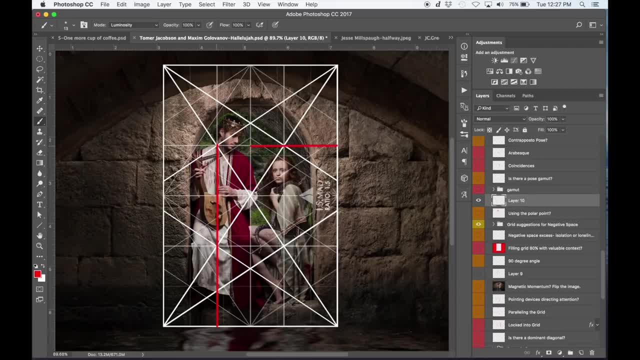 This area is a 1.5, this area, And then this area is a 1.5, this area, And then this area is a 1.5, because they're all sharing the same diagonal. So that's why I call it a polar point. 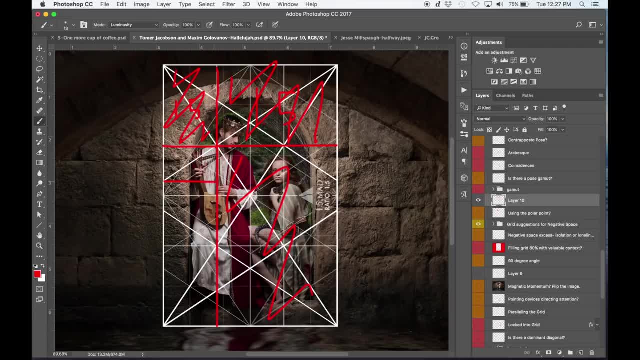 These rectangles wrap around and then this is a 1.5.. Okay, So that's why I call it a polar point, So you can start your design there if you're starting out or you don't really know what to do. but you always have to pay attention to the background. 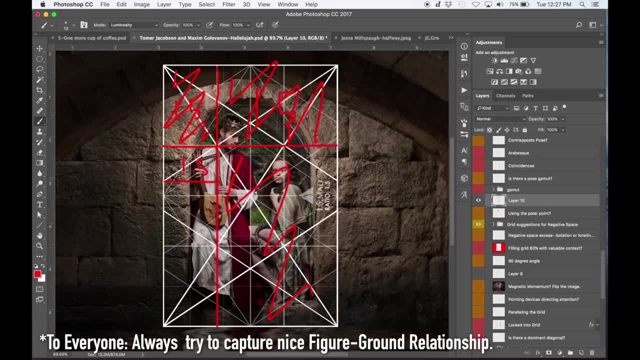 and implement figure ground relationship, because this grid is no good if you're not paying attention to the image as a whole. This is a foundation for your composition, but it's not something that you should take for granted. It's gonna help you promote unity, movement and rhythm. 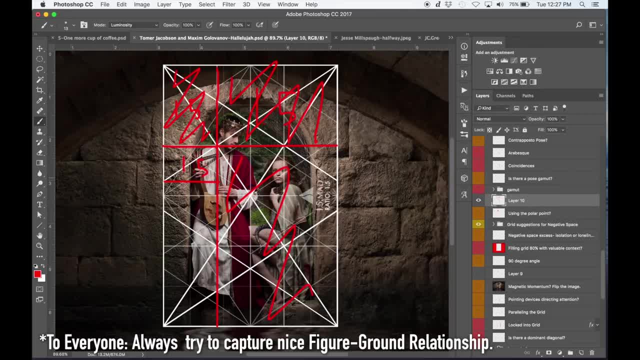 by coincidences, gamut, dominant diagonals. You can't ignore the background, especially figure ground relationship, because if your message isn't visually clear, then the whole image is gonna fall apart. So you have to pay attention to that And you're doing a good job. 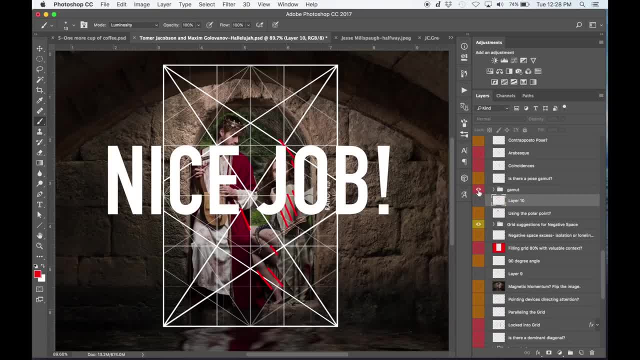 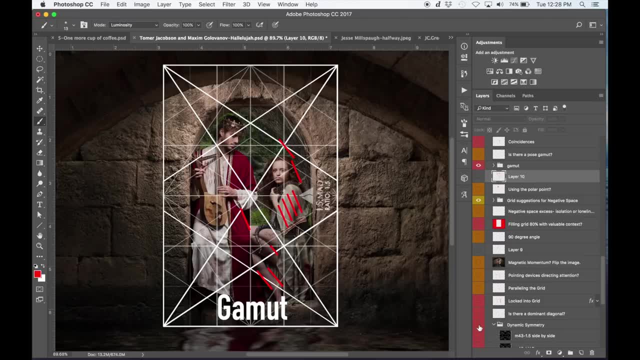 I'm not saying you did a bad job. You're doing very well and you're on your way to creating even more masterpieces. Okay, so the gamut: These are all diagonals derived from the basic armature, So I found them by lining up the diagonals. 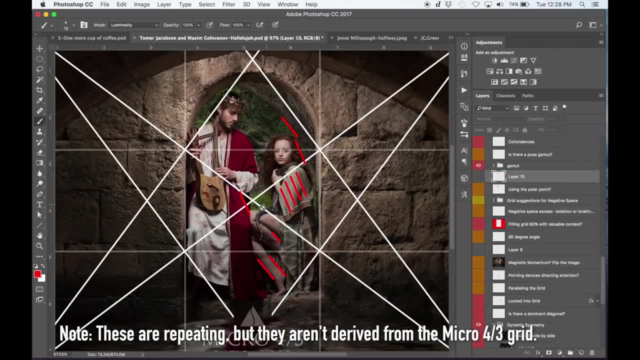 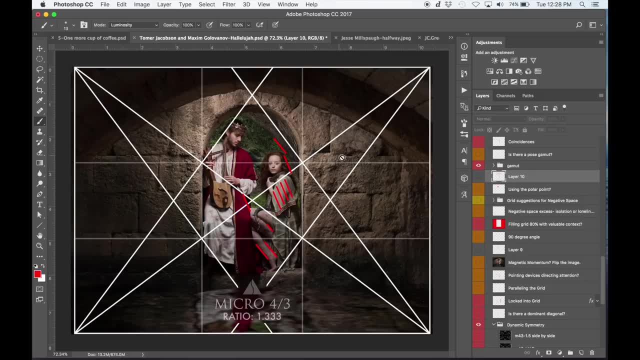 of the micro four-thirds grid and seeing if anything repeats throughout the composition, And we can see a little bit of repetition. This can have a stronger impact if you create the same diagonal within the background or the foreground or both subjects multiple times, like the master painters. 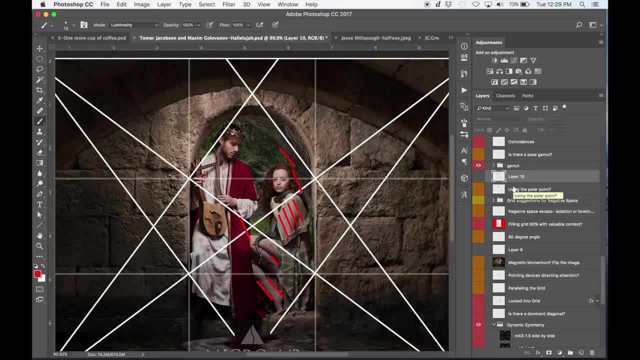 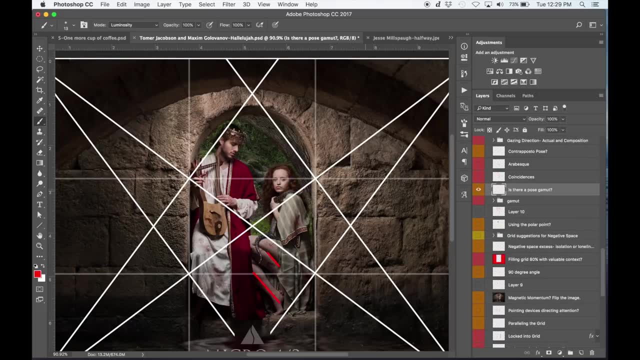 And you'll start to get a rhythm across the image And it's a hidden thing that impacts the viewer the way they see your work. It's a pretty cool technique, Okay. so we look for pose gamut if there's a rhythm or repeating diagonals within the pose. 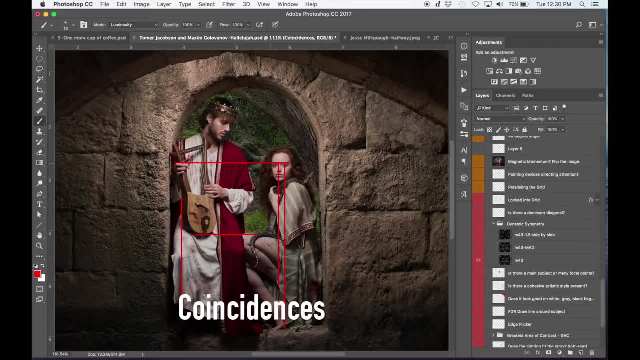 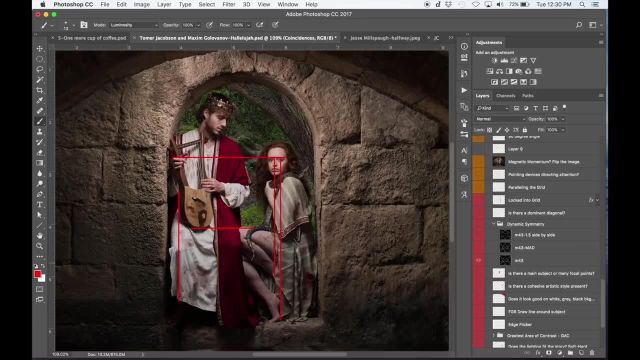 And we can see that there's a couple diagonals there. So coincidences are edge-to-edge relationships that create movement and unity, And you've got a couple here, And these can also be increased to create even more movement and unity across the background, foreground and the subjects. 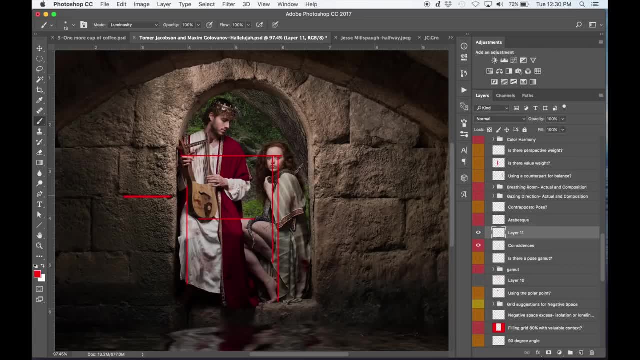 So like if his arm were coinciding with this line in the wall, that would create a coincidence And it'd create unity with the wall and the guy's arm. So the arabesque is a curvilinear element and it can be used to create unity and movement as well. 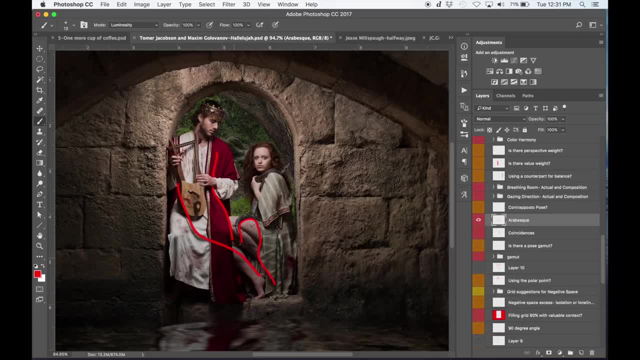 And it's a sign of beauty. It adds a beautiful movement throughout the image And we can see a couple here with the snake's tail wrapping around the wall And then down the instrument, across his robe and then down to her leg, And these are hidden, which is good. 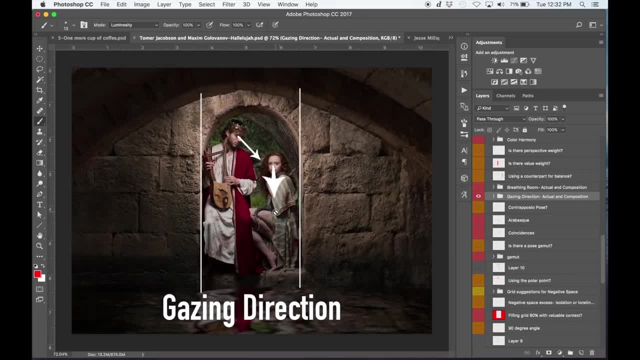 So we've got nice movement there. So gazing direction affects the balance of the image And since they're composed in the center and their gaze is beneficial to the viewer, we've got a nice balance. His gaze is going to her and hers is going to us. 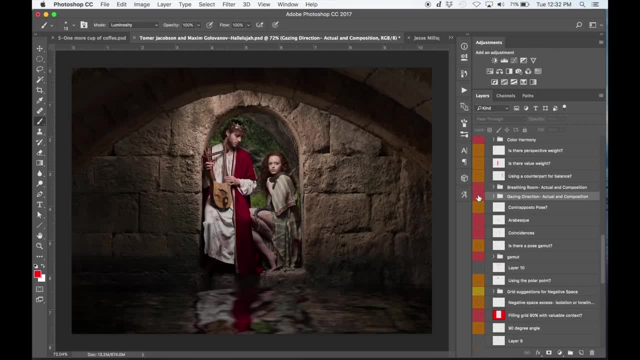 And the balance is nice and even there, from left to right, The breathing room is the balance from top to bottom And we can see that if we take the bulk of the image and draw a line here and here, we see there's more negative space on the bottom. 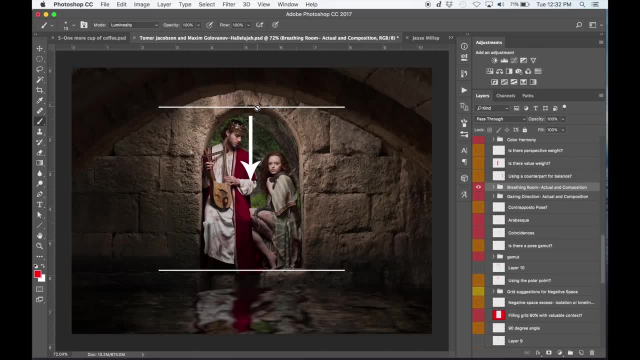 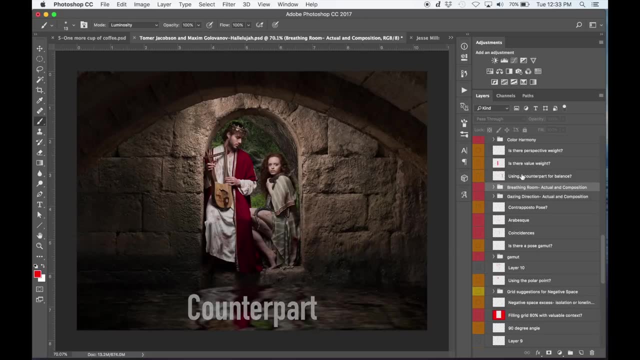 than the top. So we see that the balance of the composition is going from top to bottom. So we see if you're using a counterpart, which you are, because she's the counterpart of him, and vice versa. Is there value weight? Yes, because his light wardrobe. 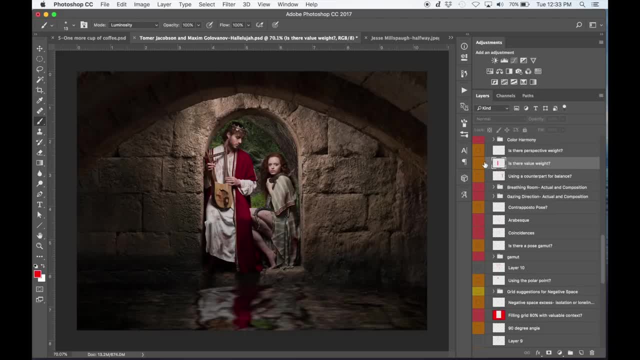 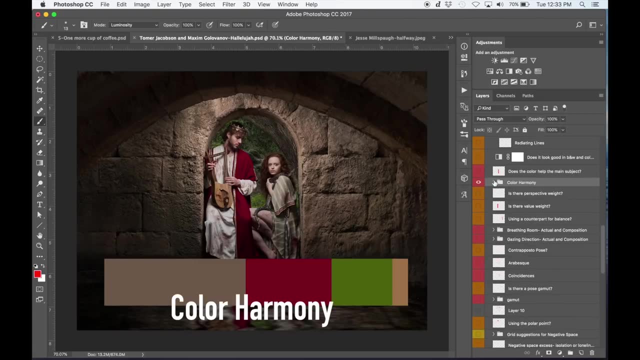 creates some weight on the left side. You know the contrast of his wardrobe against the red that creates weight on the left side, which is balanced by her on the right side. The color harmony in this. typically I teach that you should have. 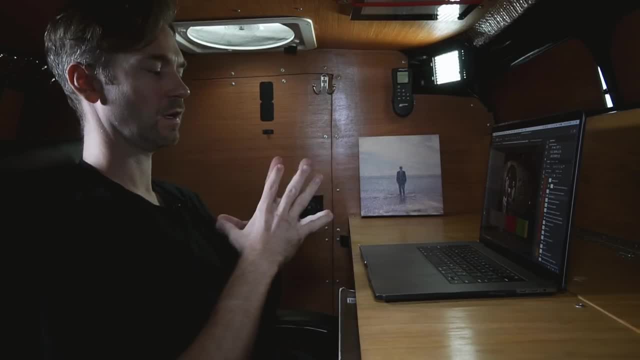 red, blue, green and yellow to present color harmony in a nice way, And there should be a hierarchy amongst those colors, So the majority of it could be red and then secondary could be blue and then some yellow and then a little bit of green. 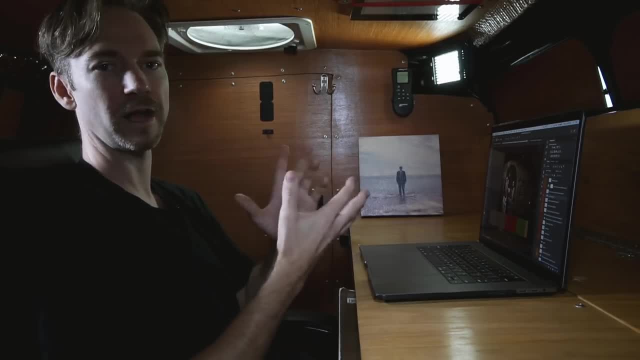 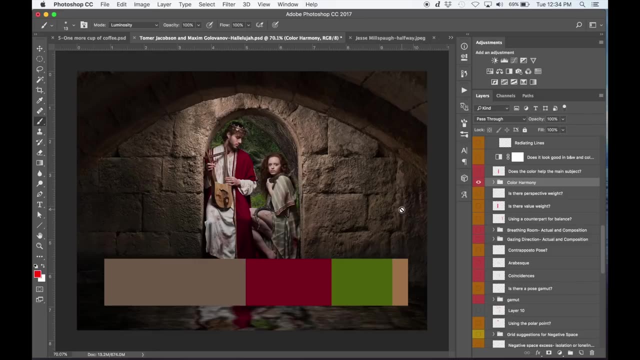 And that's what I teach as color harmony and color hierarchy. So here we have red and blue and there's a little bit of yellow on the instrument there, and then the rest is neutral. So to say that you have color harmony, like the master painters. 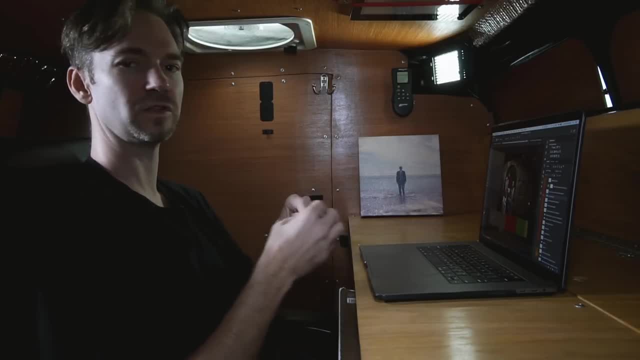 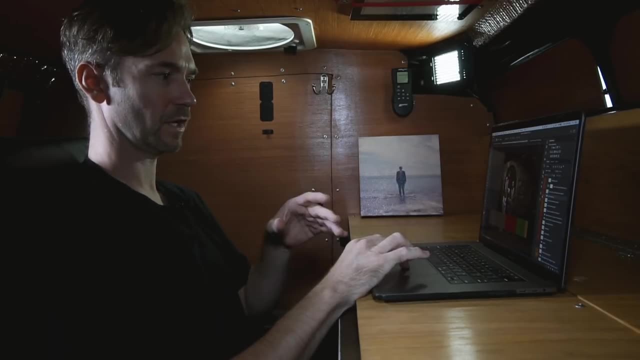 I would say we're missing blue in there. So if you add a little spark of blue it might bring the whole palette together a little bit nicer. But I do love seeing the color red in images and you're working it with a complementary color. 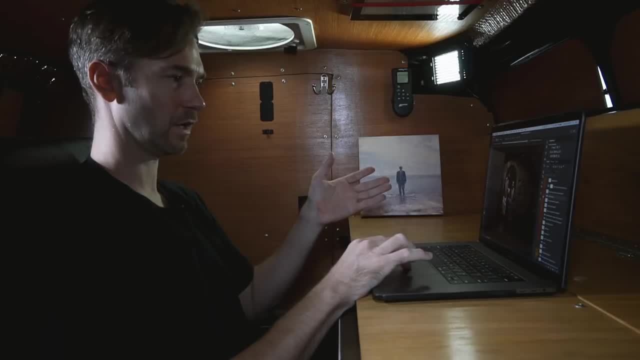 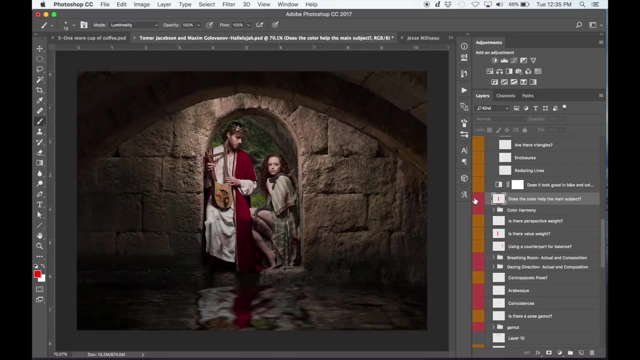 which is green. So you're still doing a great job on color, And color actually symbolizes a bunch of things which I'm not gonna cover now, Like: green symbolizes certain things, Red symbolizes certain things, So does blue and yellow. 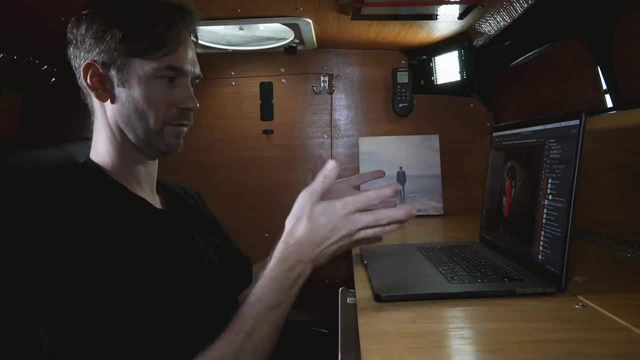 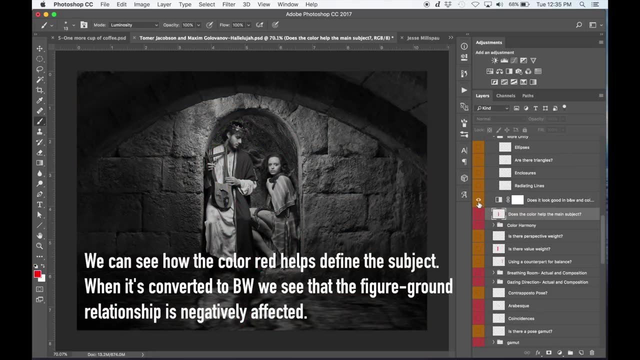 They all have an effect on the psychology of a person, the way they view your art. Okay, does it look good in black and white? and color? Yes, it looks pretty well in black and white, And this is just to see if color helps define the subject. 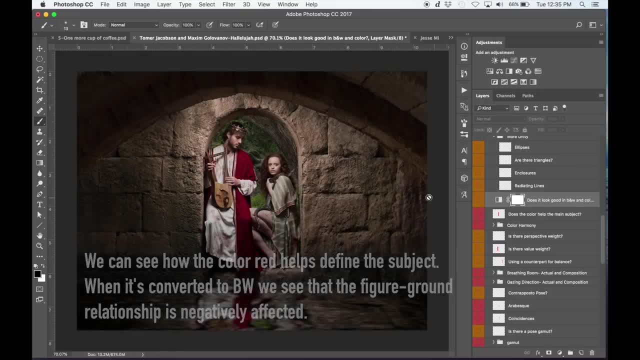 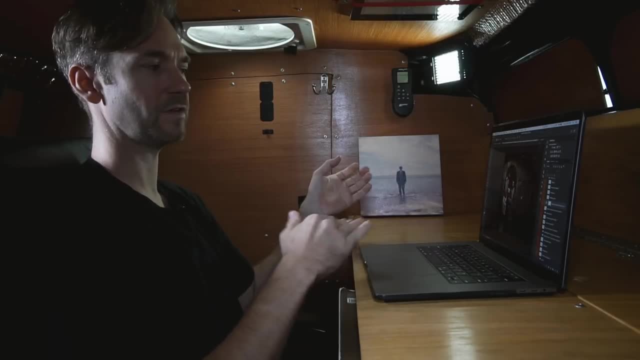 if it's distracting from the subject, If there's no color at all in the image, then, depending on what you want, I would recommend, you know, trying it out in black and white, See if it just creates a different story, a different mood. 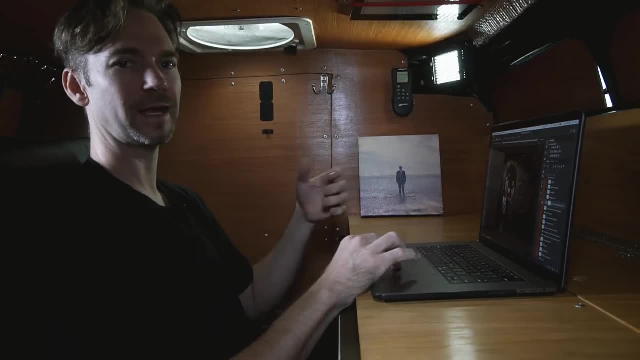 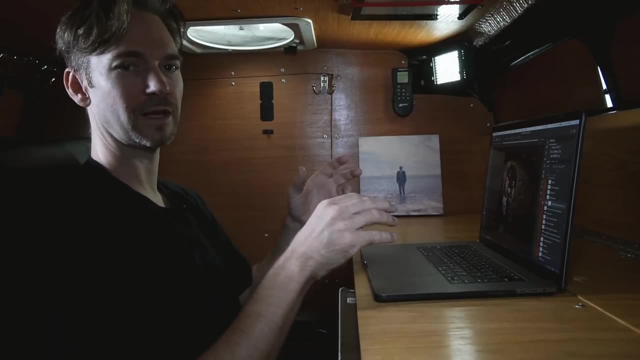 and makes it look a little better. If you're shooting film- black and white film or color film- I would just keep it as you shot it. I don't like converting color film shots to black and white. I like to keep it as pure as possible. 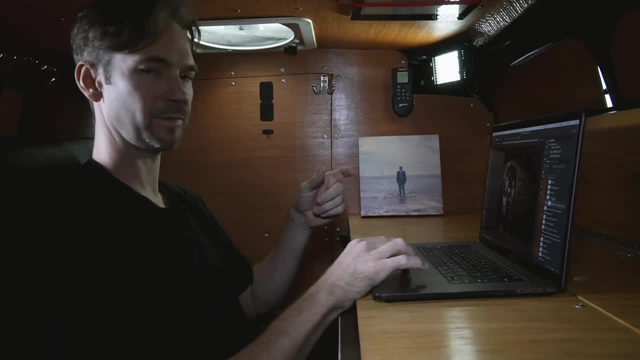 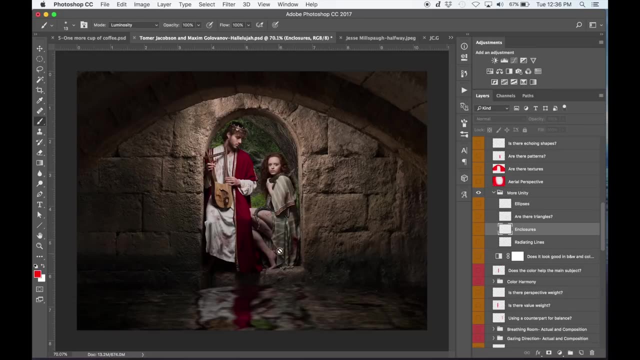 But test it out, See what it looks like black and white or color, because you'll be surprised sometimes. So are there triangles? Yes, I see a little bit of a triangle here, going across the arm, down the leg and then up this line here. 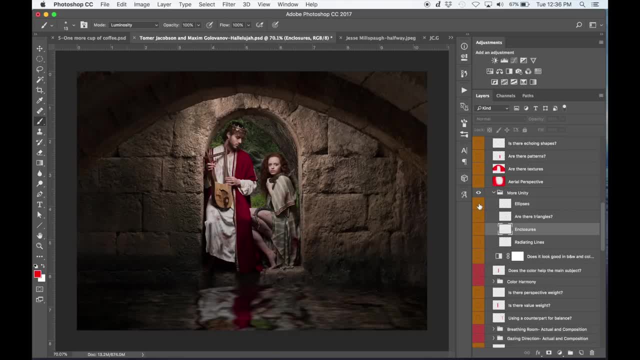 This is the line in her wardrobe, So there's a little triangle there, which is nice. Aerial perspective: yes, The way they lit it, We've got depth added and created by the use of light, which is aerial perspective. Are there textures? Yes, 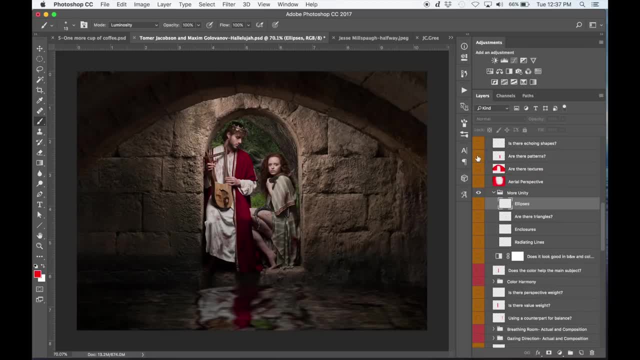 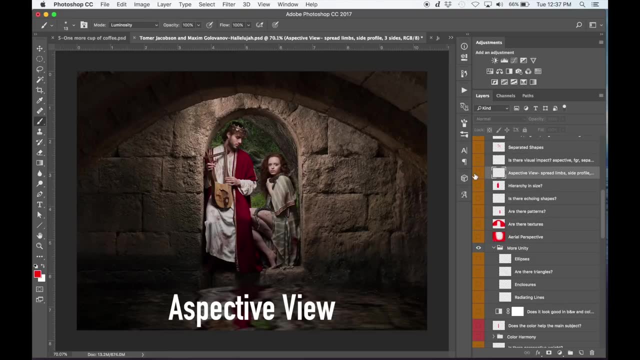 Plenty of textures in that, Plenty of patterns in the wardrobe. Is there hierarchy in size? Yes, He's larger than her and then she's larger than the snake. Aspect of view: we've got a little bit of aspect of view with his face. 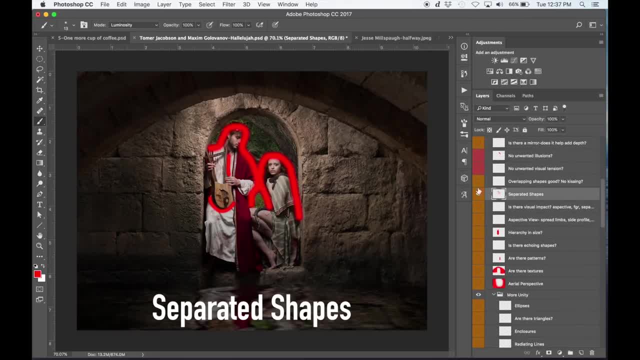 the side profile of his face. Separated shapes kind of. but the figure-ground relationship is a little bit weak in these areas, so we don't see the separated shapes and get the benefit of it like we should. Overlapping shapes- decent. 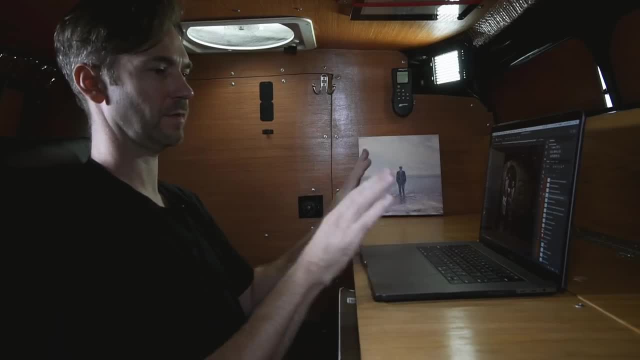 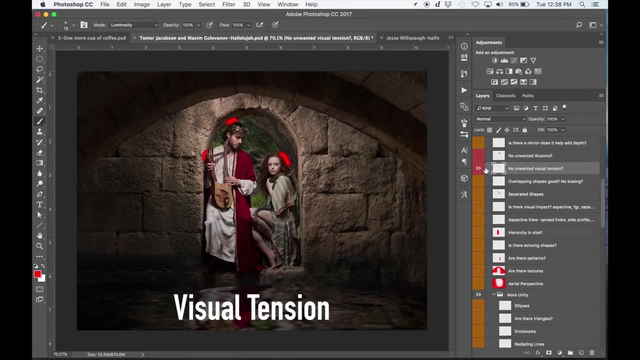 There's no kissing that. I could tell where edges meet each other and you can't tell what's overlapping each other or creating unwanted illusions. Visual tension: Is there visual tension? A little bit, because this is very close to the wall. His head is very close to the doorway. 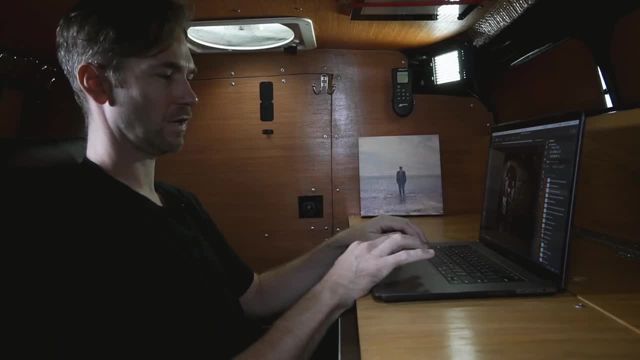 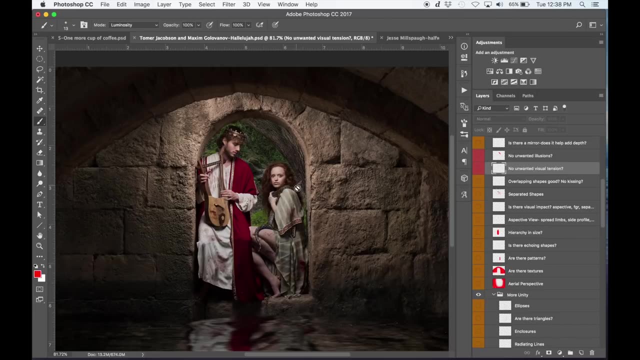 Her head's very close to this. so in art class with Myron Barnstone he called this a gutter, so it creates high contrast in an area where you probably don't want any eyes to go. This area's not very important- the back of his head. 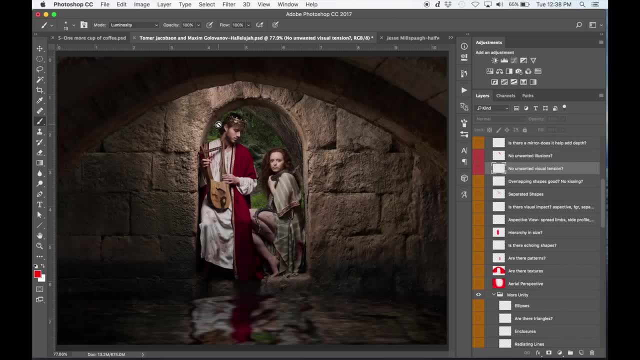 so since there's this visual tension and things are so close together, we're getting a high contrasting area and we don't want the viewer's eyes to go there. so one remedy to that is just to either subdue this area, the contrast seen there. 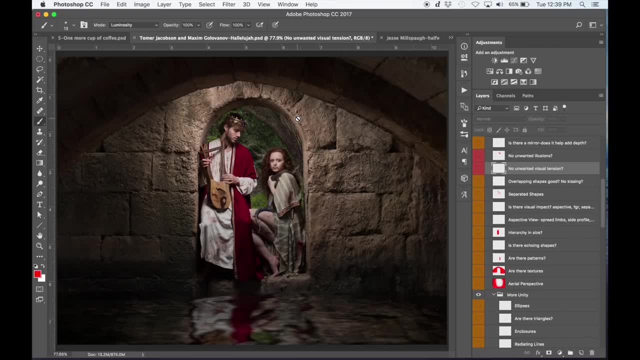 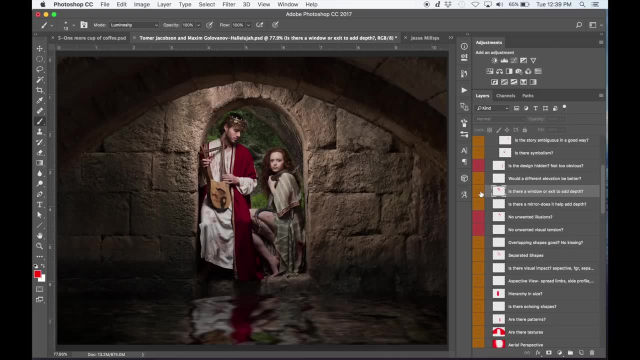 or give it a little bit more negative space So it's not quite as close. Is there a window or an exit to add depth? So we've got a nice exit here for the eyes. It's not too deep behind them to give more context to the image. 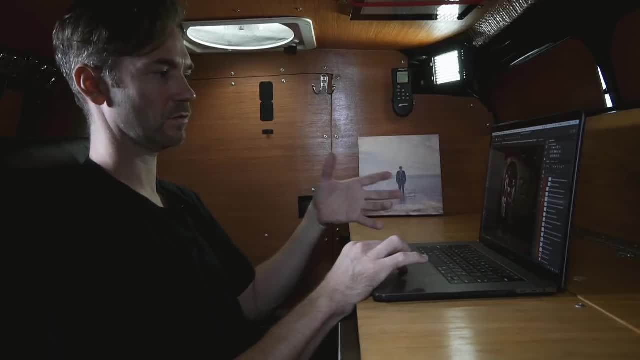 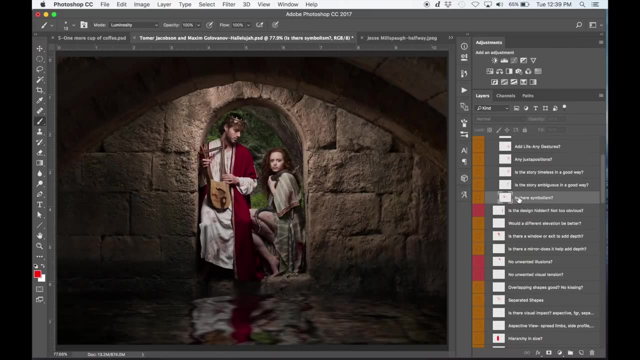 and let the eyes travel back and forth, but it still allows the composition to breathe a little bit more in depth. behind them, Is the design hidden? Yes, Is there symbolism? Yes, We've got the snake, the crown, the instrument. 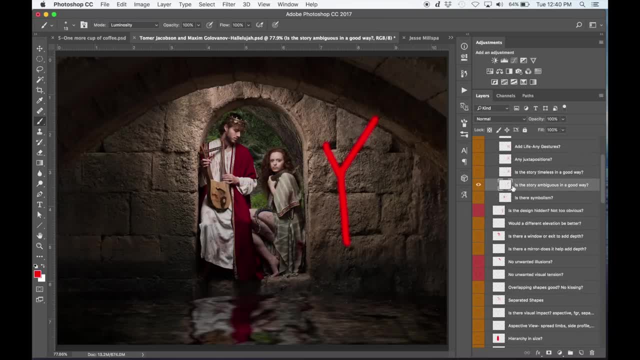 All these things are different symbolism, different symbolisms to help tell the story. Is the story ambiguous in a good way? Yes, I think it is. We don't really know what's going on, but we can create our own story- It's not too obvious- of what's going on. 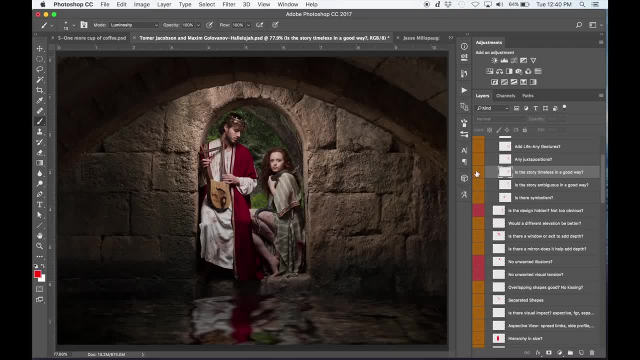 Is the story timeless in a good way? Well, no, it's not very timeless. We know it's kind of a set in the older period when there were kings and people like this playing the instruments like that. I don't know what era that is. 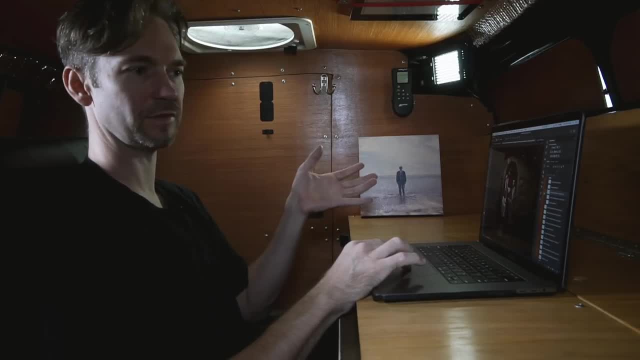 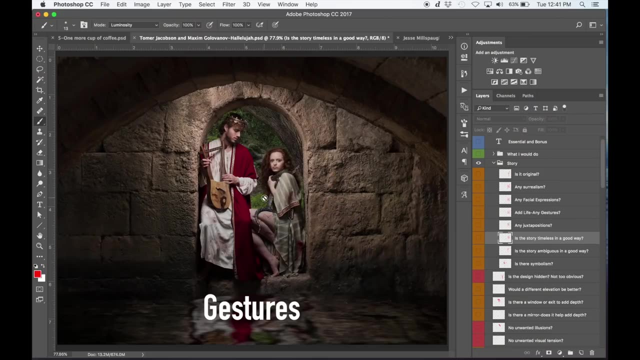 but we can tell it's definitely set at a certain time. You can't be mistaken for the 70s or the 1800s. It's further back than that. Any gestures- No Gestures- add a little bit of life to the composition. 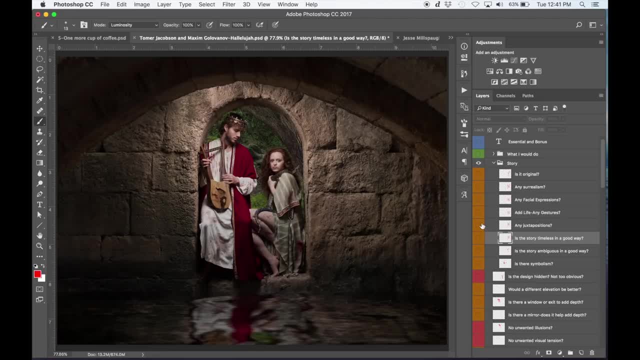 so it's always good to include a gesture if you can. Facial expressions add a little bit of life also. If her eyebrows were pointed upwards in the middle, maybe she would be showing concern If his mouth were frowned down just a little bit. 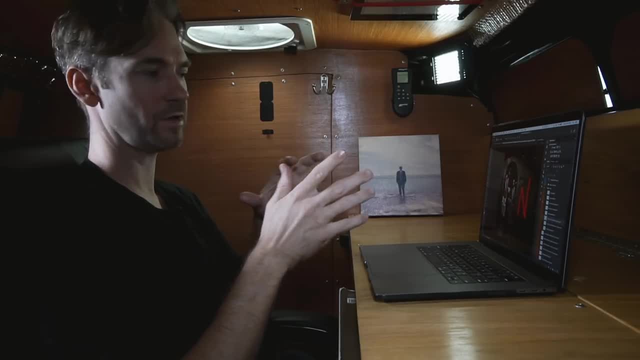 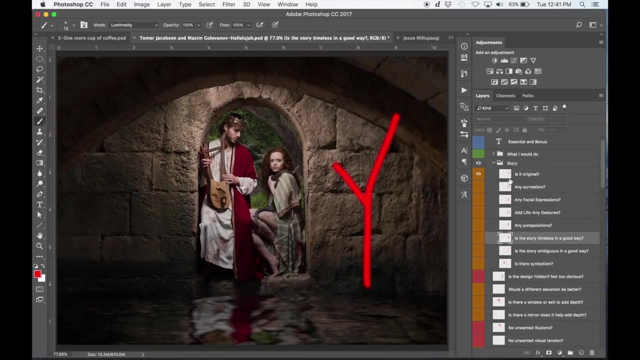 maybe he would be presenting a little bit more context for the viewer. So facial expressions are gold sometimes and they can help tell your story. Is it original? Yes, I've never seen really anything like this. I also like to show what I would do if this were my image. 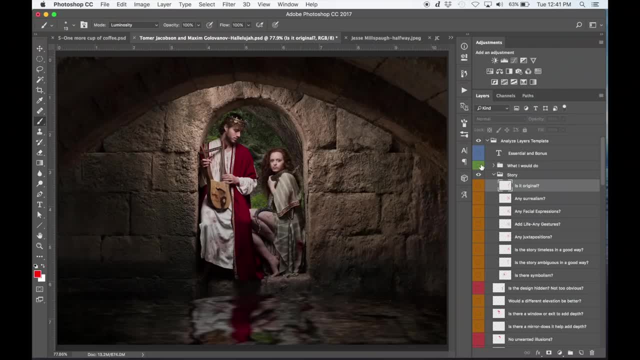 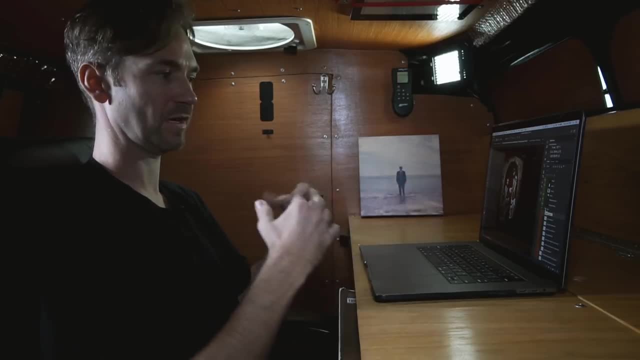 and I were editing it to present it online or in a portfolio. So I edited all that, And this isn't to say you should do this. This is just to say like if it was mine, Based on the design techniques and the story I would want to tell. 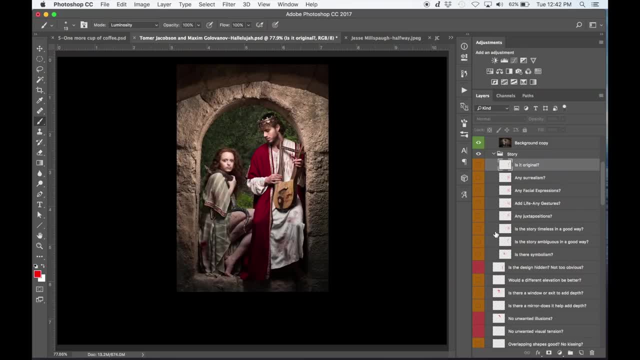 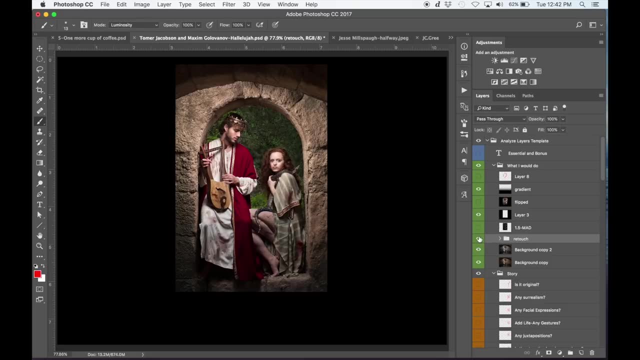 I would make these adjustments. So I would have flipped it, I would have framed it differently with the 1.5 grid. So let me take this off and show you the way I retouched it. So I darkened some of these areas on the wall to reduce the contrast. 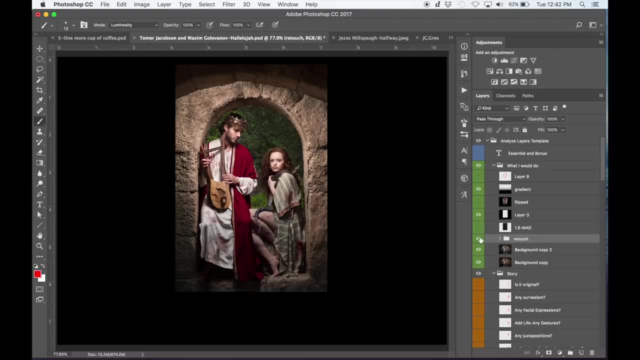 because they're drawing more attention to itself than the man. I simplified the background, took out that tree, because that tree was creating an illusion like that was the doorway, because it's sharing, it's coinciding here and then it's sharing the same curve going up. 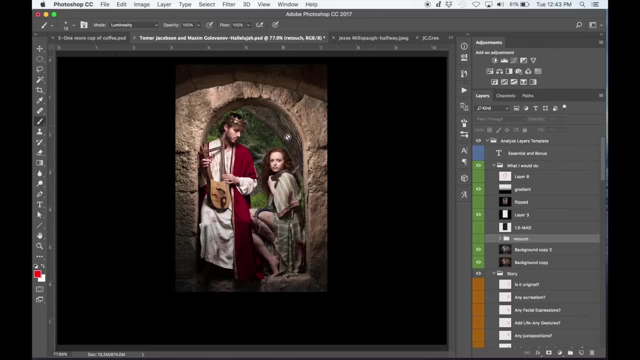 So it's easy to mistake that for some type of 3D-ish doorway. at first I thought it was part of the doorway at first And then I got to looking at it and it was a tree. So I took that out, adjusted the high contrast in the background. 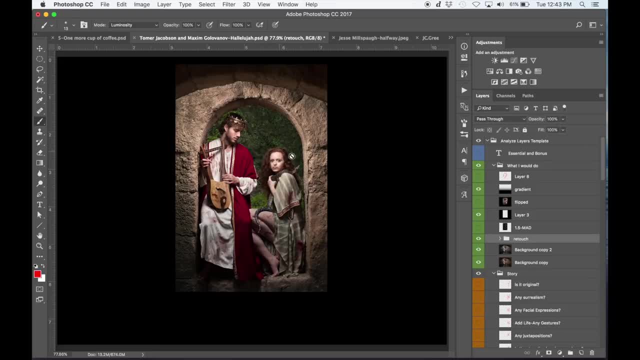 near her face or near her head. tried to improve the figure-ground relationship with dodging and burning around their heads. improved the figure-ground relationship on the snake. reduced the contrast in his robe, cropped it like I said, I flipped it to take advantage of this movement going up there. 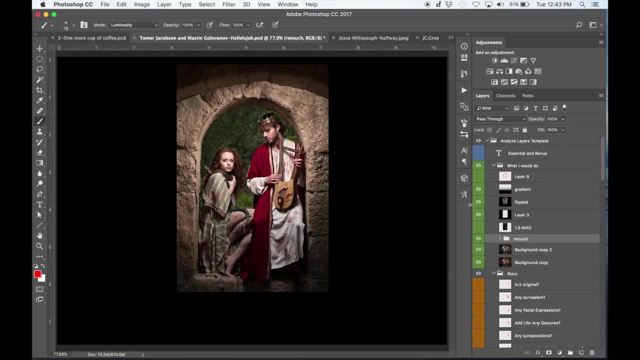 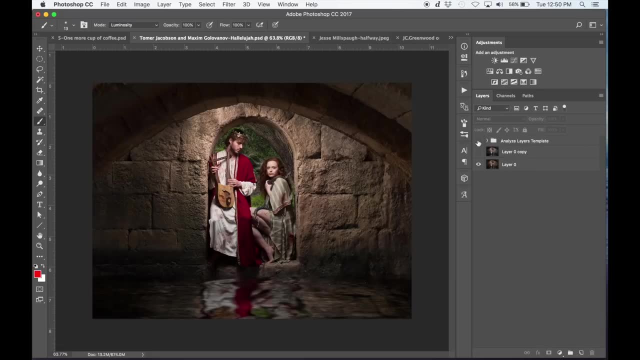 And then I reduced the contrast a little bit more with the gradient at the bottom, just so the eyes go up to the people more. All right, so let's just take a look at this before and after. Before and after Before: after. 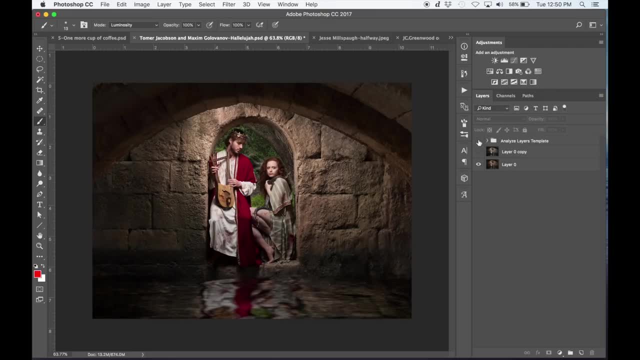 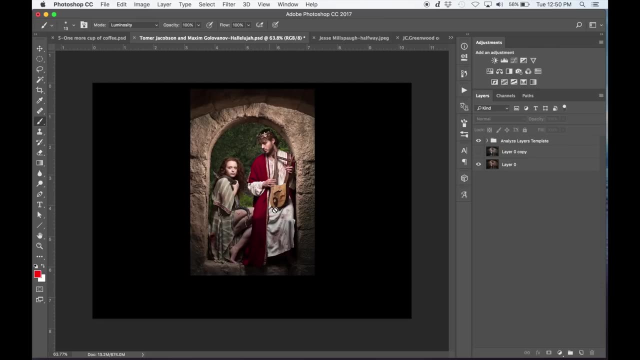 I love this cavernous area, but it depends on the story you're trying to tell. This would be the story I'm trying to tell: to get closer to this snake, find out what's going on. see the blood on his wardrobe. 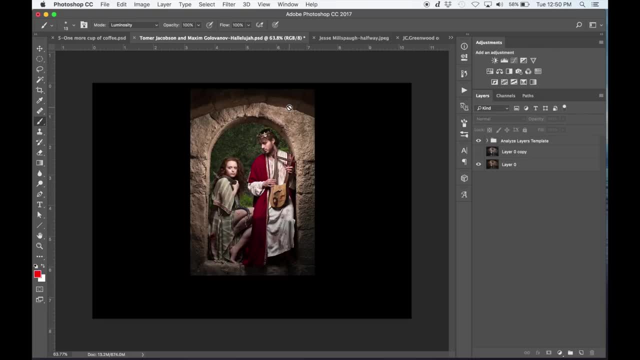 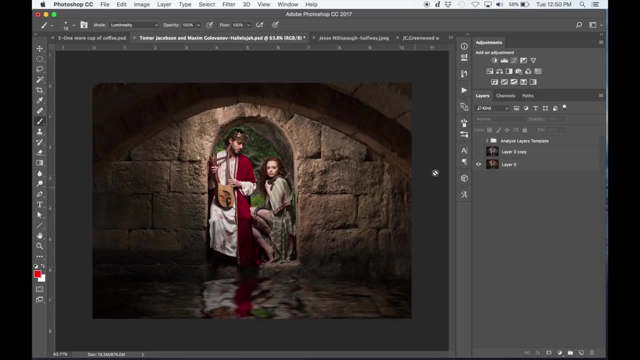 and then the cavern area can take a bite. This is the back seat to the story. So that's before and this is after, And we don't have people questioning our water reflection here. just straight to the point to the story. 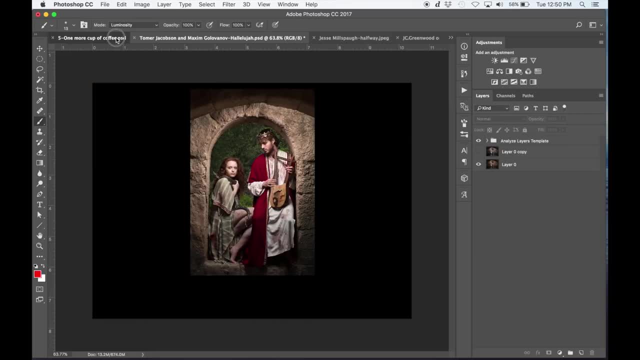 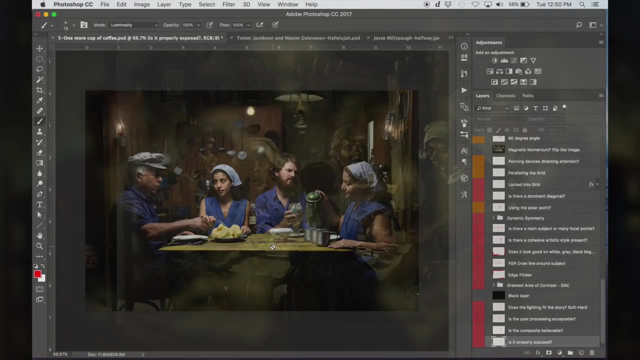 and going about it that way. So let's take a look at his other one. Good job, you guys. This one's pretty cool. It's a reenactment or recreation of a Van Gogh painting, and I'll put that up there. 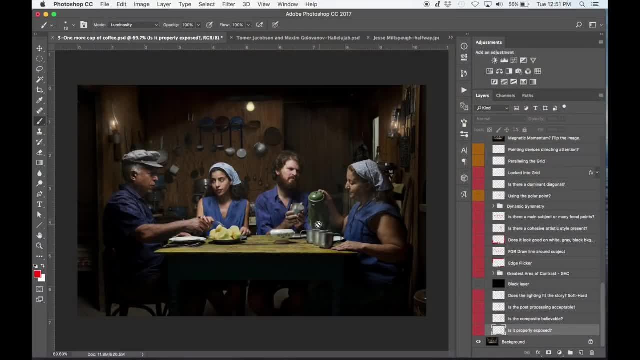 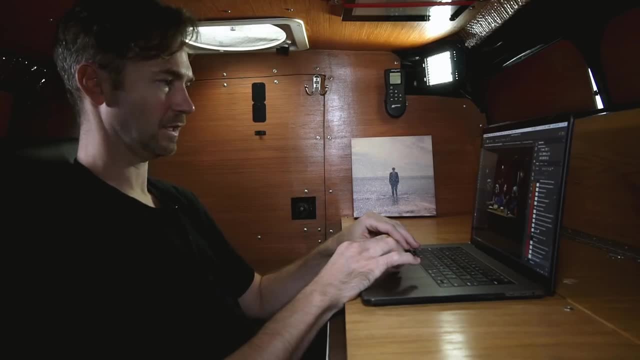 I think it's called The Potato Eaters. That's a Van Gogh painting and this one seems to be inspired by it. I don't remember which song it is, which song you guys chose to create this one, but people see and imagine stories differently. 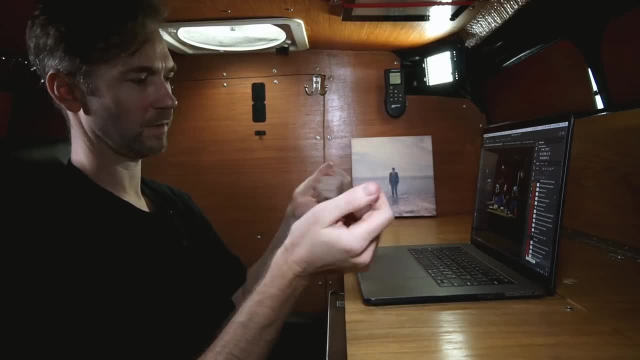 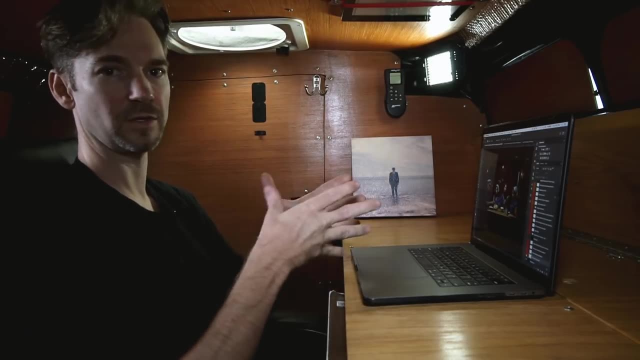 depending on their whole life experiences, not just random songs or anything. So the way you guys see this image when listening to that song is going to be a lot different than how I see the image when listening to the song. But let's just look at the visual effects that are remaining for us. 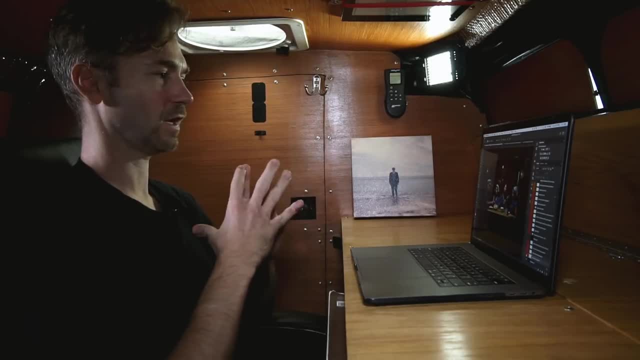 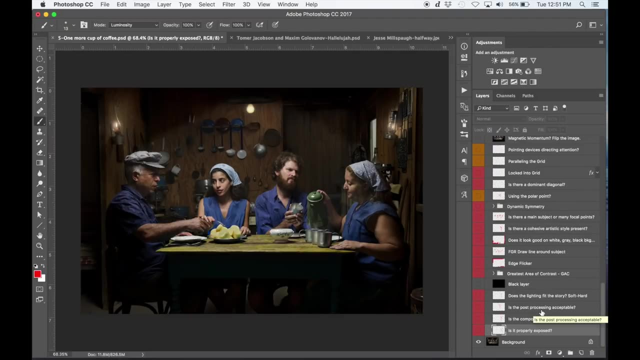 just like we do master paintings and kind of see how it works and how visually clear it is. So we can run through these a little bit quicker, because we covered all the techniques in the other photos, So let's just get into it. 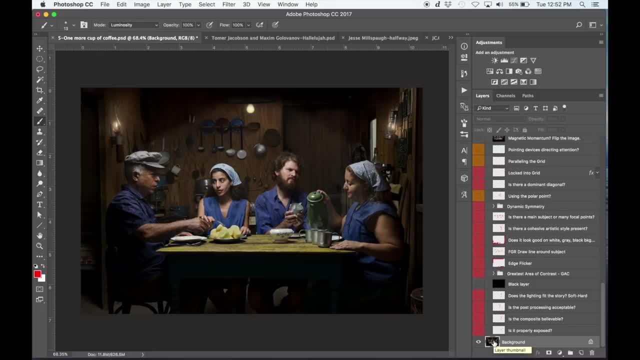 Is it properly exposed, Just like the other one, it's a little bit off exposure and I'm not sure if that's because of the way you're trying to tone it or maybe our monitors are different. But a good way, like I said, just do the auto color thing. 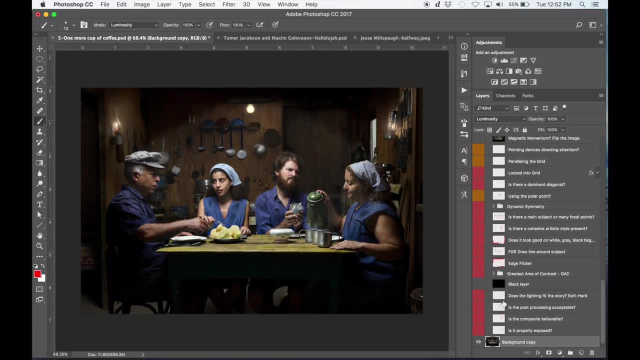 and see what it does, and then set it to luminosity and see if it gets brighter or if it stays the same. The processing looks good. Does the lighting fit the story? Yeah, it's a soft lighting. I noticed you have these lanterns here. 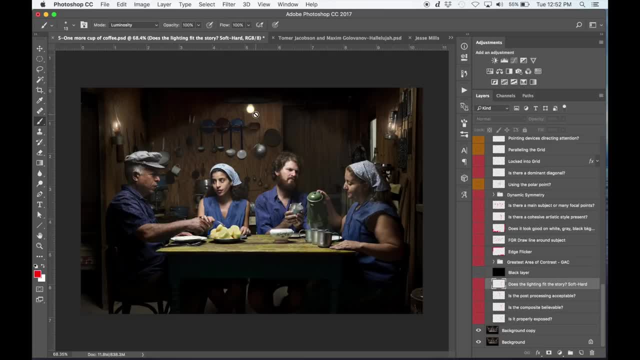 I'm not sure if those are composited. Looks pretty good. Same with this light, But we can tell that the light, the majority of the light, is coming from above, which is probably why you have this light here. Maybe you could add more lighting coming from here. 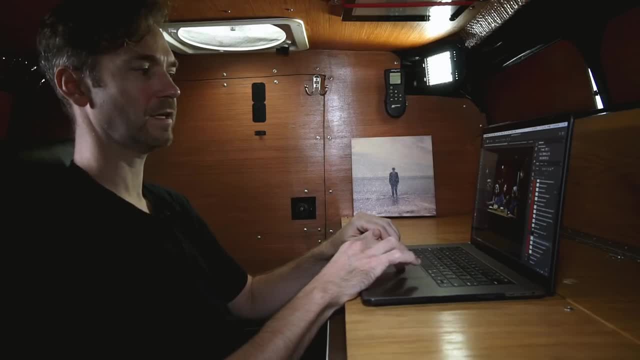 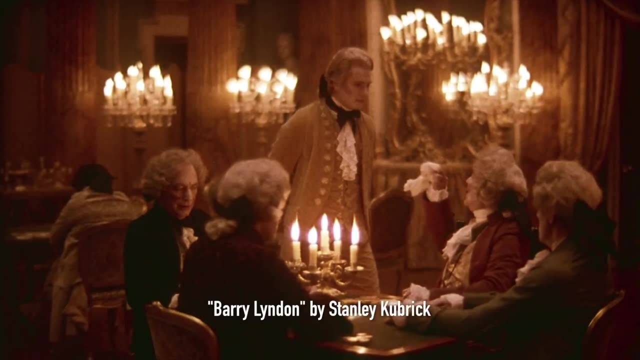 Like I just wrote an article on Stanley Kubrick's practical lighting. So he takes lighting that's actually from the scene or would be seen in the actual environment and he creates the lighting around that and doesn't have the artificial lighting because the way he's telling his story 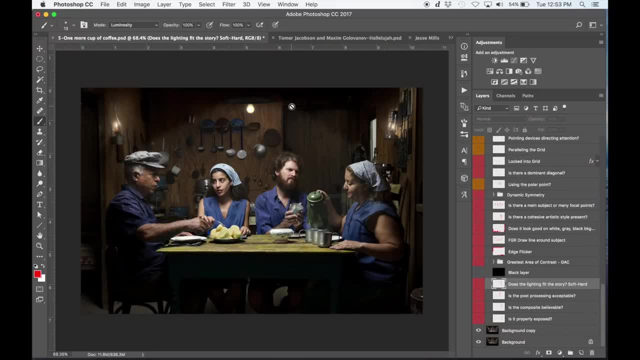 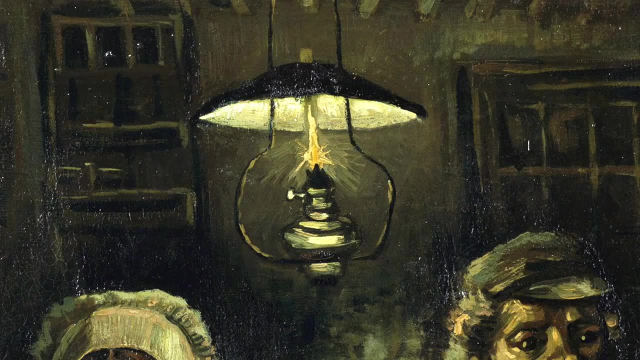 it's presented as being more authentic, And maybe some nice candles lit on each side of these people and a candle chandelier like we see in the Van Gogh might have lit the scene a little bit better and more authentic. So this is an updated version of what we could have seen. 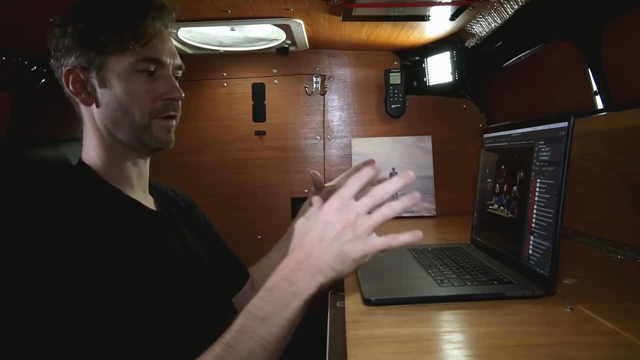 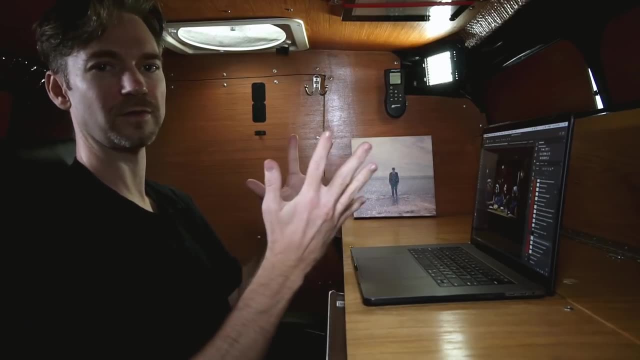 You could have set the mood and the timeframe a little bit better if you actually used the lighting from these lanterns. Not to say your lighting's bad or anything like that, It's just another option for you to deepen the story you're trying to tell. 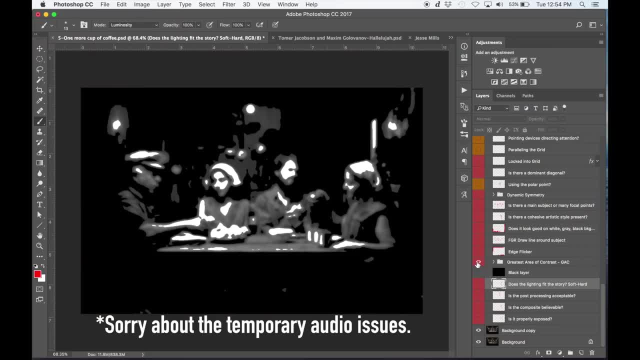 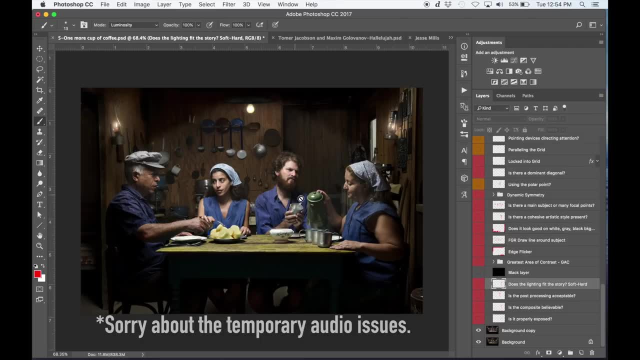 So let's go into the greatest area of contrast. What I see is that this girl catches my attention more than this man asking for another cup of coffee. You titled it- One More Cup of Coffee- which gives the viewer an impression of where they should look. 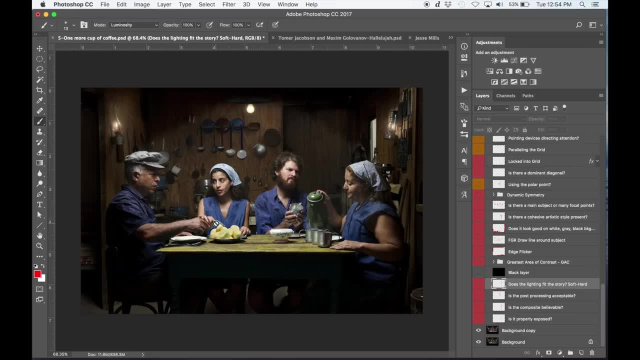 and what the story's about, But without the title. and, looking at this scene, I'm seeing this woman as the main subject and what their interaction is- hers and the man's on the left. Not this interaction, which is probably where you wanted us to look first. 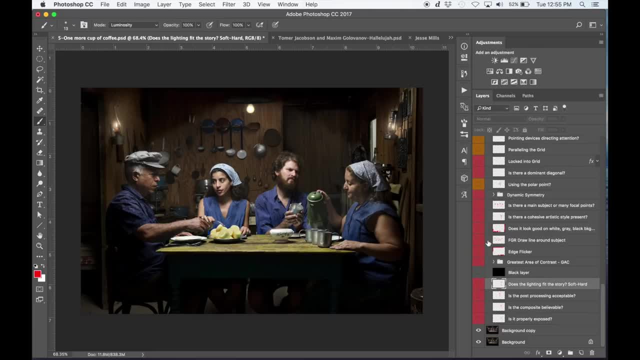 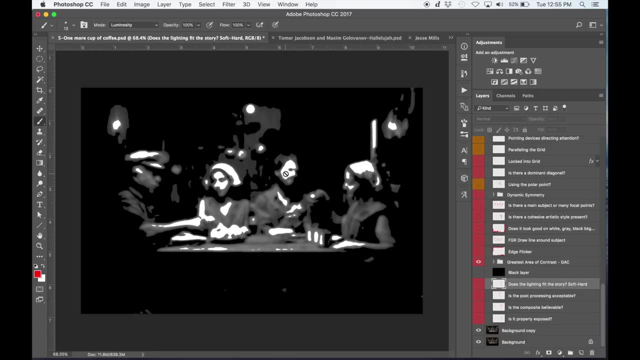 is the coffee being poured and stuff. But the way I see it is, I see her as the main subject, So the greatest area of contrast is where she is. This man's face is well lit against the dark background, but we still have a figure-to-ground relationship. 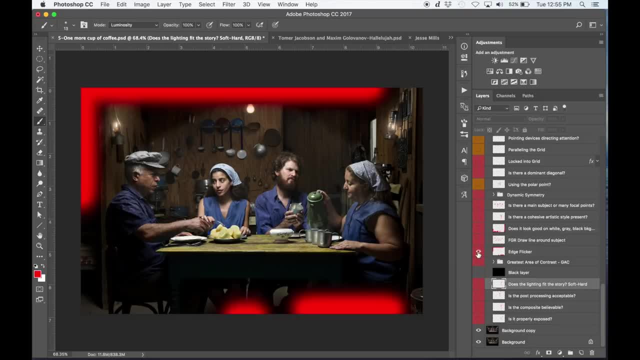 with this right side here And we'll get to that. in a sec Edge flicker Are there high contrasting areas near the edge. Everywhere where there's not red, there's a lot of contrast which can draw the viewer's attention. 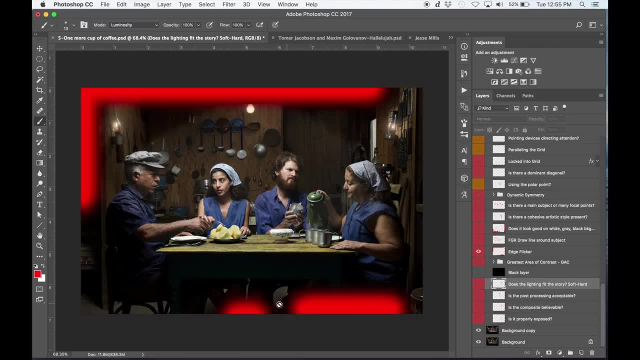 So this edge flicker is not as good as it could be. You could darken this, these areas, and then this area should be lit. but there's some reflecting metal, which is okay to have. reflecting metal. It shows the texture and things like that. 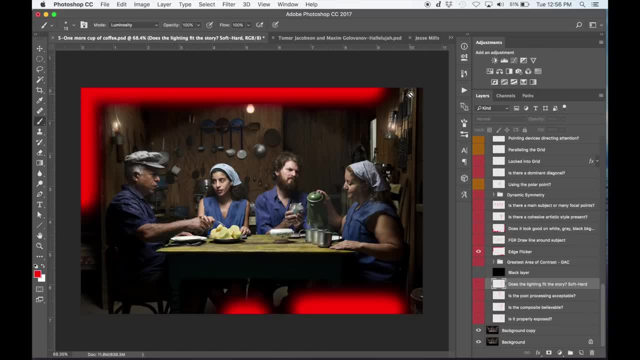 but it's right near the edge, So I would subdue that because it's not serving a purpose. I would just clone in some darker colors or paintbrush some black, And then this reflection on the table here is right on the edge. You could just get rid of that. 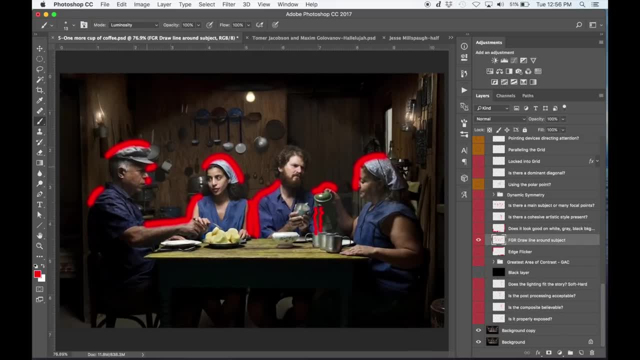 and no one would miss it. So figure-ground relationship is kind of suffering on this man's face. If we draw a line around the guy's head we see quite a few places reducing contrast, which makes it hard for the mind to see clearly what's going on. 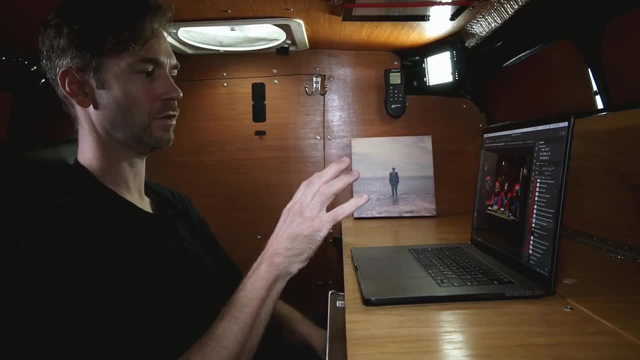 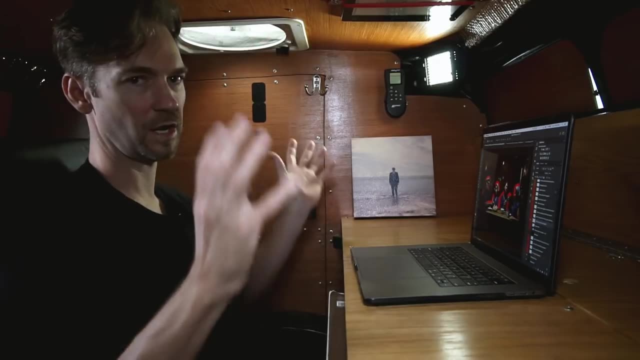 One thing: if you're trying to implement figure-ground relationship and you don't have a lot of area to work with, you need to find the pocket, and I teach this. Sometimes you can fit the subject in a large area, which is a large pocket. 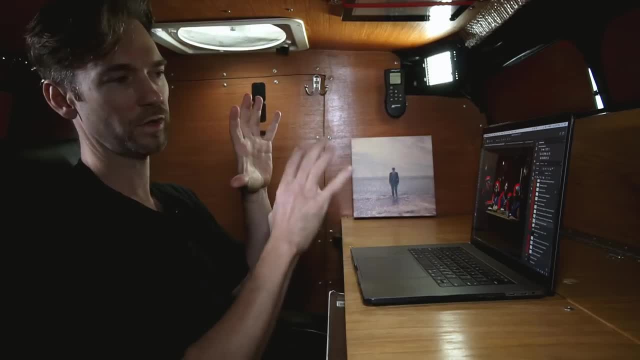 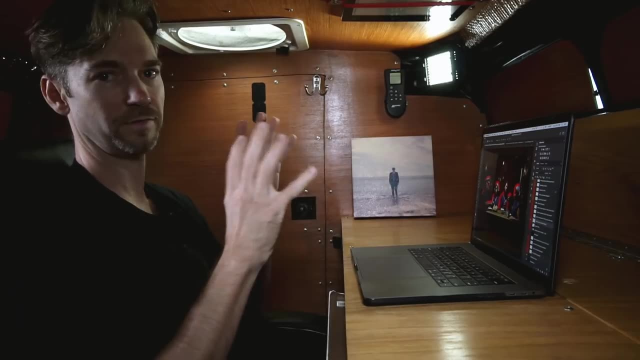 but other times you have to squeeze them into a smaller pocket where there's sufficient contrast. And the area you should focus on the most is the head, and if you can't even get the head in good figure-ground relationship, you have to work with the features. 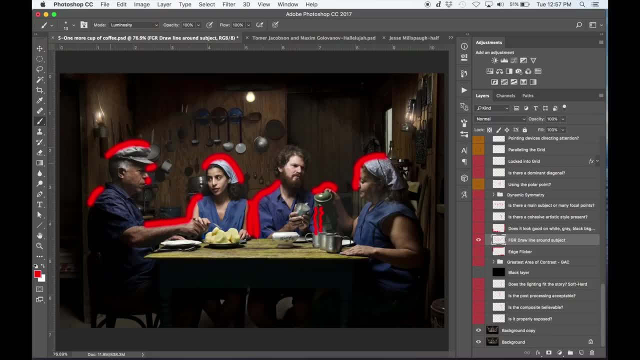 and mainly the eyes. So you always got to look at the way the head is fitting into the background. and his head's fitting into the background, kind of slamming into the props that you have in the background. Unfortunately, Same with her head and then his head is missing. contrast completely. 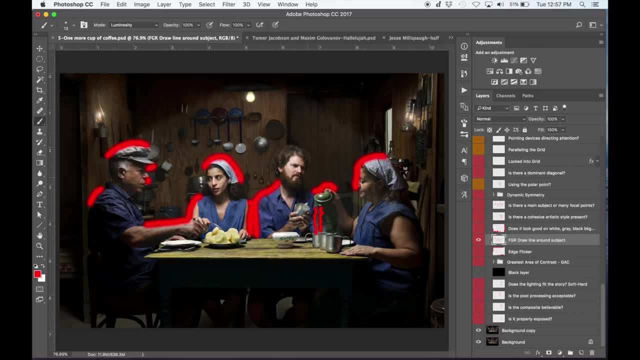 because he's got dark hair on the dark background and then dark beard on the dark background. So all we see is this chunk of his face And then her head kind of collides with the background. props as well, and I understand this is just the lighting. 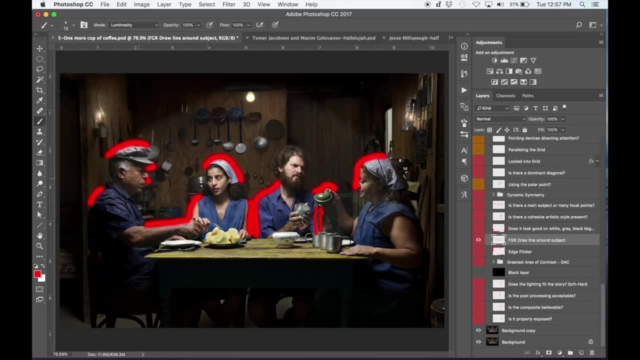 fading away, which is nice. but we got to make sure all these people's heads have nice figure-ground relationship. and then we start with their body. see if their body has figure-ground relationship. So we want them to stand out and be noticeable as an important part of the composition. 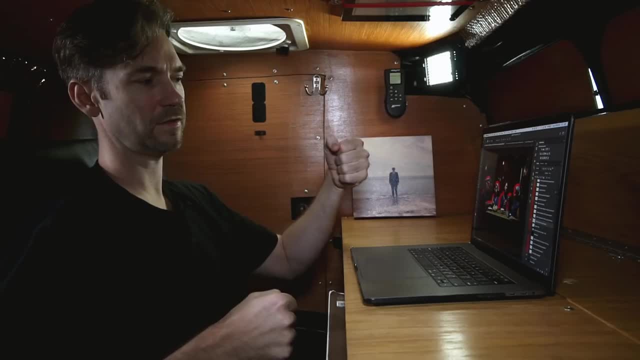 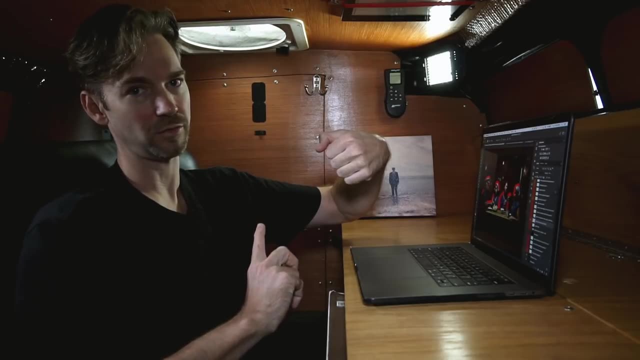 Even the coffee being poured. she's holding it like this towards the camera, but if you were to tilt it just a little bit, we'd see the spout coming this way and the coffee being clearly poured into the glass. but it's competing with the contrast of the coffee pot. 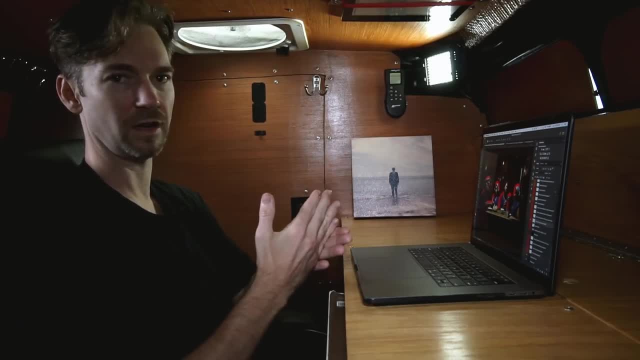 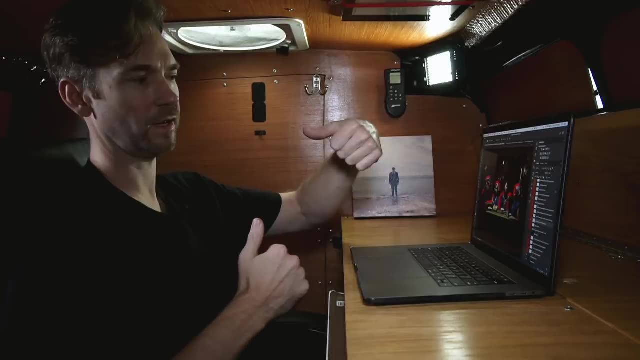 You've got the dark liquid on the dark shadows of the coffee pot so it doesn't stand out as much. But if you turned it to the side to show an aspect of you, we would see that clearly being poured in there. So to adjust that. 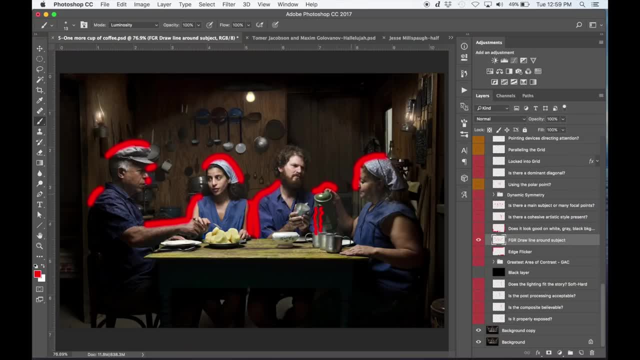 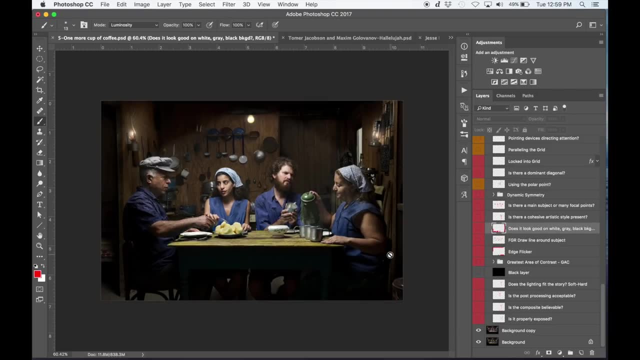 you can just dodge and burn a little bit, keep your adjustments subtle and improve the figure-ground relationship with everybody and the props. Does it look good on black and white? Like I said, those areas around the edge really pop out when you put it in a black. 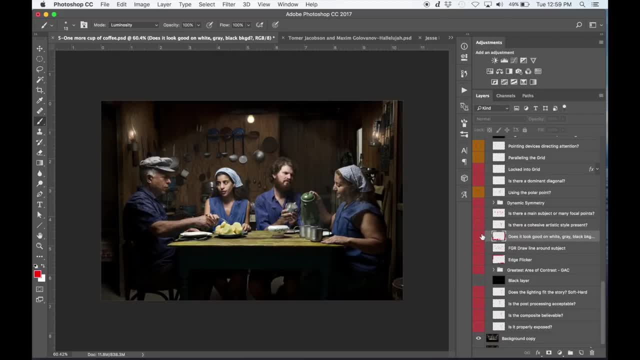 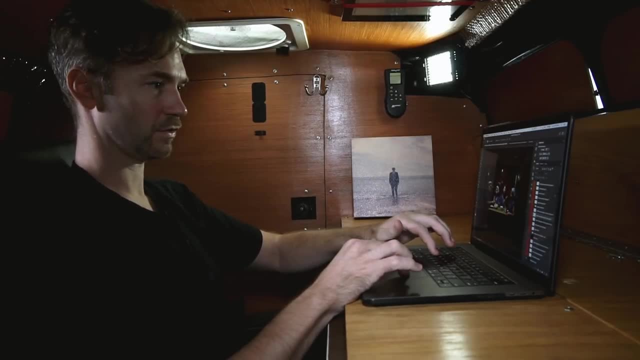 You can see how much attention they grab, and so those areas aren't even needed really to tell your story clearly. Is there an artistic style present? Yes, you have strong artistic style amongst all these photos that you submitted. So good job on that. 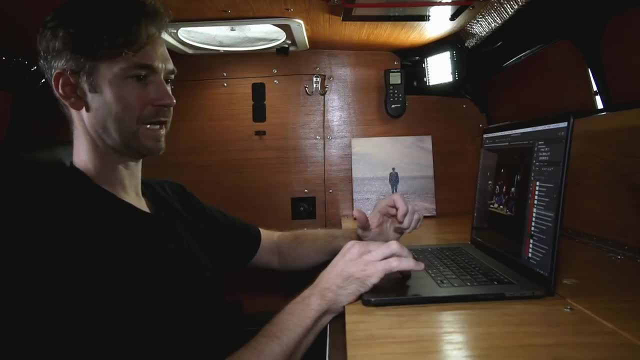 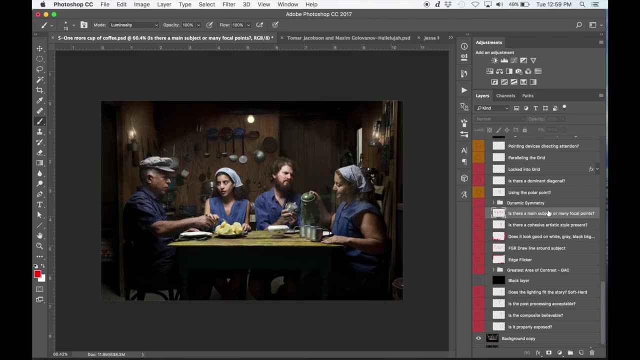 That's usually a hard thing to do and it's usually lacking in a lot of beginner photographers, So we can already tell that you're developing your style pretty well. Is there a main subject or many focal points, Like I said this lady? 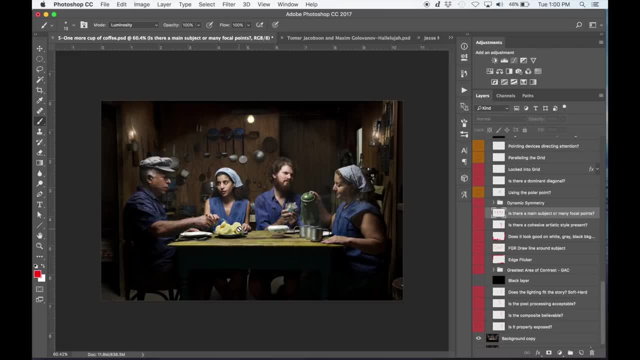 is the main focal point for me, and it's because she's the brightest and we see her face the most. These are side profiles. His face is partially lit, and then we have this big plate of potatoes, which creates a lot of contrast there as well. 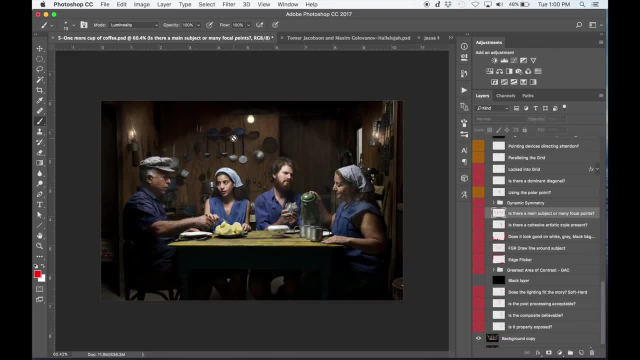 And then we'll get into the design which we see these ladles pointing towards her also. You got a main focal point here- It's probably not the one that you were hoping for- which is the coffee pourer and the guy begging for a cup of coffee. 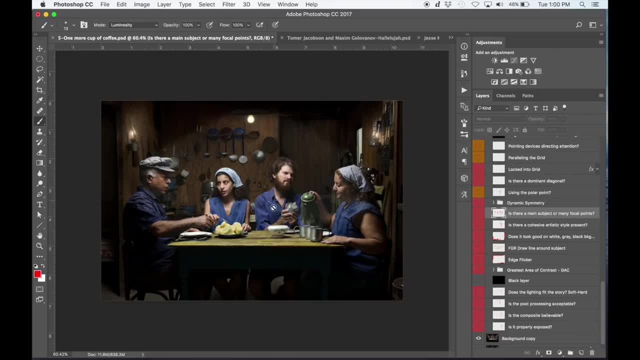 If you wanted to direct attention towards this, if this was your main subject, you could have had her looking towards it and then his eyes maybe lit a little bit better and looking over there as well. As far as pointing direction towards this subject, 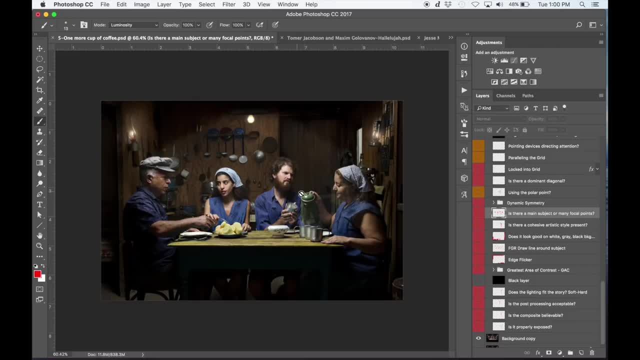 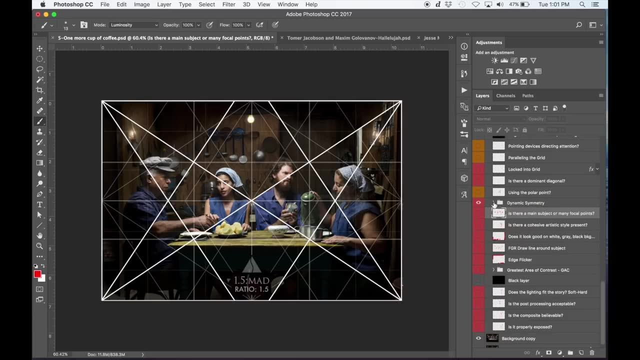 if that was your main subject, I would have her looking towards it as well, and that would help the viewer determine what the main subject was. Okay, let's look at the dynamic symmetry. Looks like you used the 1.5 ratio of your camera. 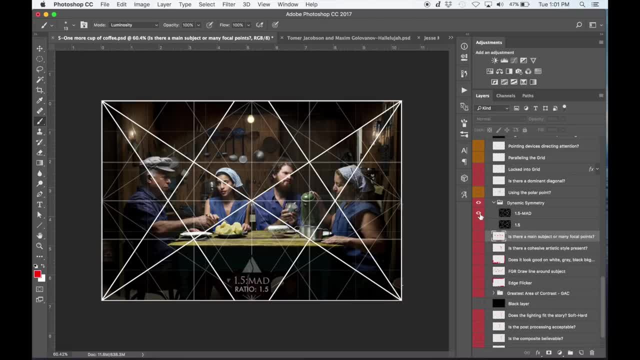 which is good. and now to see if you used the dynamic symmetry grid to compose your image. we have to look for dominant diagonals, and the only dominant diagonal I see is her arm, this lady's arm, but the figure-ground relationship is so bad. 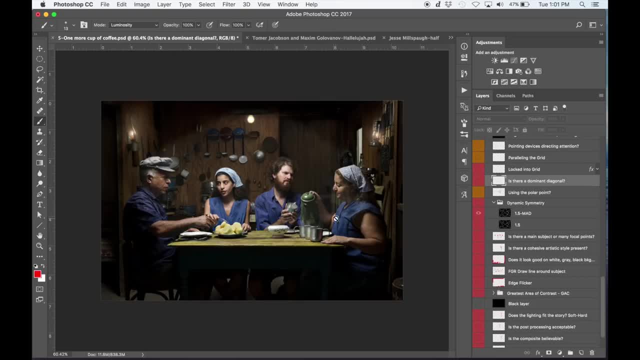 that we can't really see the dynamic movement that that diagonal creates. It's a sinister diagonal, but it's so lost with the background that we can't really see it as part of the whole image. It doesn't affect the whole image, as it should. 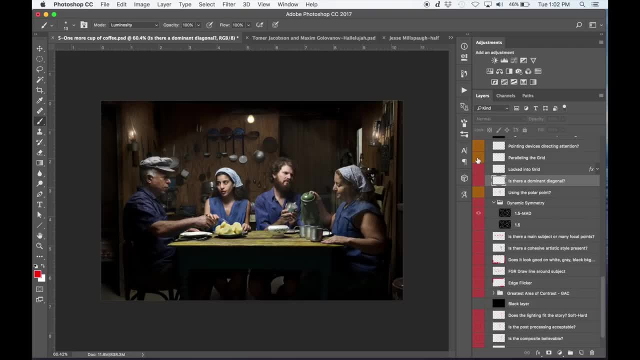 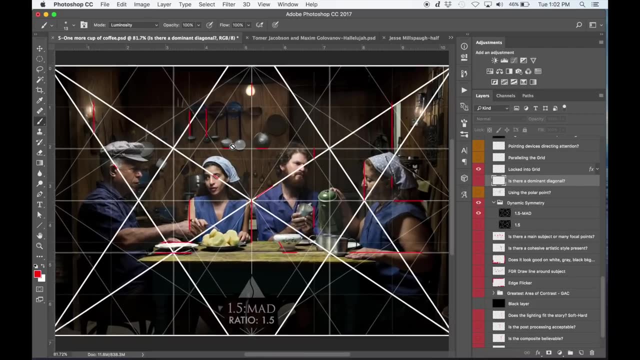 We need more dominant diagonals, more diagonals repeating in this. If you were to compose it with the grid in mind, that's what we'd like to see Locked into the grid. we have quite a few things locking in. You can see these ladles locking in. 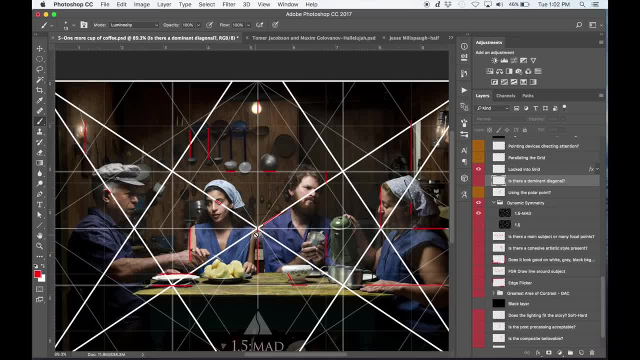 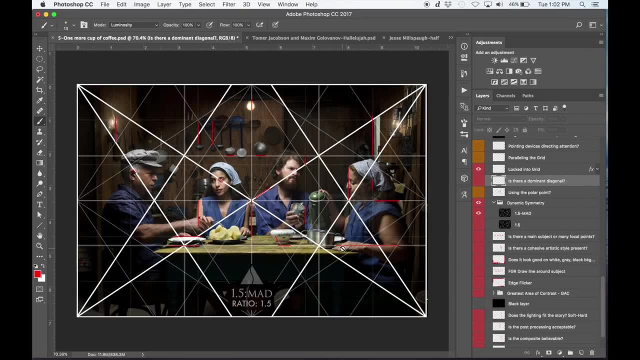 the lantern, her arm, her eye, her other arm, this guy's shoulder, these ladles, the edge of his head, this lady's face, the doorway in the background and her arm. A lot of things locking in, but not very many diagonals. 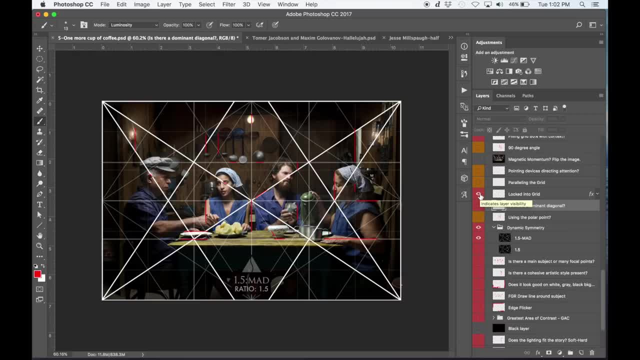 which is one of the main reasons we use the grid, is to incorporate more diagonals, So do we have paralleling the grid? We have a couple areas that are paralleling the grid, which is good Pointing devices, like I said. 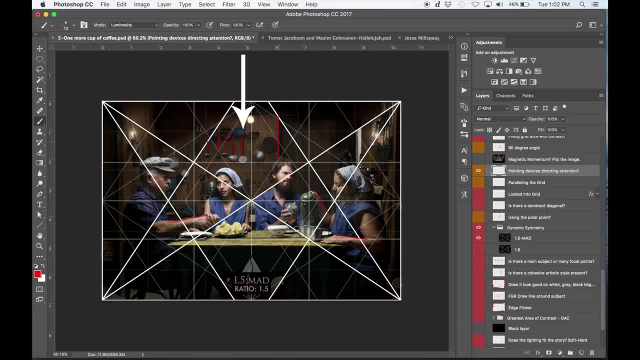 these ladles all point to this lady. The edge of the wall here points to this guy. Her arm is a pointing device, his arm is, and her other arm is a pointing device. So all these have the potential to direct attention to different elements. 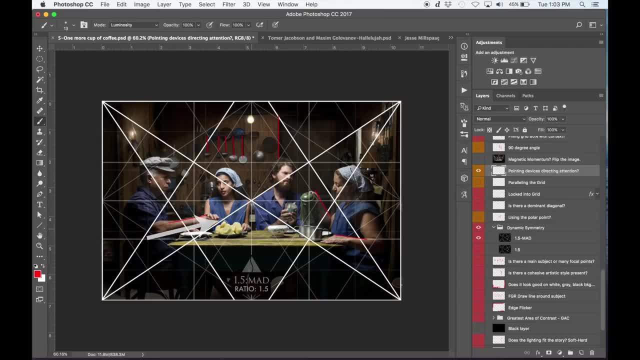 So this guy's arm draws more attention to the potatoes on the plate- Magnetic momentum. let me turn this off. We'll flip it, see if the movement's changed a little bit. Like I said, there's not a lot of diagonals. 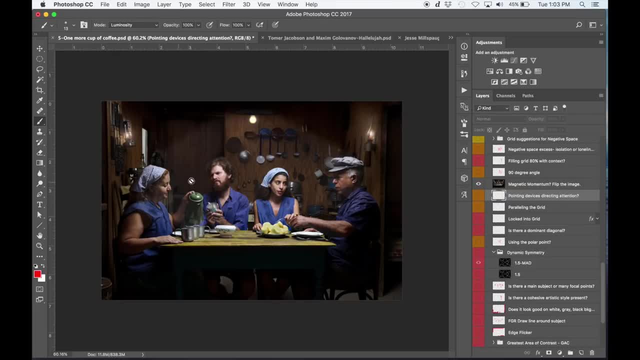 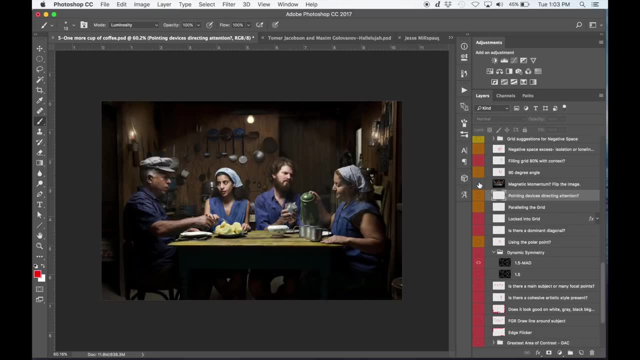 and all of the contrast seems to be with the heads and all the focal points seem to be amongst the heads. so there's nothing really on a dominant diagonal and we don't see any different movement. so that's cool. Is he filling the grid with 80% of context? 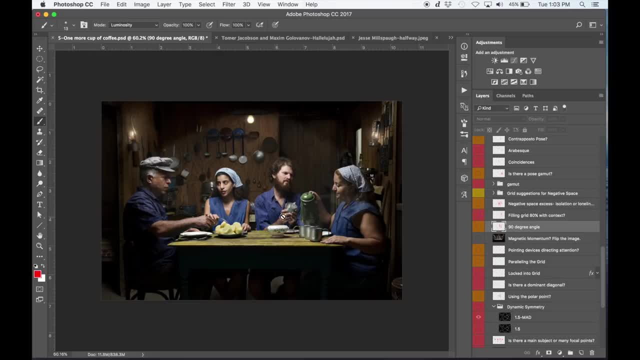 Yes, you did a very good job of filling the grid, although when we look at the background, we're gonna see that there's quite a bit of distractions from your props. Is there a gamut? Yes, we've got a couple repeating diagonals. 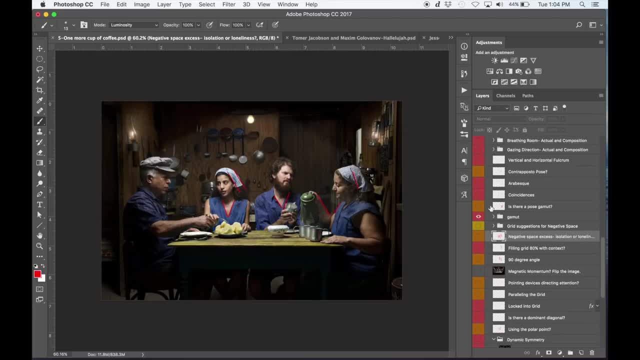 in the shirts and the hair pieces, but nothing prominent and nothing tying the foreground with the background. If you had something diagonal back here that was equal to this diagonal, we'd get a little bit more unity, and if you followed it across the form. 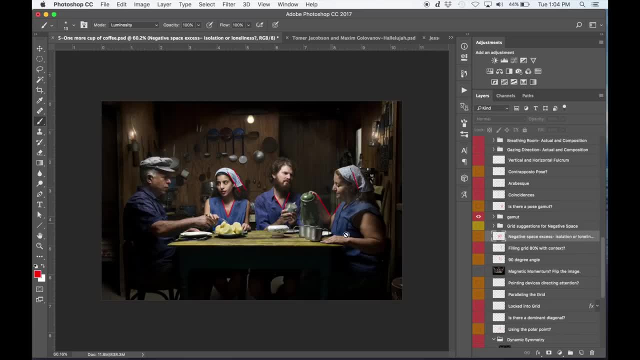 like with this guy's arm or the lantern here, things like that. we'd get a little bit more movement, unity and rhythm across the composition. So we've got a few coincidences. All of these lines from the ladles create a movement downwards. 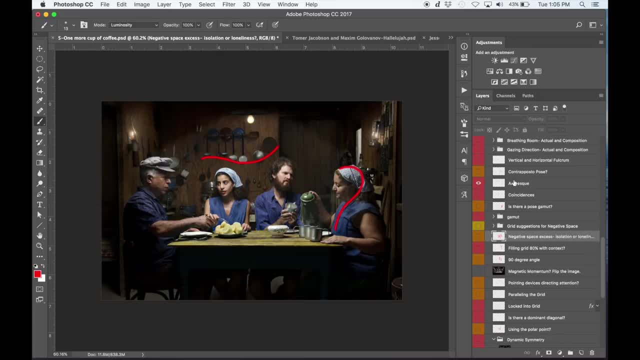 and actually some of them coincide with the woman's arms, which is cool. The arabesques: we've got a couple hidden arabesques. One of them I liked was this one that's sweeping around the ladles and going up and then kind of coming down this way. 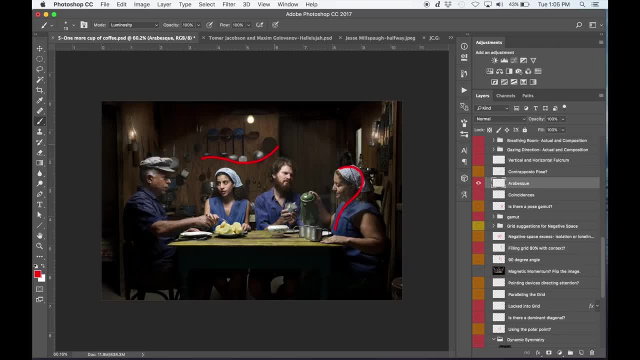 so that's a nice movement you've got there. It'd make it even better if it were being united with the characters. Maybe his face was right here and then his arm swung around here. We'd have a nice arabesque sweeping around. 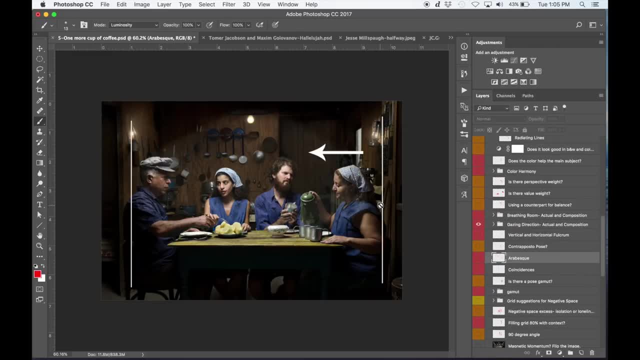 and there'd be more unity there. Gazing direction: if we measure the bulk of the image and we look at the negative space on each side, we see that the gazing direction is going from right to left, which is fine. It's almost a centered composition. again. 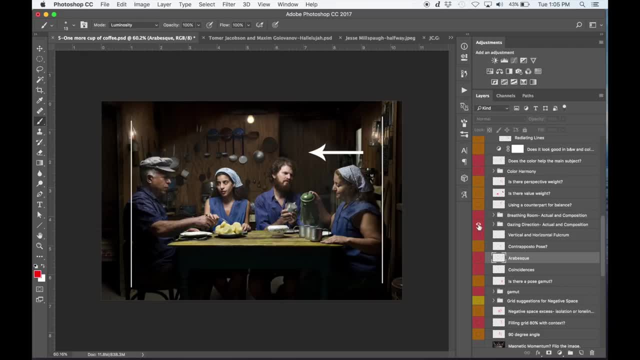 which works just fine because you're balancing from left to right very well- The breathing room. if we take the bulk of this and look at the negative space, we see that there's a little bit more area on top, On the top here. 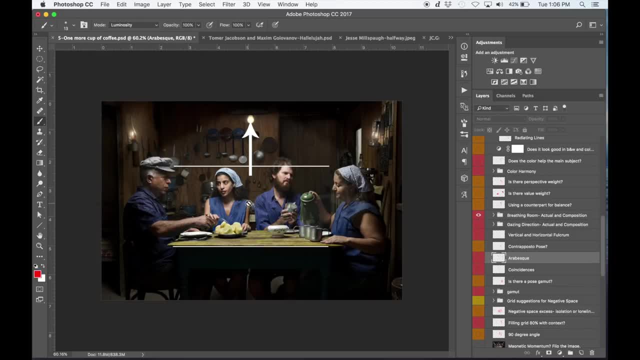 a little bit more negative space. so we see that the balance is good from bottom to top. So there's a lot of value weight added here with the plate of potatoes, like mentioned before, and then her hair piece up here because it's light up against a really dark area. 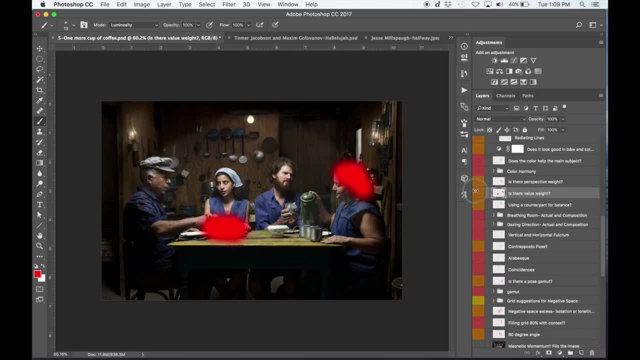 so we've got a lot of value weight, but they tend to balance each other a little bit from left to right. If we're looking at the horizontal and vertical center lines, we can see that they're both on opposite sides of the center line here. 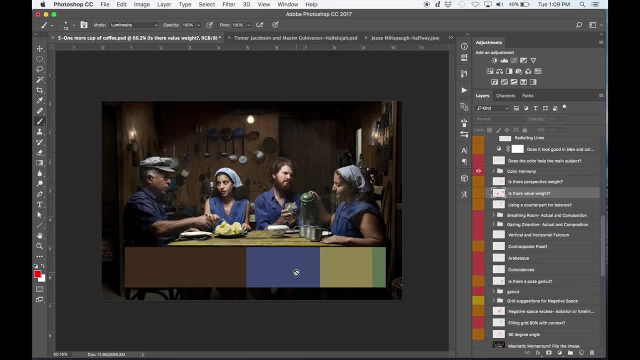 the fulcrums. Color harmony: like I said, we need red, yellow, blue and green for nice color harmony. Here we have the neutral brown and the blue obviously is main color of this- yellow and then a little bit of green seen here. 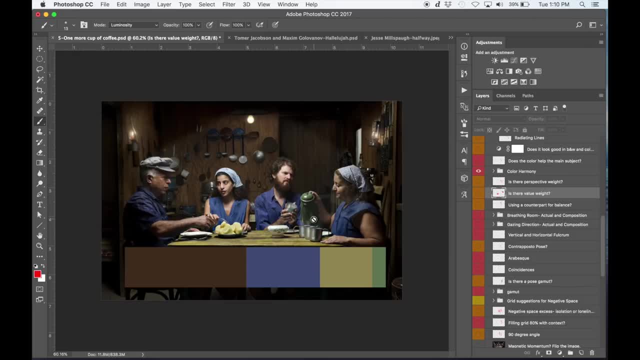 You could have enhanced the color of this a little bit better, maybe to choose a layer, set it to the color blending mode and then color it in some green and then adjust the opacity just to make it pop out a little bit more, since that's the one that's singing. 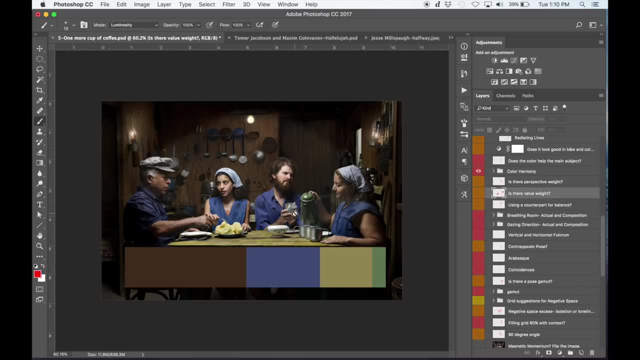 and that's where your main subject is, supposedly with the coffee. And another thing you could have done to add more color to it is select red potatoes instead of the white potatoes, and that might have added a little bit more color to give you the color harmony. 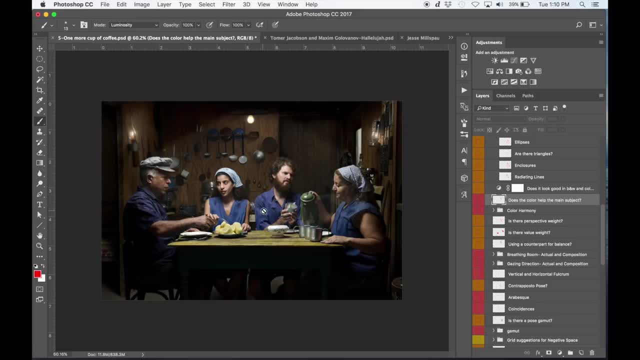 Does the color help the main subject? Yes, Like I said, blue has a certain emotion attached to it, and then green does too, And then, since green is the least amount of color, it's gonna be attracting the most attention right here. 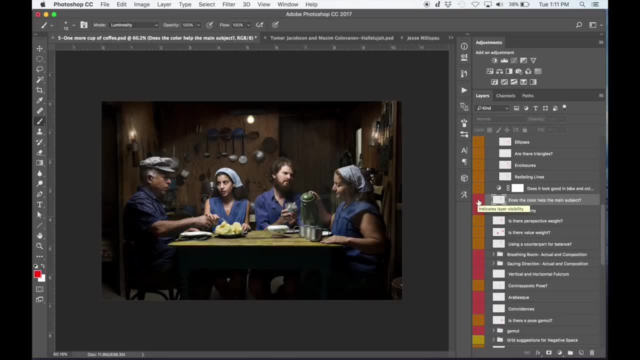 So that's good, that the smallest amount of color is right where you're wanting the main subject to be. Okay, does it look good? black and white? Yep, looks great. black and white too. Triangles: there's a little bit of a triangle here. 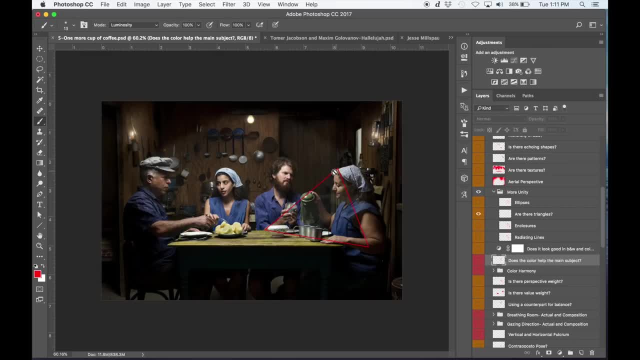 You can see the movement from her head. There's a diagonal coming down and created here with these coincidences, and then this and then going up her arm and the edge of her head, So there's a little bit of a triangular enclosure there. 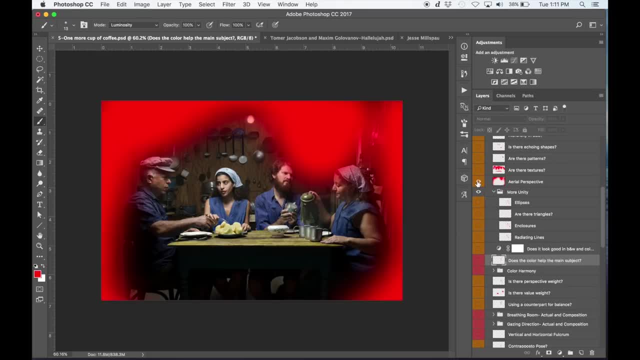 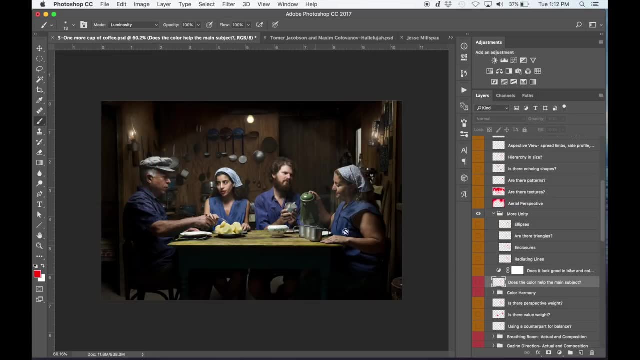 Aerial perspective: yes, The way you lit it was good to create some depth and atmosphere in there. Are there textures? Yes, You've got nice wooden wall textures and then the table is a texture also. Are there patterns? Yes, 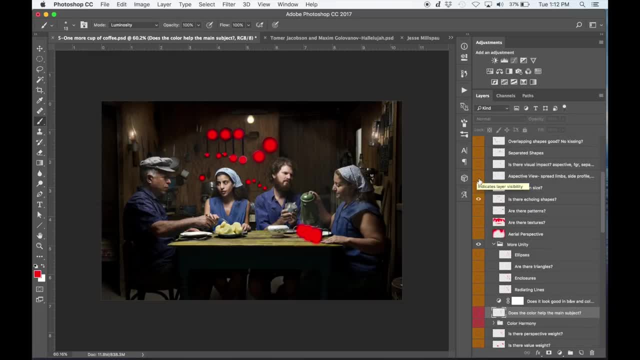 She's got a little pattern on her head. You have echoing shapes- yes, You've got all these circular shapes on the wall, and then you've got the repeating shapes on the table as well. We have an aspect of view. yes, 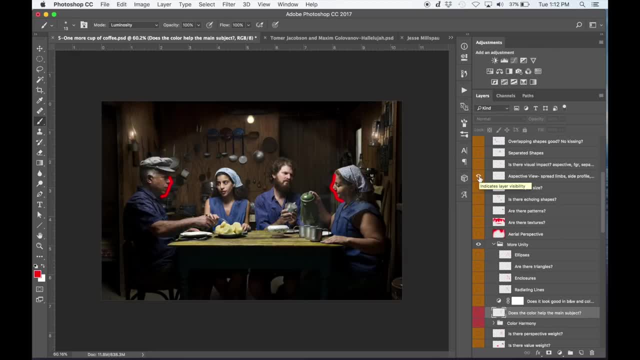 but, like I said, the figure-ground relationship is negatively affected by what's behind there, so that affects the aspect of view. So side profile of the face helps us identify the person's face a lot better with minimal information, but it also has to be combined. 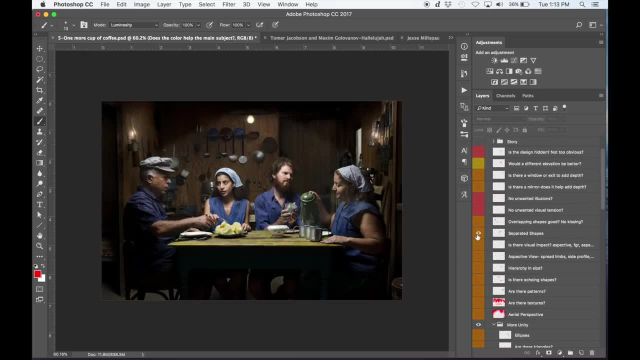 with figure-ground relationship. Separated shapes: this guy's got a separated shape but also the figure-ground relationship is affected there, not creating clear separation. Overlapping shapes: I've got a couple things overlapping poorly, Unfortunately, if we look at the potatoes and her hand. 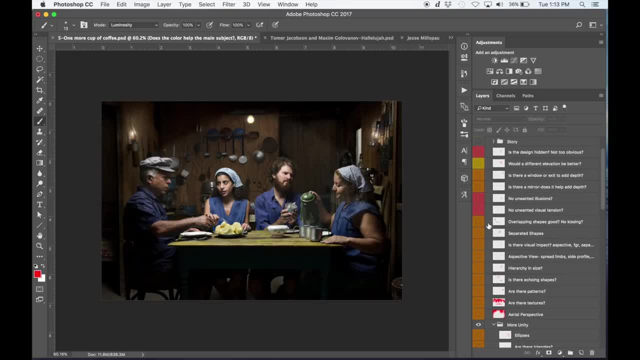 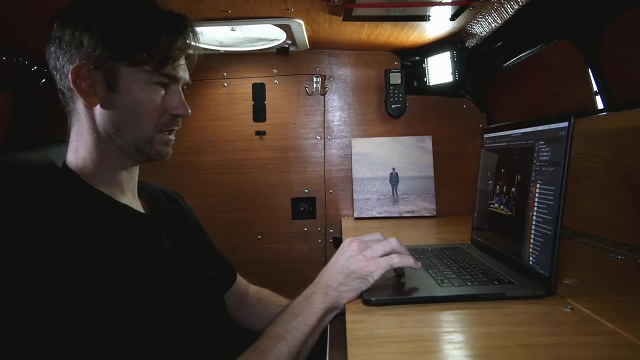 it's almost kissing. We want to avoid kissing, which is where two edges meet and it's hard to determine what's going on. Sometimes it creates an illusion that's unwanted, and sometimes it doesn't allow us to determine what the foreground and background is. 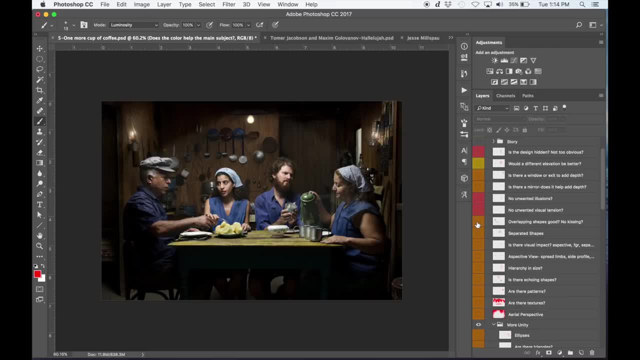 what's in front of the other. So we don't want to cause any visual confusion. We want to make sure everything's as clear as possible, and the way this guy's doing it- his hat- coincides with the light shape of this pot in the background. 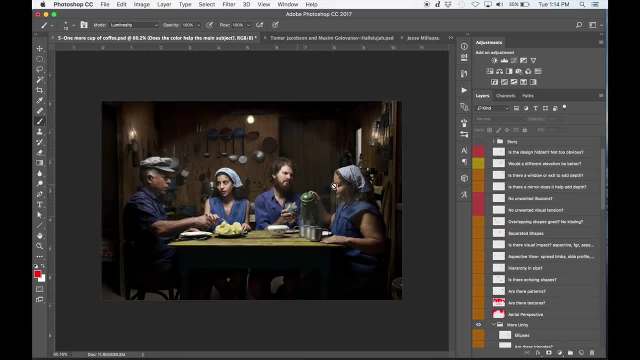 and then his face coincides with the background as well. All these things can be cleaned up to clarify the visual message. That's the unwanted tension, Also with the plate being placed kind of through the handle and then through the handle. here kind of just creates some shapes. 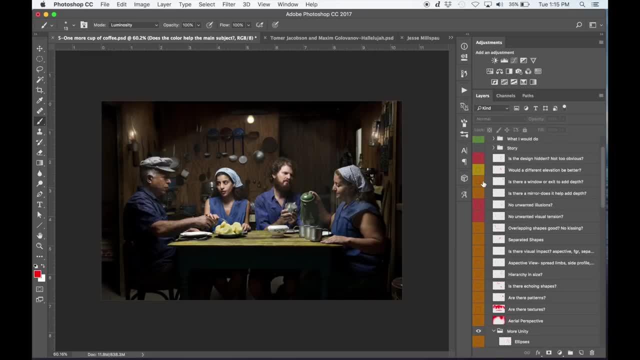 that draw a little bit of attention that's unwanted. Is there a window for an exit? Yes, you have a little bit of an exit to add depth. What I mean by window for an exit is just if you look at a lot of master paintings. 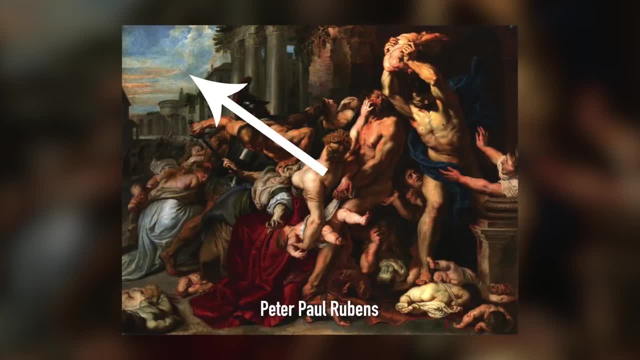 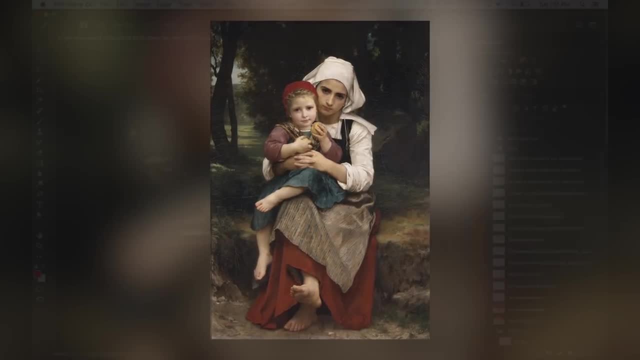 you'll see that there's an area in a forest or something like that. that creates a place where the eye can travel to and come back to. It just adds a little bit of depth. But this one is just a sliver. It doesn't really show the outdoors or anything like that. 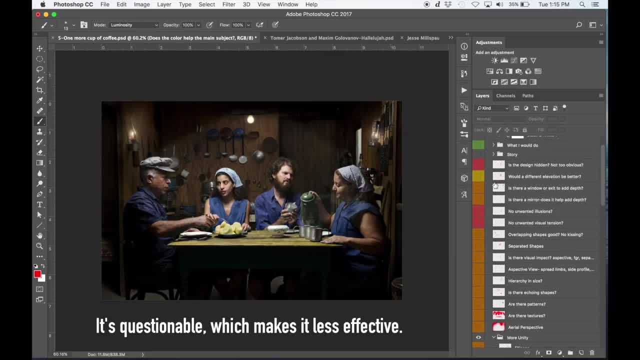 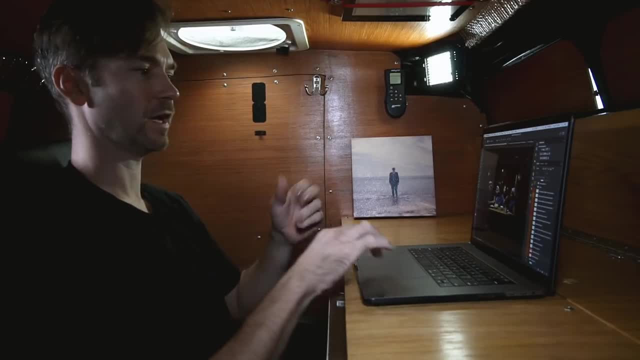 so it's not as effective as it could be. If he showed maybe the whole window on this wall here and then he showed like a forest or something, that would add to the story Right here it doesn't really add to the story. 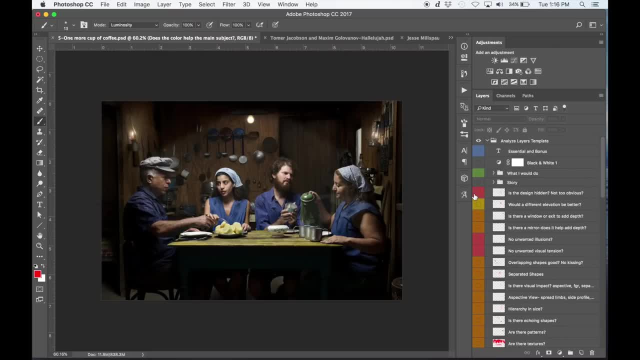 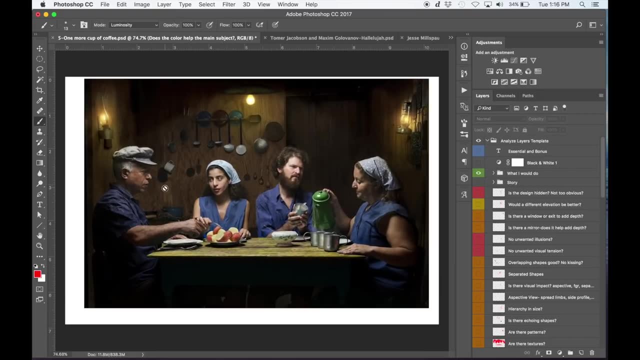 so it doesn't have to really be there. Is the design hidden? Yes, most of your design techniques are hidden, which is good, Okay. so what would I do? I would simplify the background. So what I did was photoshopped all this stuff. 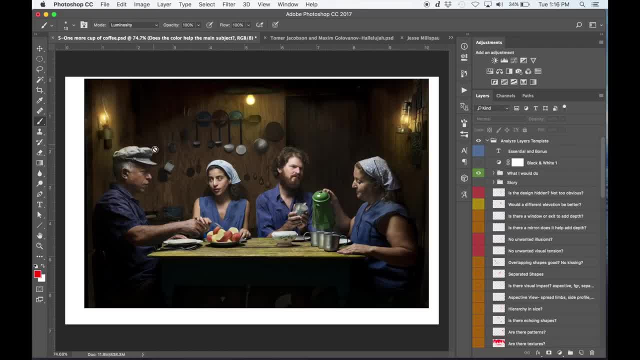 the clutter, the props. The props were cool and the props were nice, but they really interfered with the main subject and we have to give priority to the main subjects first and then add the props in afterwards. They have to fit in as a whole. 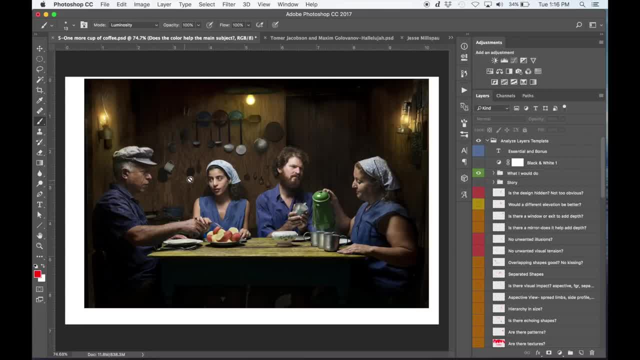 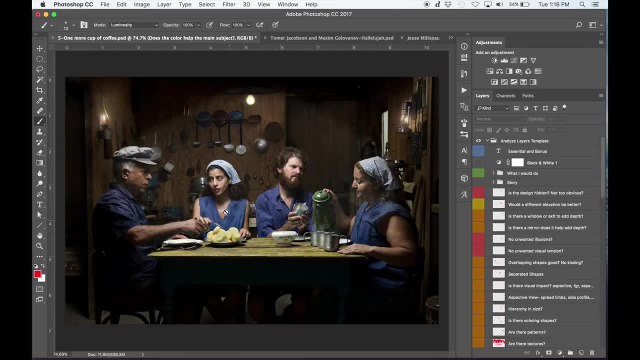 as a team working together instead of fighting for attention. So I cleaned up the background quite a bit around each subject. I'm going to flick this on and off. You can see the pots around this girl all disappeared. This guy, even this woman. I got rid of all that. 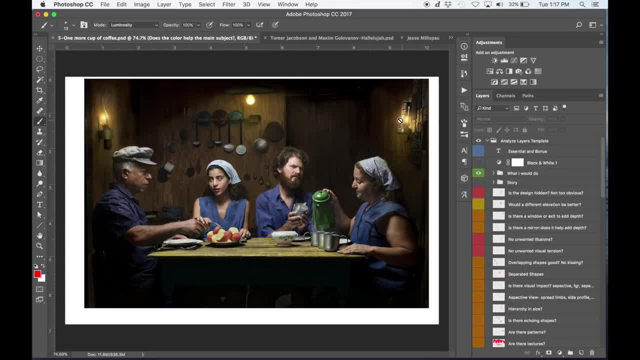 Got rid of the window because it wasn't adding. I added a little bit more glow to the lanterns, cropped it in a little bit, got rid of the high contrast near the edge and then subdued this area on the bottom here And then I brightened some of their eyes. 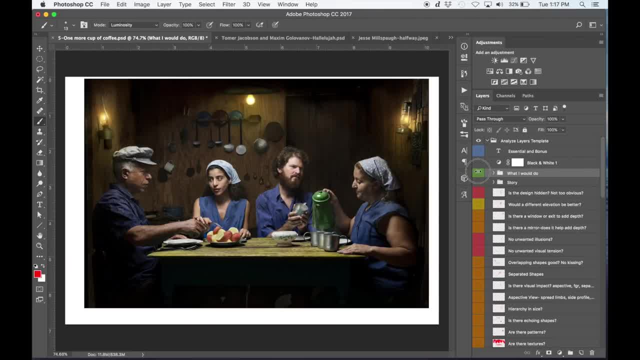 Her eyes, his eyes, his eyes. I brightened those. If you look close, I'll turn it on and off. you can see how their eyes are getting a little bit brighter. And then this guy's head. you can see. I tried to dodge and burn. 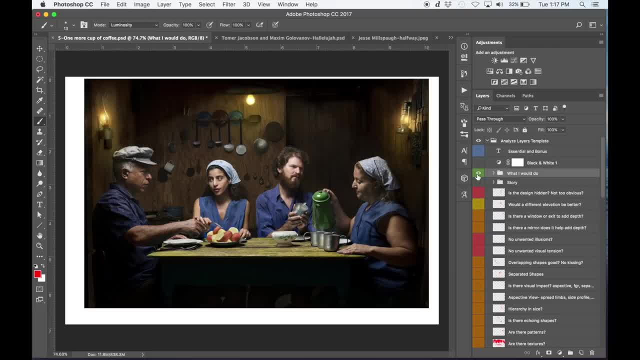 and improve the figure-ground relationship. So look at his head and see how I used simultaneous contrast to darken this, lighten this, lighten this, darken this and just go around, Not just make everything around his head bright. I made it according to the areas on his head. 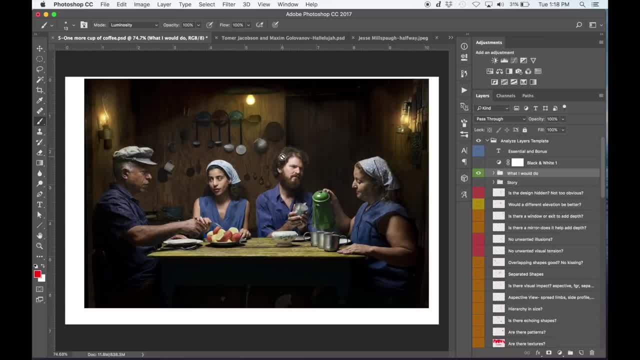 This area of his head is really light, so we want to darken this and lighten this. Over here is darker, so to make that work, we have to make this a little bit darker and this a little bit lighter, and that'll pop it out. 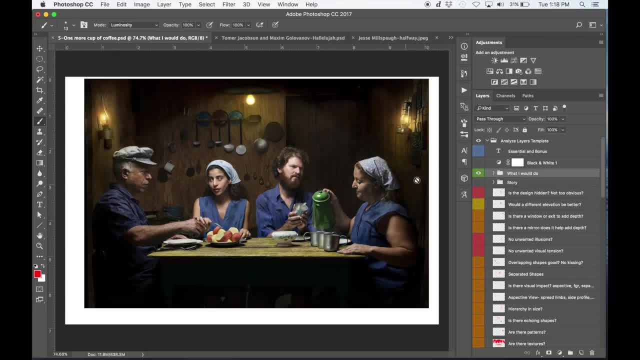 I increased the green on this. Like I said, I added a little bit more green to make that pop and draw the attention this way a little bit. I dodged and burned the cups so they would be separated a little bit more. You can see that. 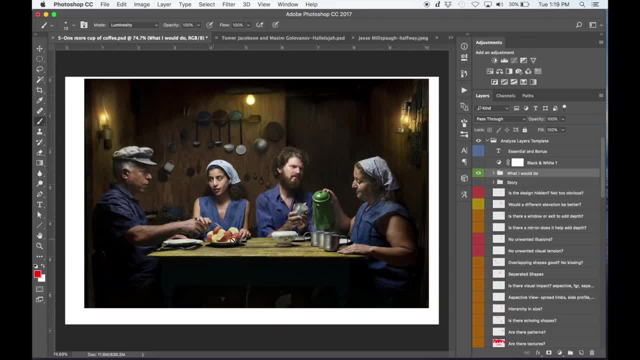 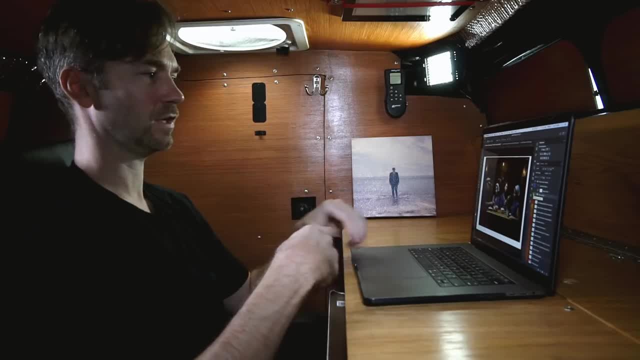 Subdued the bright whites of the plates and then added a little bit of color with red peeling on the potatoes to add a little bit more color. So all this is stuff I would do to tell the story in my head, but this might be completely different. 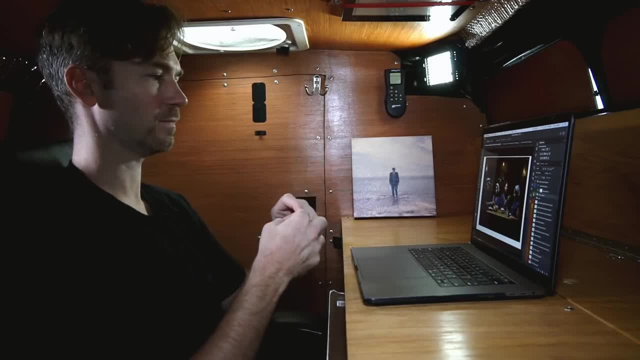 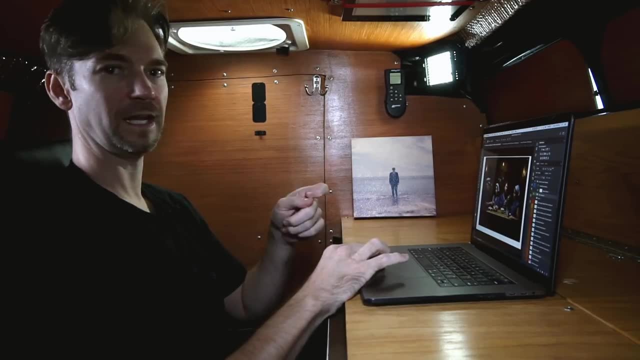 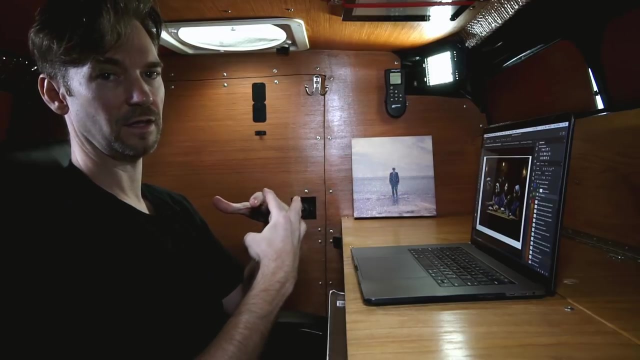 than what you're trying to present to your viewers. One other thing, before I move on to another photo, is that a lot of your photos had white in it, like the white plates, the white wardrobe, all that stuff, and that's always going to draw more light than maybe you want. 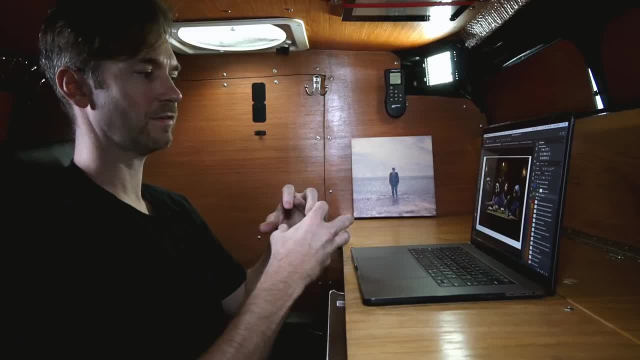 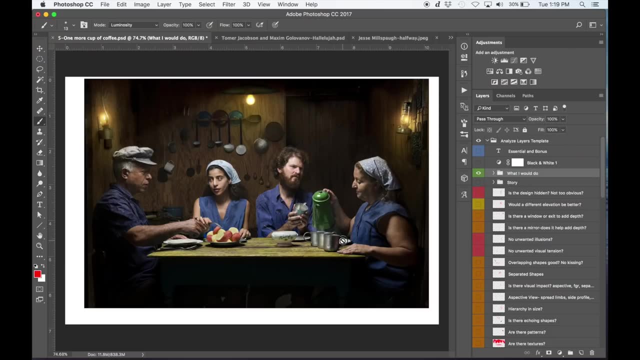 So if you want to be able to control the greatest area of contrast, look where you're adding white, because that's going to grab a lot of contrast and you may not want that. Like this area down here by the plate. that's grabbing contrast and you may not want that. 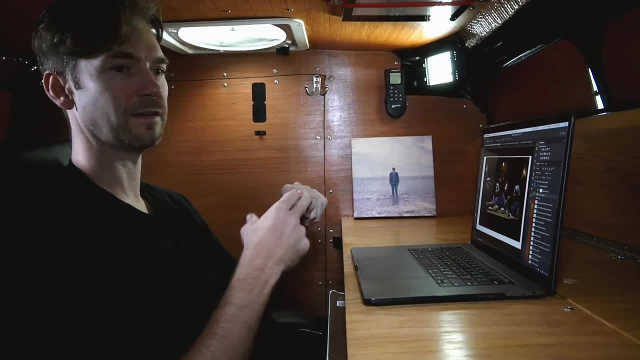 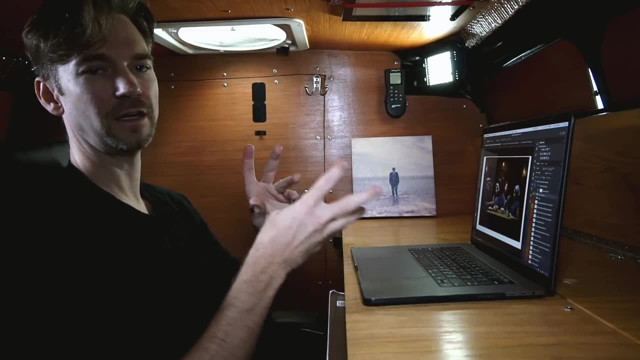 So you may have to choose different color of plates, like a neutral tan plate, or a different color to add to your color harmony. Just be aware of the light colors of your compositions, because that's what I saw in a lot of your photos is that's grabbing a lot of attention? 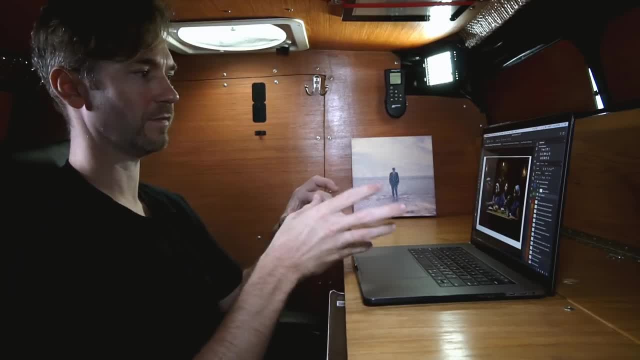 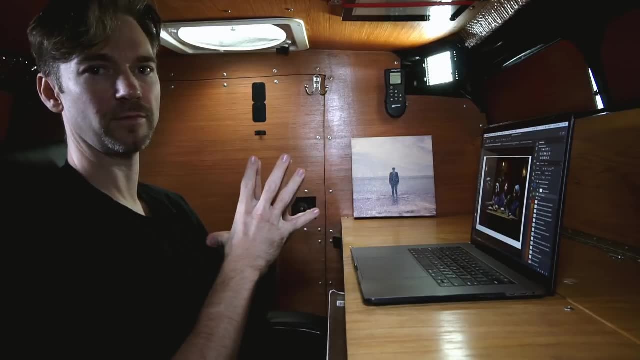 and it may not be where you're wanting that attention, So just be aware of that. But anyway, nice thanks for submitting that and good job overall. Just make some minor tweaks: learn a bit more about design and figure-ground relationship and use more of the grid. 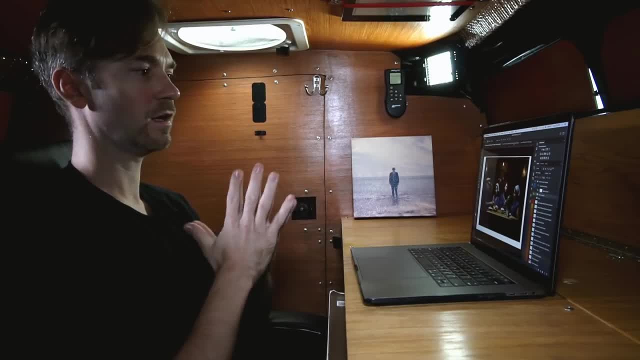 and try and implement color harmony, color hierarchy and balance and you'll be on your way. You're doing a very good job of lighting, You've got elaborate sets, You've got multiple characters and I know all this designing stuff. this stuff is tough at first. 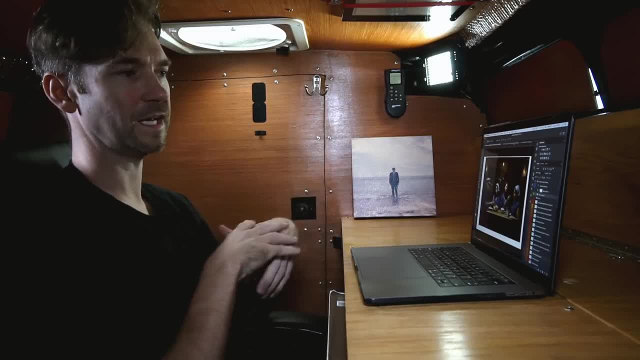 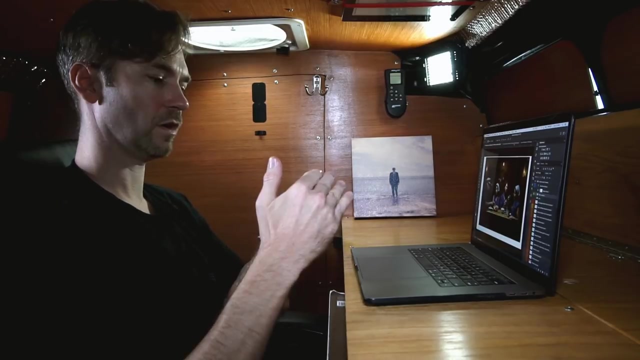 I find it frustrating to work by myself with lighting and multiple people. That stuff can be frustrating. but to reduce some of the frustration, just work out the design on your computer in a drawing or a sketch and be sure to implement it. Maybe bring a written-out plan. 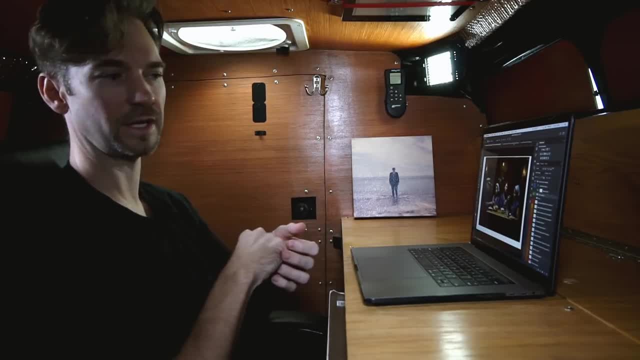 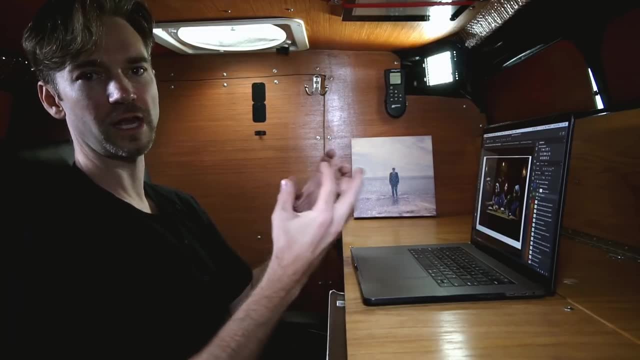 Be sure to include the arabesque. Look for the white material that's creating contrast, things like that. I know you're paying attention to your background, to incorporate the background as a cool element, but in some cases the background distracts from the main subject. 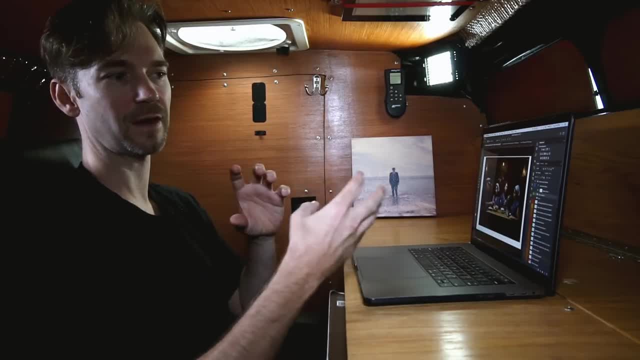 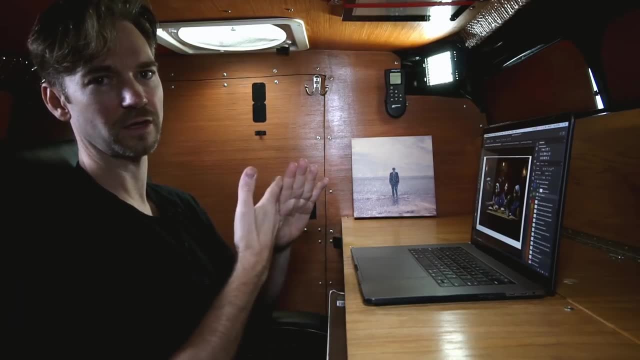 So always prioritize the main subject and how it fits into the background. and if the background has a lot of high contrasting areas, it's going to compete with the foreground subjects. So you just got to make sure you double-check that stuff and work it out in your head. 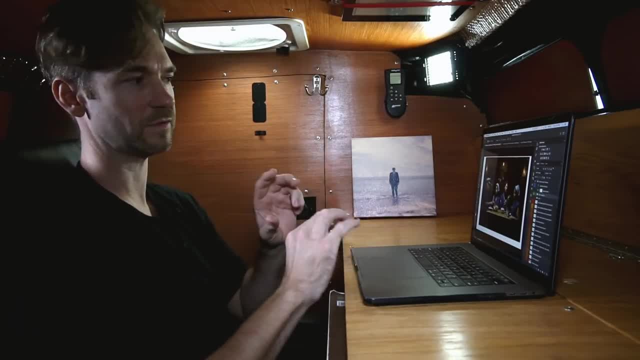 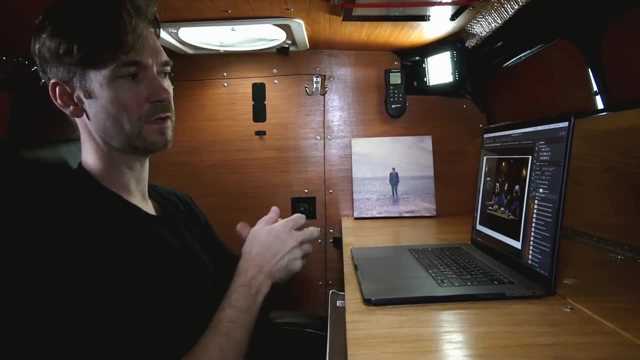 and look for the greatest area of contrast and figure-ground relationship and stuff. Make sure it all works together first before you go on set and capture, because you have some cool backgrounds but some of them compete, unfortunately, with the foreground subject, So just pay attention to that. 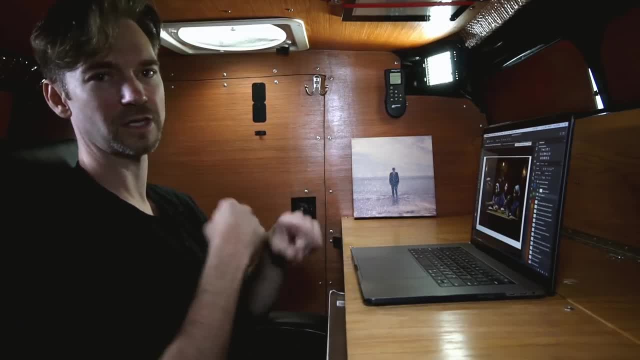 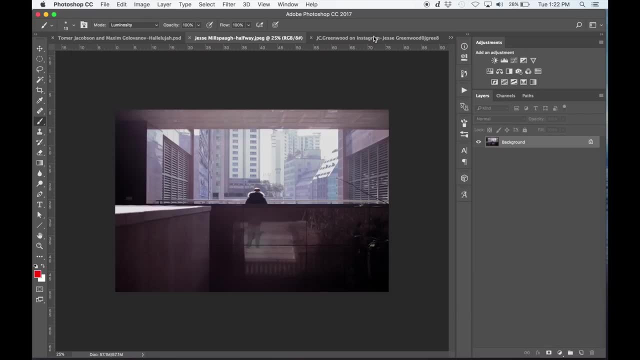 and keep doing what you're doing, because you're doing good, and just keep educating yourself on the design techniques and you'll be fine. All right, let's move on to the next person. I got a couple more that I have time for, and then I'm going to call it quits. 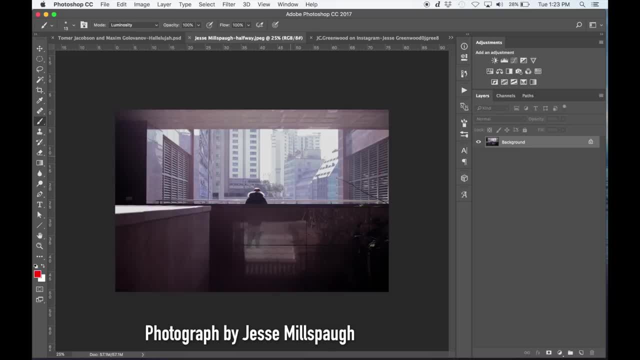 So this one is from Jesse Millspa, and I'm just going to run through these last two real quick, because they're considered street photos, because you're not able to implement as many design techniques as a fine art photo or a painting or anything like that. 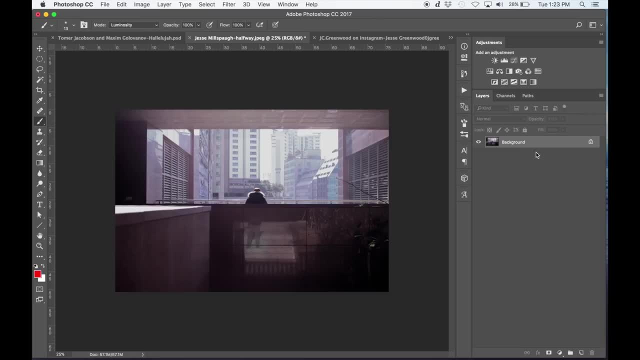 So I'm going to run through these. I'm just going to do the same auto color, like I did the previous images, and then I'm going to look at the design techniques. So this guy's pretty much centered and what Jesse's doing here is creating a coincidence. 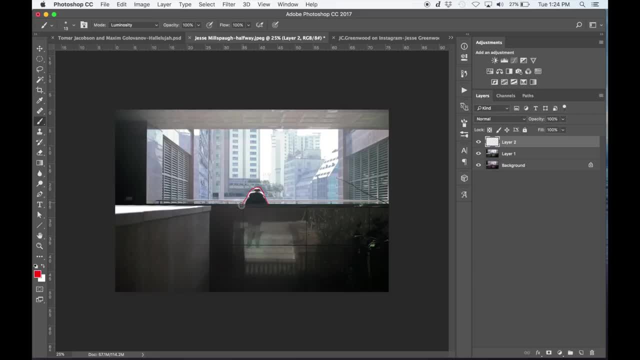 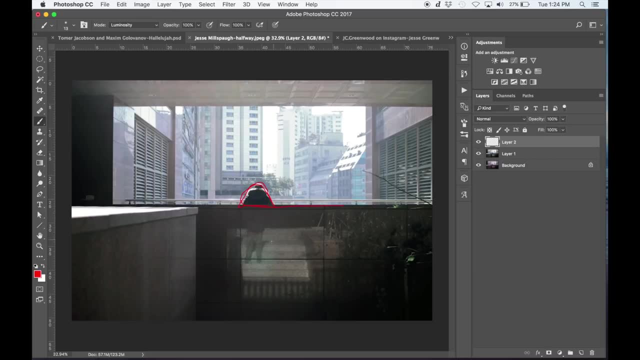 So this guy, he's creating an illusion. This is a surrealist image and he's got this guy, his body, on a different level. but here's Jesse in the reflection and he's lining it up with the guy's body. So he's creating an illusion. 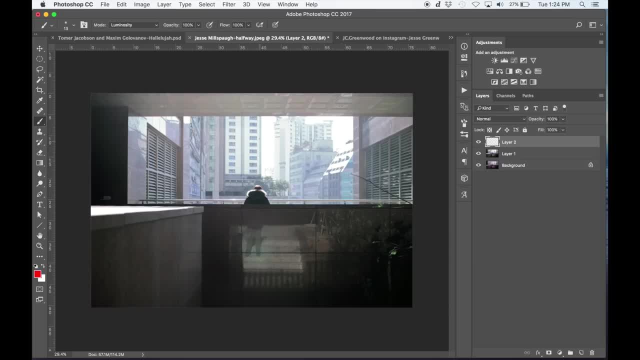 So that's pretty cool and you know it's nice and balanced. You've got a coincidence: going down here meeting the guy meeting your legs, all these repeating shapes, nice shapes here, subdued edges around the edges here, so there's not too much high contrast. 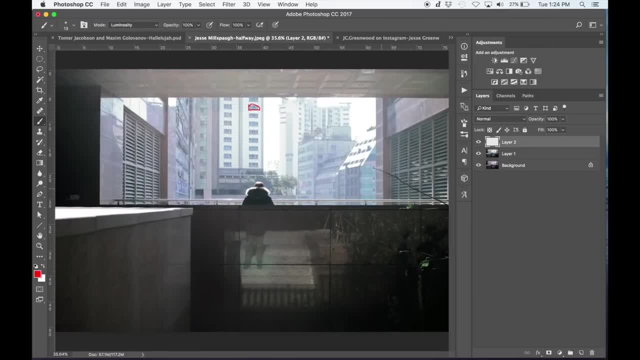 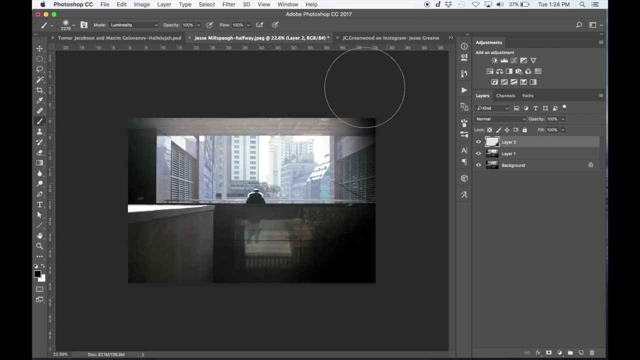 There's an area here that's high contrast, so what I would do maybe, is to subdue that a little bit and just draw in with some black and then maybe up here, subdue that a little bit and then reduce it to about 10%. Maybe you can add a little bit more down in this corner. 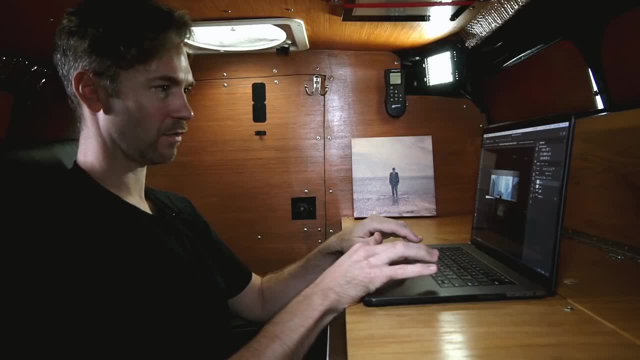 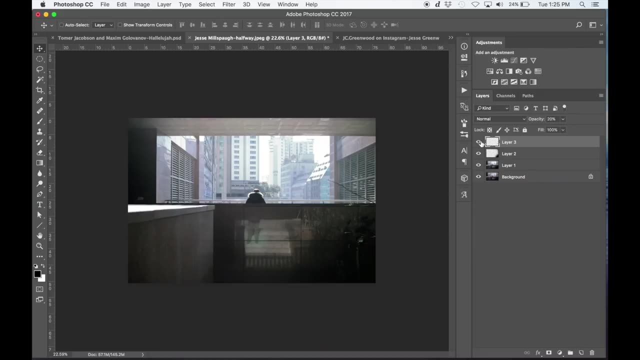 So with street photos, I don't like to edit anything out or manipulate it in any way, but I will use traditional darkroom techniques- dodging and burning of things- to subdue some of the contrast. And what else might have made this a little bit better. 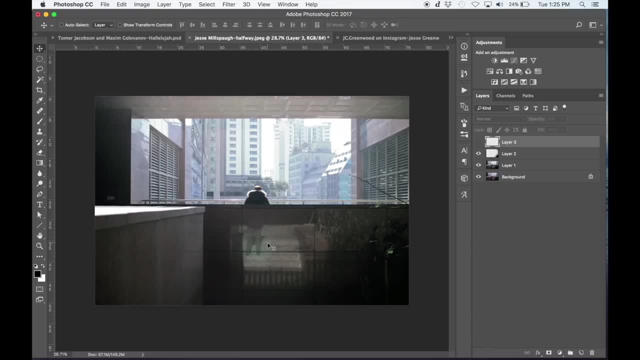 You can't really adjust it now, but if you positioned yourself to be more in the center, so if you were moved, maybe standing here, if you walked to the right a little bit more, you could position that guy in the center and that would help the balance a little bit more. 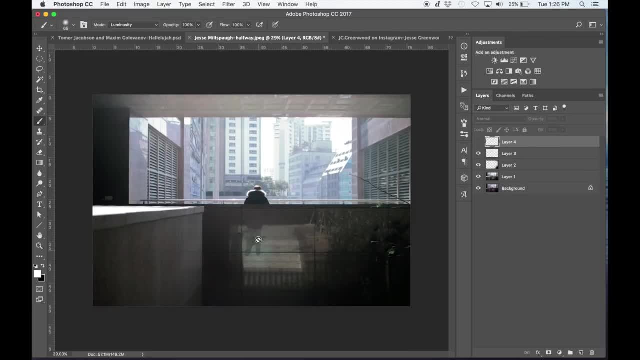 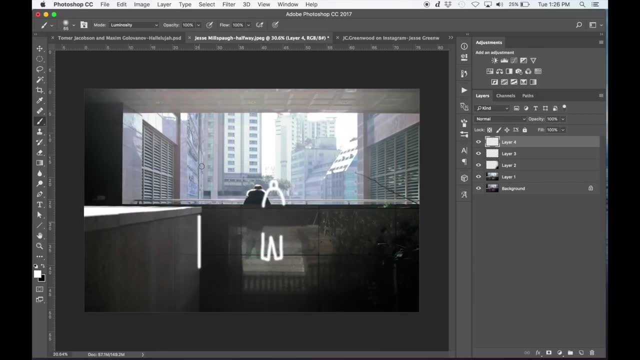 So far. I mean pretty cool image. You're incorporating coincidence, creating a surrealist image, creating balance. got a coincidence there, right here, run this up and it's coinciding with that. So another thing I wanted to point out is: 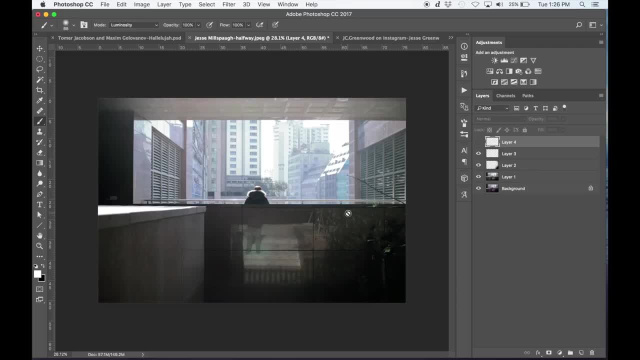 if we're looking at the color. sometimes, if images don't have that much color, then it's better just to convert them black and white, like I was talking about earlier. Unless it's film and you're shooting film, I wouldn't recommend converting color film to black and white. 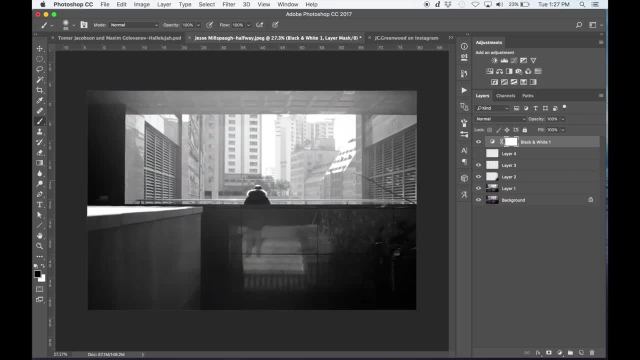 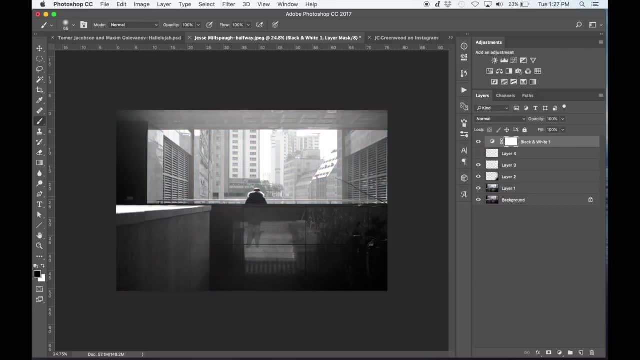 But in this case you could convert this to black and white and maybe clarify the story a little bit more. instead of like having minimal color that doesn't really help the image. You can convert it to black and white and increase that surreality, A lot of like images from Cartier-Bresson. 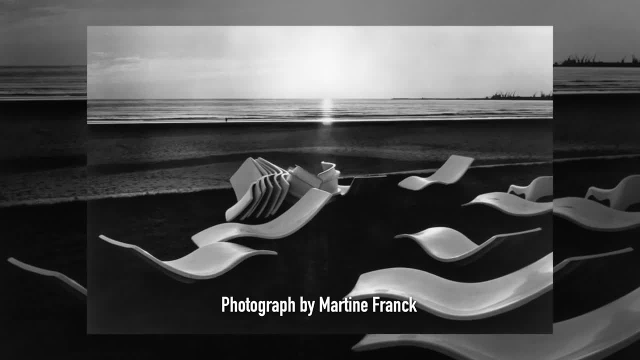 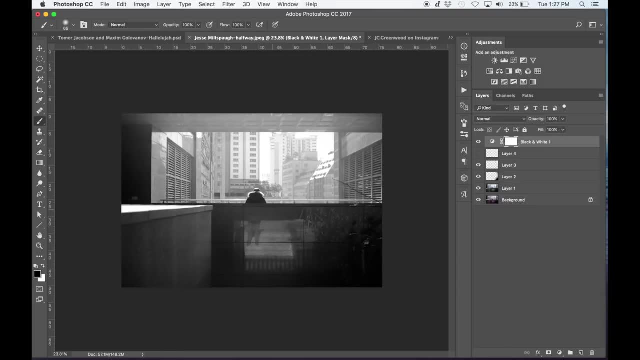 and Martin Franck. they had black and white images that were very surreal. So then we can go in and double check the contrast here. We want our main contrast point right here, the greatest area of contrast right here, So we can manipulate that by increasing the brightness. 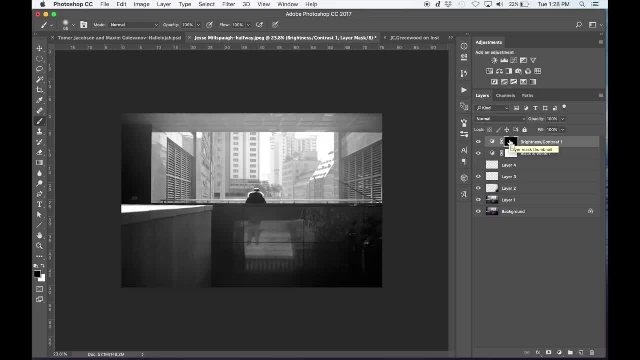 and contrast, pushing Command-I or Control-I to invert that and then brushing in with a white brush To increase just that area and draw attention to where we want people to look first. Then we can look at the other contrast in the image and maybe reduce that. 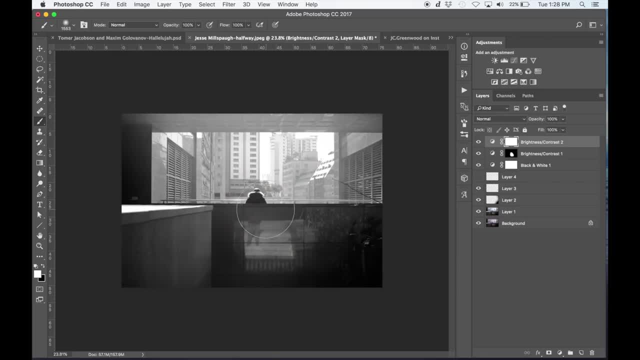 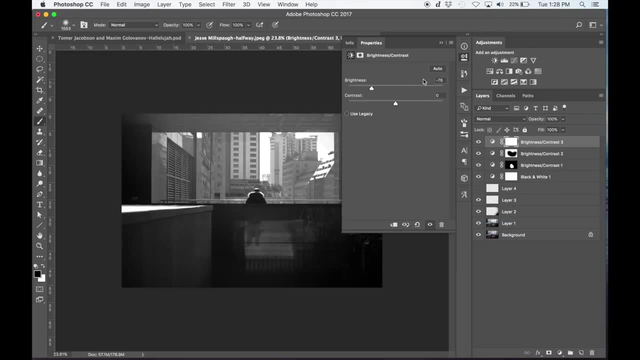 So reduce the contrast and then brush out the areas that we don't want reduced. If you look at some street photographers, you'll see these horrible, horrible vignettes around the edges that just suffocate the whole composition. You don't want high contrast near the edge. 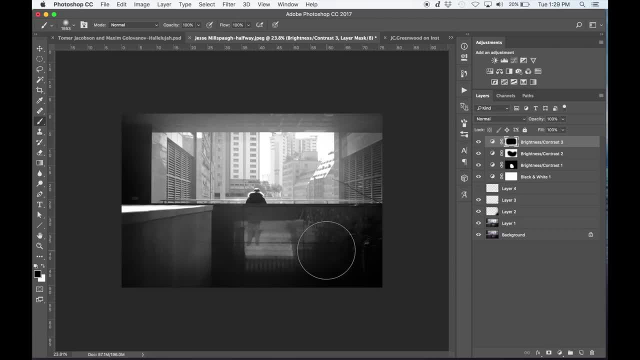 but to do a blanket vignette that just chokes out the whole composition is a bad idea. Usually I'll darken an area and set it to 10%, and usually that's good enough and subtle to slightly draw the eyes in a little bit more. 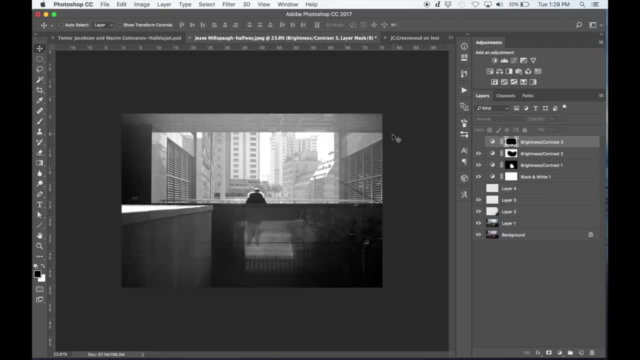 and keep them from the edges. So you're not doing that in this image. I just wanted to point that out. So let's move on to the next one. Cool image. Good job And thanks for submitting that one, Jesse. So this one by JC Greenwood is a pretty cool story. 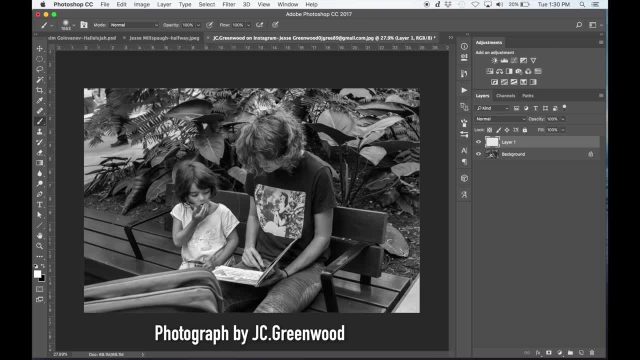 It can be improved, though. The main thing that's messing with the visual clarity is the figure-ground relationship. So if we draw an imaginary line around the subjects, we'll see that we're starting to lose contrast in the head, and we want to keep the head in great contrast. 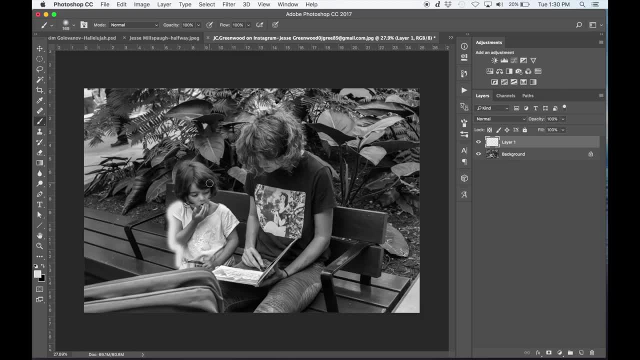 So what's happening is we have different lights and darks in each head, and then the background's capturing light and creating these dark and light shapes too. So it's creating some visual noise in the background, Where we need it, subdued and calm, to help us identify our subjects. 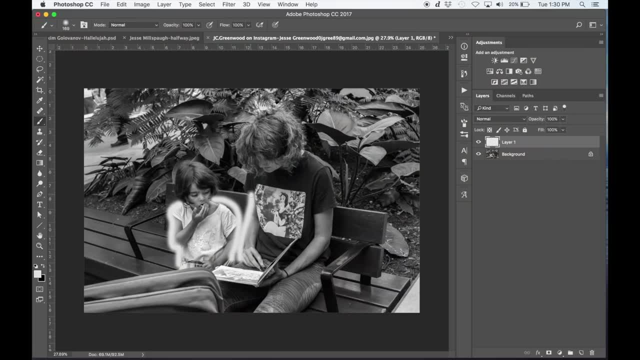 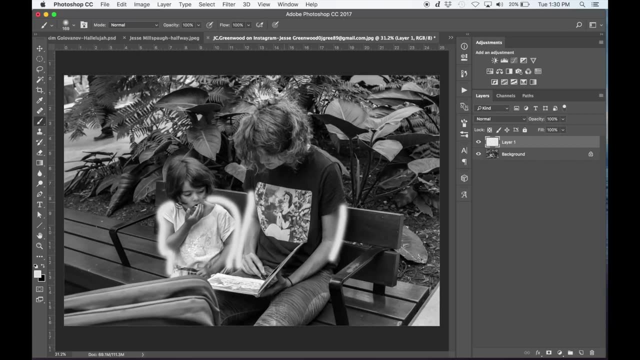 So this is good figure-ground relationship, all except for where the head is Okay. so this is a mom reading to her child that's eating cookies, and then the mom has a Snow White shirt on, which is pretty funny. So it's a funny scene. 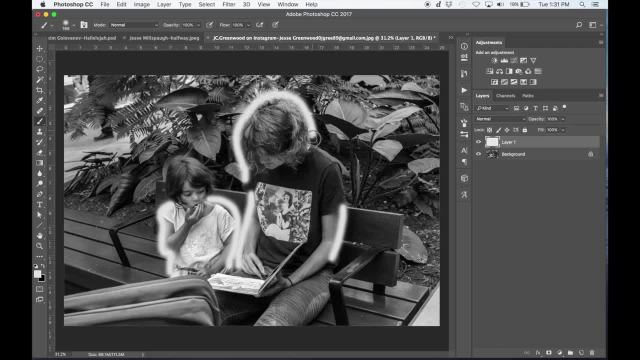 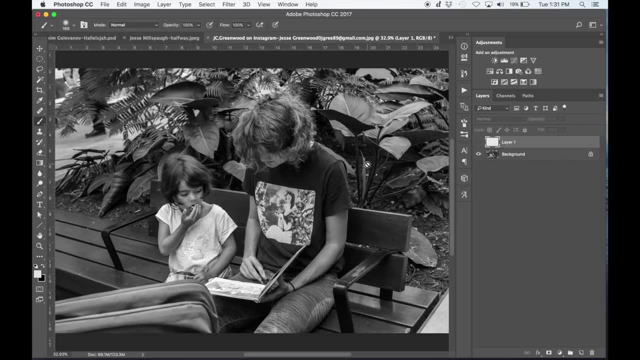 Unfortunately her head is not clearly defined and we have to kind of work to see what's important. I know street photography. it's hard to get close to some people and you don't want to be obtrusive and you know, sometimes it's just. 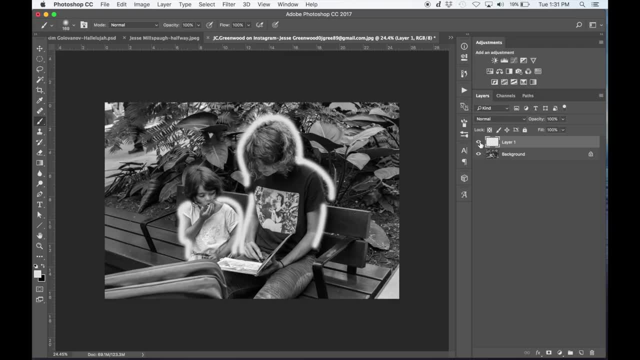 you got to get what you can get. One of the funniest, coolest things about this photo is that she's- this is a gesture- she's shoving a cookie in her mouth while she's looking at the book, So that's hilarious. 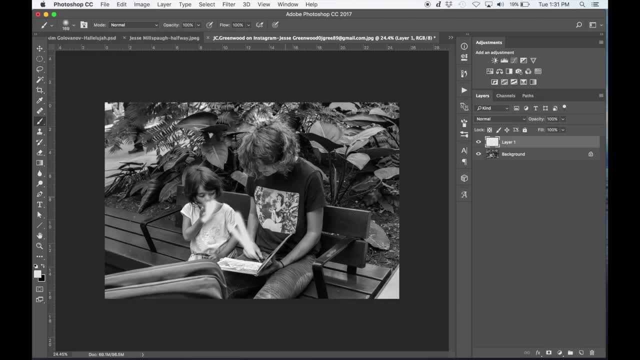 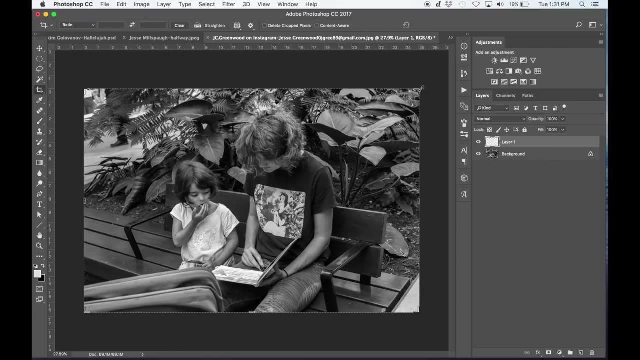 And with the Snow White t-shirt. you know it adds to the story. So if you can't get close, I don't recommend cropping any photos, but maybe you can snip off just a little bit to bring more attention to the story you're trying to tell. 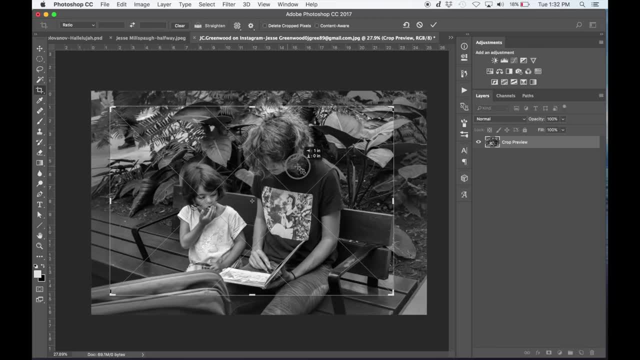 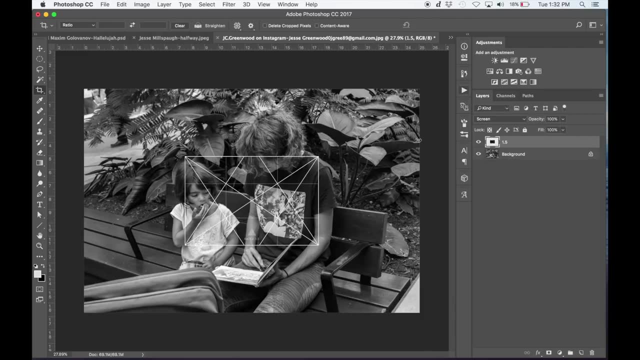 Okay, So I'm going to take this piece in the corner and then adjust it for the balance, And I would typically do that with a grid, So let me put a grid on there. We're going to see if a slight crop would help bring attention. 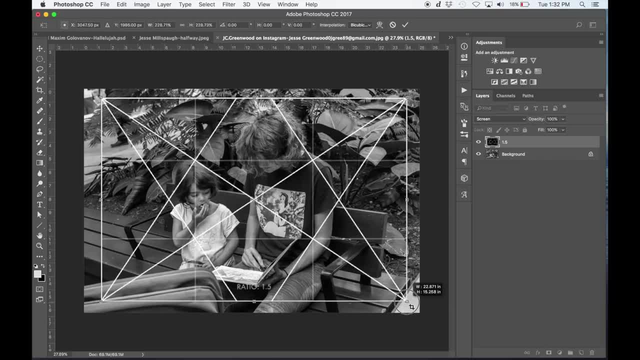 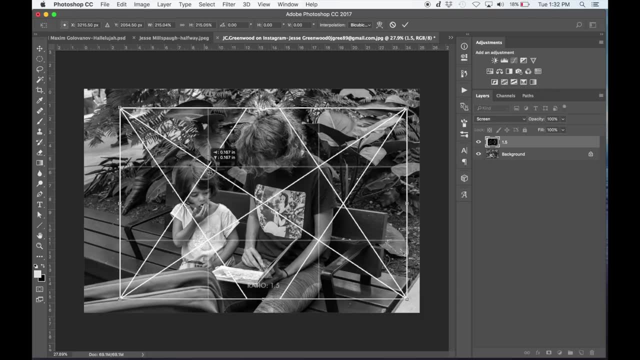 Like I said, don't crop. Try to frame it in camera. I don't recommend cropping to fix an image, but if we can bring the viewer closer to our subject and tell the story in a clear way, like if we were printing this in a book. 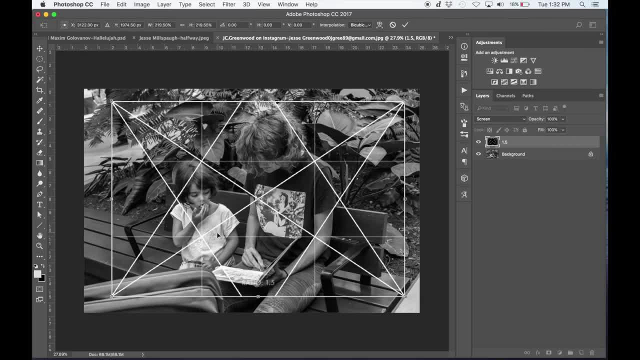 then we might want to do that to have a more successful image, Because you already you have to start with an awesome image. You have a pretty funny image, but cropping is not going to save a crappy image, but maybe it'll save this already pretty funny image. 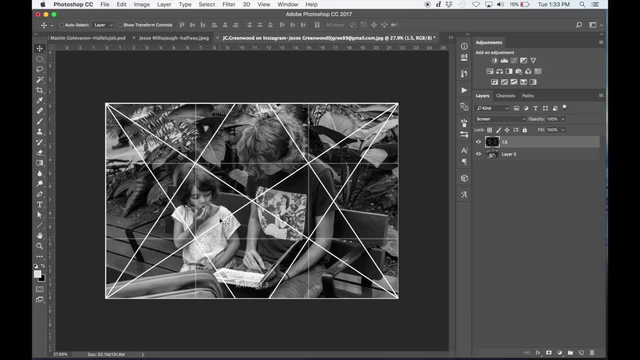 Okay, So I'm just trying to look at the diagonals that you have present in the image and then looking at the balance from left to right. So now, from here, I would go and subdue the edges, for the edge flicker, So I darkened it and then I'm going to lighten this up. 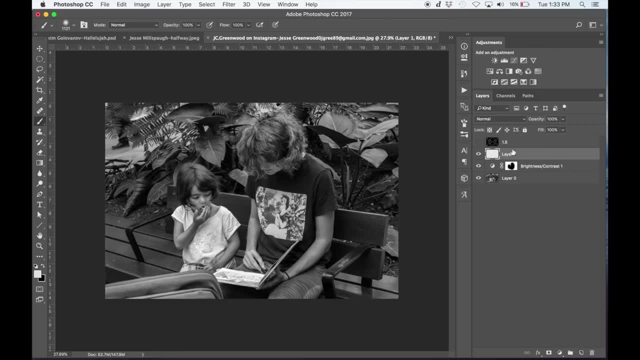 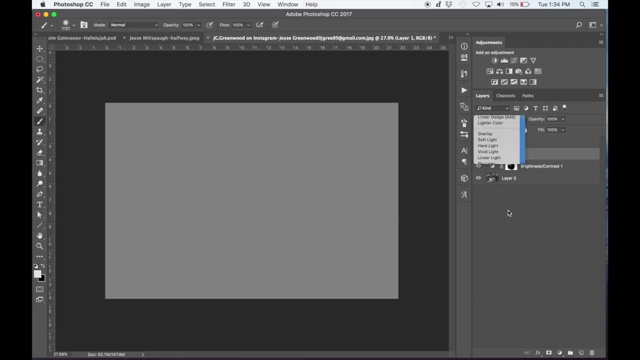 just add contrast where we want to look, And then I'm going to go in, and you can do this a number of ways. I'm going to fill the layer with 50% gray, I'm going to set it to soft light and then I'm going to use my brush tool. 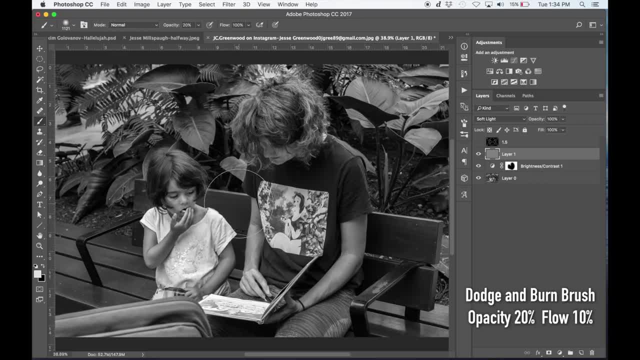 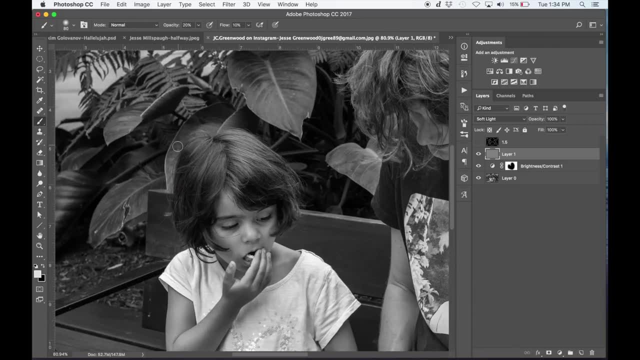 with an opacity of 20% and then hold, shift and push number one and we'll get a flow of 10%, And then I'm going to just go around and improve the figure ground relationship. So this is a little bit of visual tension here. 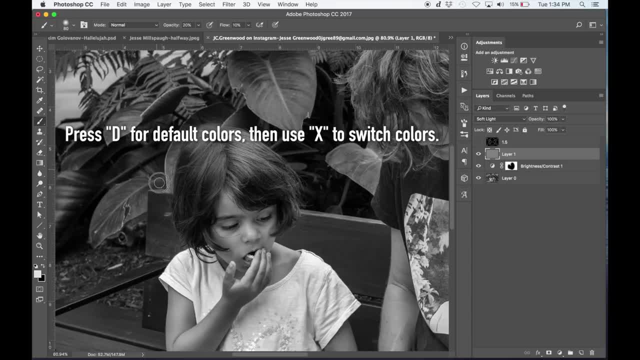 that gutter of contrast. So I want to lighten this, to expand the area, so it's not a small area of contrast, And then maybe I could darken this and darken this even more. Lighten this, darken the leaf in the background, darken this, lighten this. 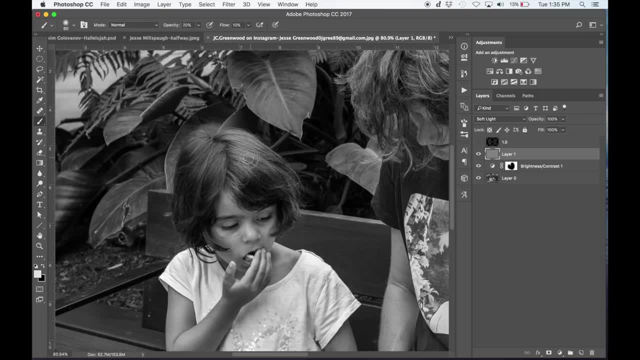 This is real sloppy, but you get the point. Okay, you can manipulate these areas and I switch into black to do the dark spots and then just go around. And what I'm doing? I'm looking for which area is lighter, which area is darker. 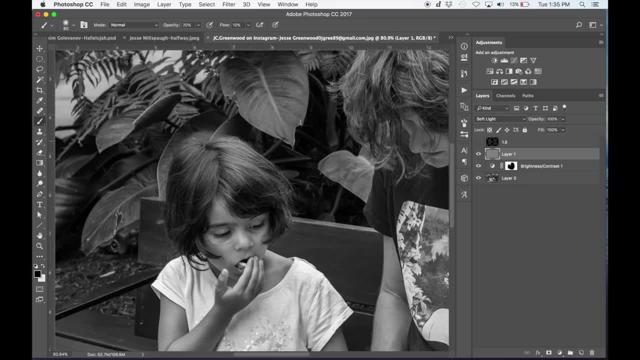 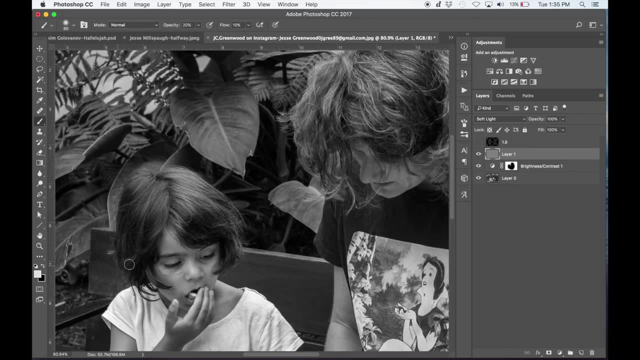 This area is lighter than this. So I'm going to darken this and I'm going to just amplify whatever's already present, Okay, And then just go around this area. So what's lighter? this area or this area, And it's real subtle. 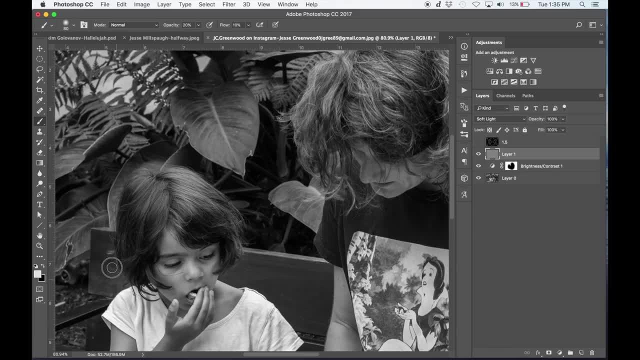 The bench is a little bit lighter, so I'm going to go and lighten that And I'm going to do it in a subtle way and I can adjust the brush size and fan it out a little bit. The flow helps with is just to lay on these darks. 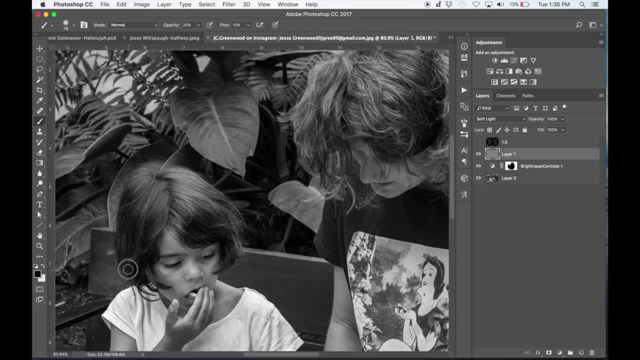 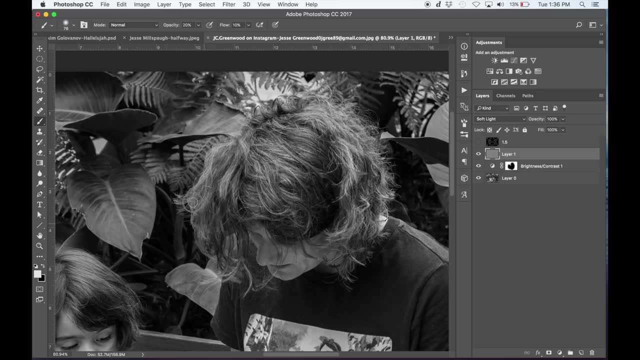 and lights real subtly. So then I'm going to color the hair darker, make that pop a little bit, and then go to this woman's hair and we can see that her hair is lighter than the background. So we're going to just accentuate the light. 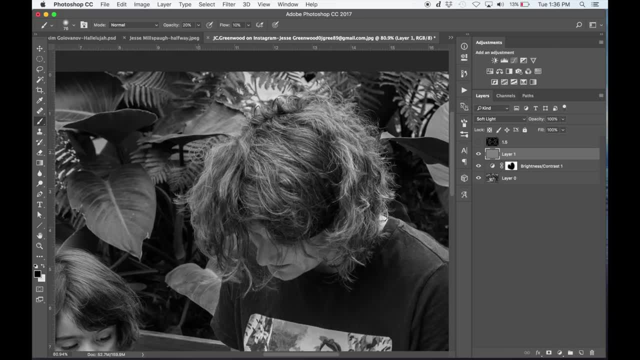 And right here we can see the background's a little bit darker. So we're going to make that darker And this is going to help our figure ground relationship a little bit, make them pop off the background, help our image. So here's darker and that's lighter. 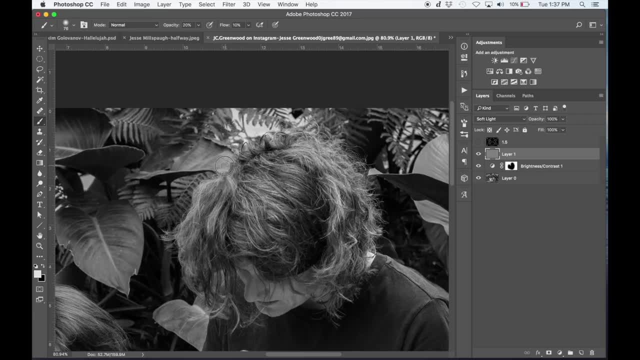 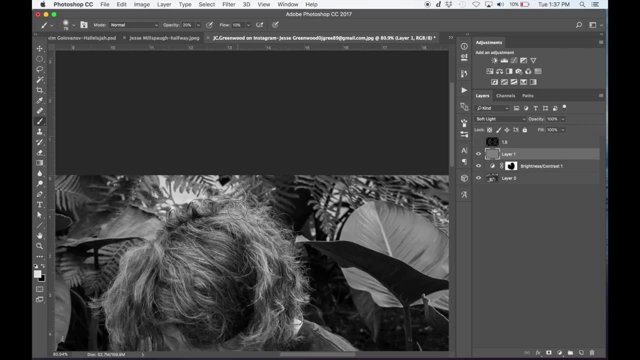 So we want to make this darker, make this lighter. Just work with what is already available and do that value more. That way it looks realistic. Okay, this is lighter, So we're going to go lighter on here, darker on the background. 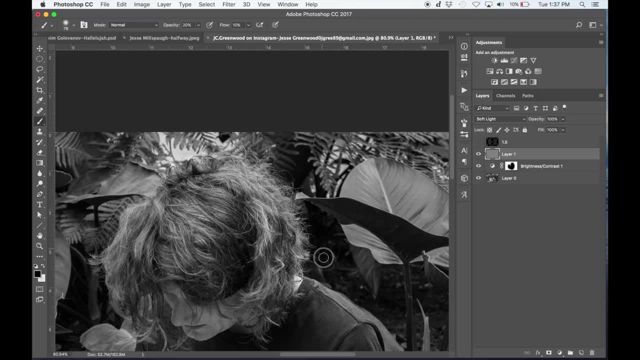 And we want to. we don't want like a big halo effect around our head. So if we start seeing a solid black line like this, we want to just expand it and then fan it out a little bit so it blends in better. So the technique is still hidden. 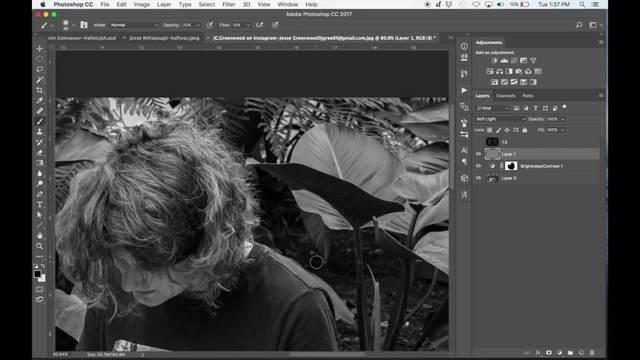 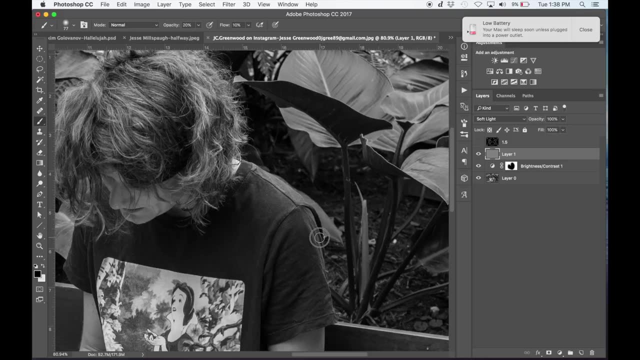 So right here is lighter and the background's darker. We want to go lighter here then and then darker, And this leaf kind of creates some visual tension. So there's nothing we can do about that, unless you wanted to Photoshop it out. but I don't recommend Photoshopping anything. 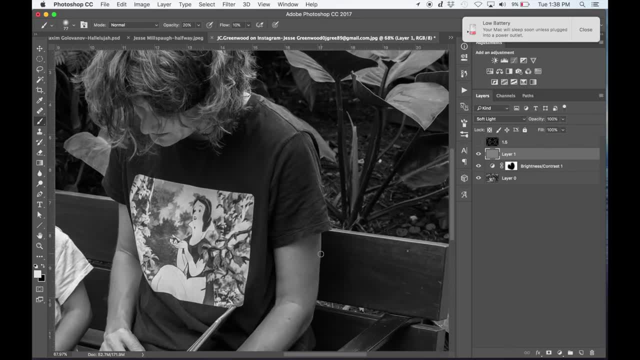 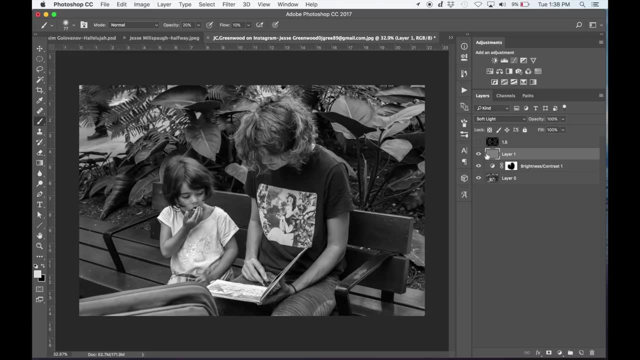 or cropping anything, unless you're really trying to improve it for print work or anything like that. And my battery's about to die, So let's look at: this is after and then this is before, So it pops it out a little bit. 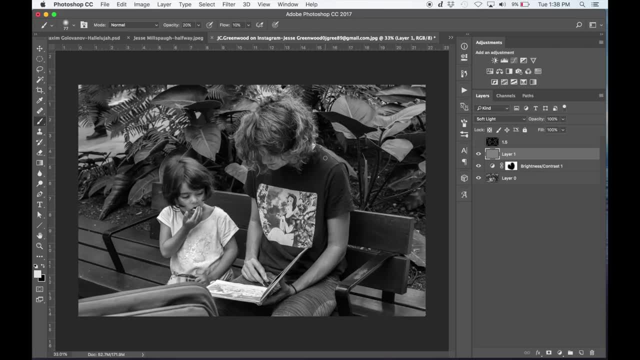 But one thing you want to just look for is just try and capture at least their head in a good figure ground relationship and clarify it for the viewer, if you can. Sometimes I know it's not very possible, but I'm also going to darken this suitcase a little bit. 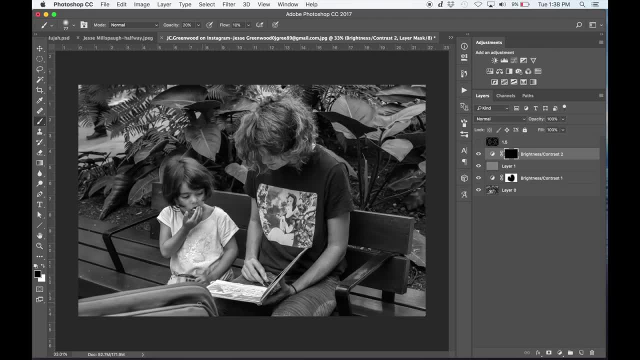 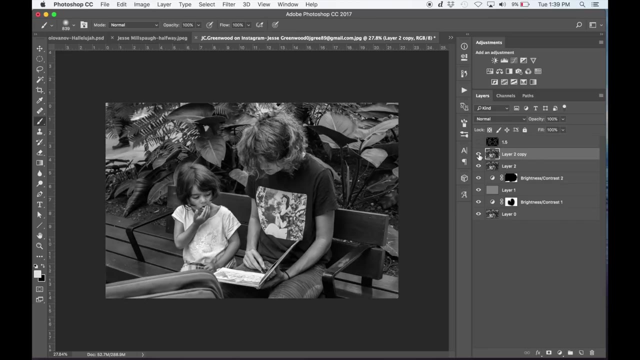 whatever that is, if it's a suitcase or something, And then we should be done, And then up here, maybe over here, and then down here, I'm going to actually merge all those together and then, yeah, our exposure was just a little bit lower. 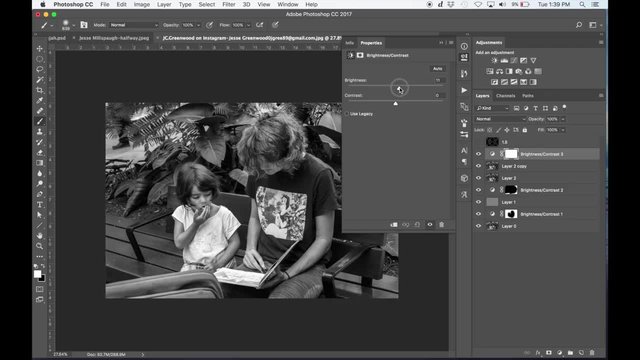 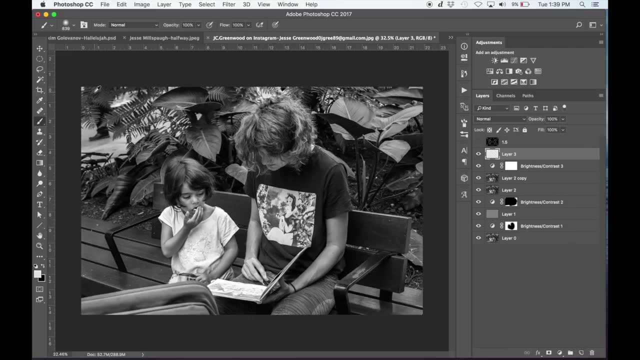 And let's see if we can brighten this up just a little bit more. Okay, so that's okay, so that's finished. And this area up here is bugging me, So I would just subdue that a little bit. 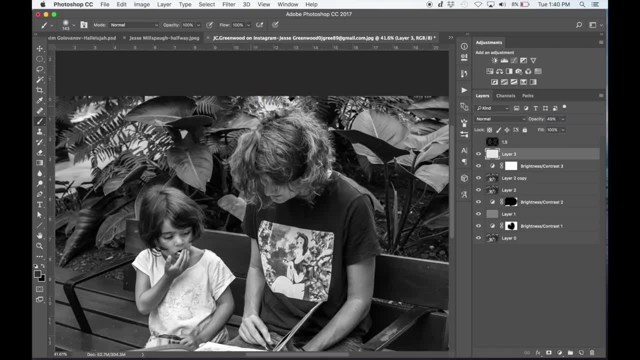 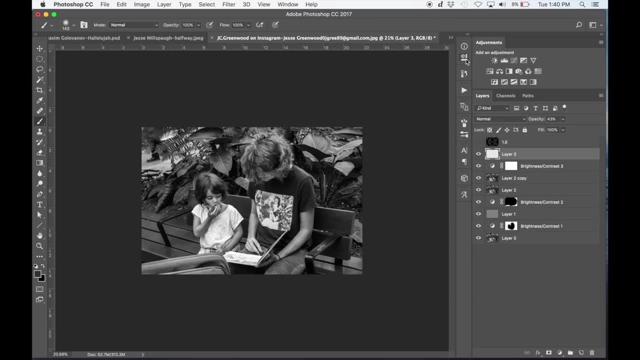 subdue this and then reduce it. There we go, This area. Okay, so that's my edited version: Sloppy, but maybe a little bit clearer on what's going on. Let me look at before and after, and then we'll get out of here. 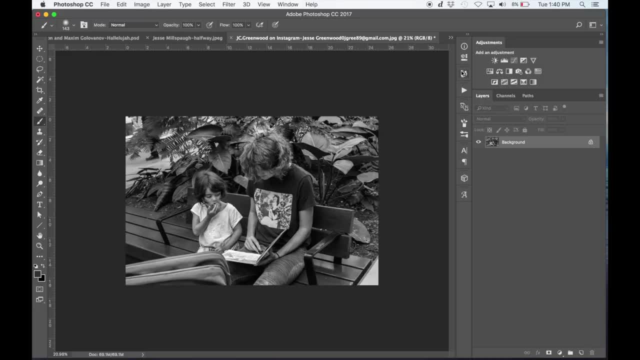 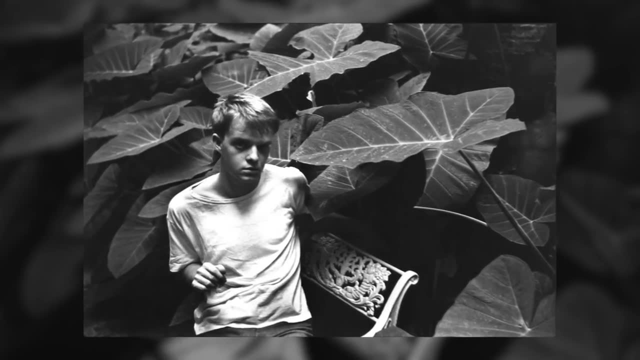 So there's before, after before, after, A little bit clearer, but that background is really hard to work with. That's just to give you some ideas. I love that picture, Just needs some fine tuning to emphasize the story that's being told.